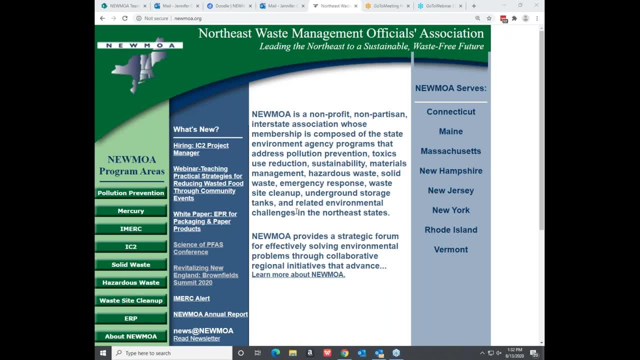 And I will just show you where they are, And also there's a lot of other information that you might be interested in. So you would go to the homepage, which is just NMOWAorg. pick Wayside Cleanup here on the left side. You'll also note that NMOWA's website is very 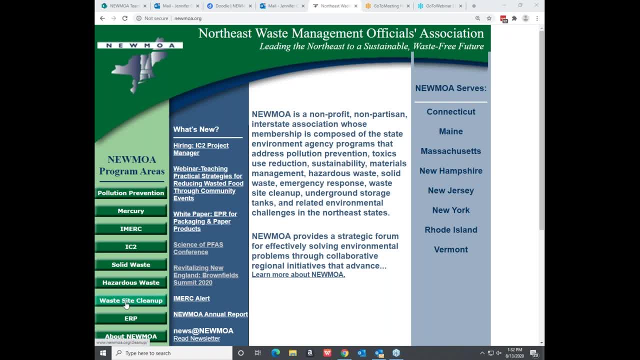 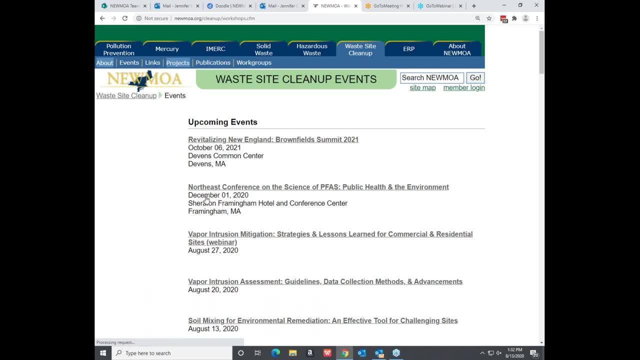 ancient. I think it was designed back in the 90s, But it still works. So you pick Wayside Cleanup, you get here, you pick events, And then we have a lot of other things. So we'll show you more of what possible events there are going to be happening in other jeitoes. 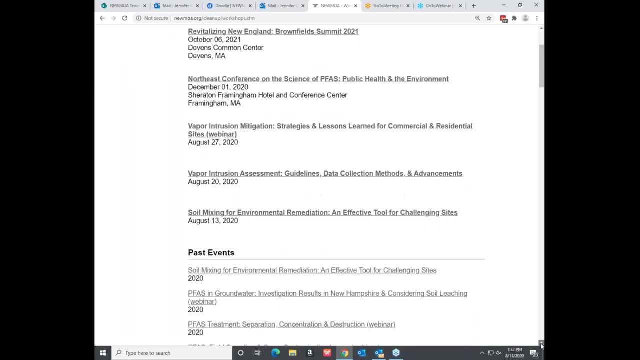 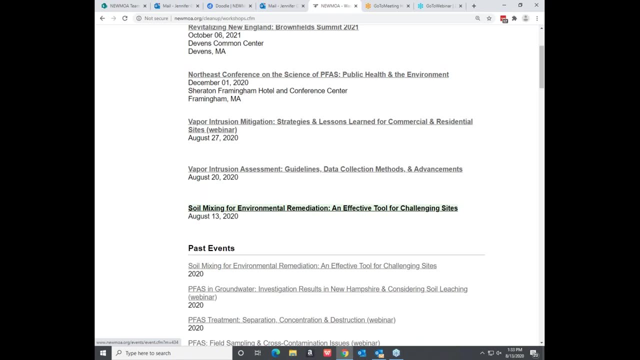 and situations along the way aboutadeshorg, And then we have some future upcoming events. We have 2 more webinars that are currently you can register for. They are about vapor intrusion, if you're interested. The next week will be a focus on assessment and the following week on mitigation, But today 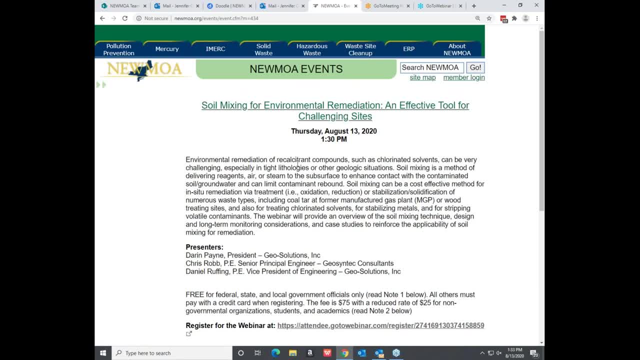 we're here for 來, So this will obviously become a past event- Oops, it's already duplicated- And then the presentation will be posted. I'll rework the webpage for that as well, so you'll find the the website for the webinar to put in the past tense and post the presentations here. but as you 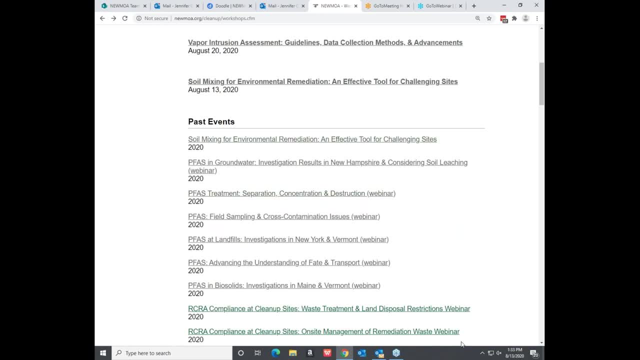 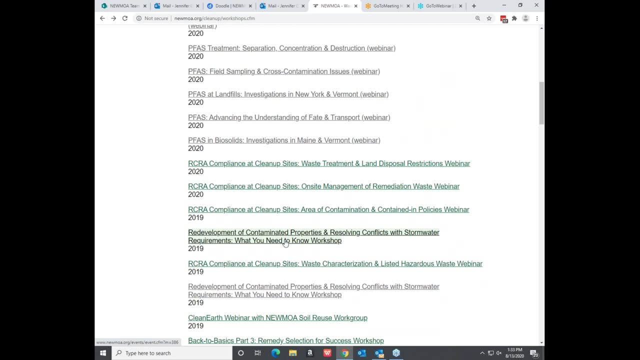 can see, Nemo has done a lot of other webinars and we've also hosted in-person workshops back when we could do that. so here was a workshop and all the presentations from all of these different events are posted for your future reference. so, on the webinar today, we've got people from all. 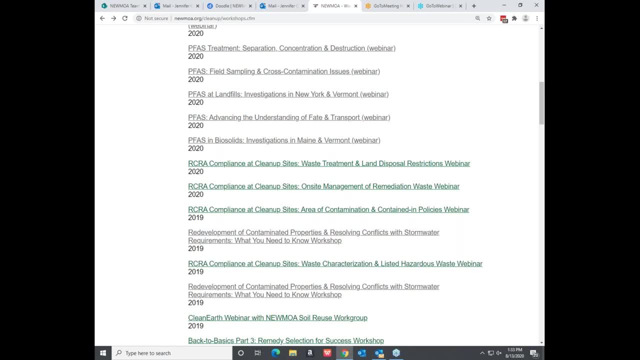 across the country. so thank you for joining us and because of the large number of people attending, we will not be able to ask questions verbally. you can type them in at any point. so in your control panel for go to webinar there should be a box or a section for questions and you can enter. 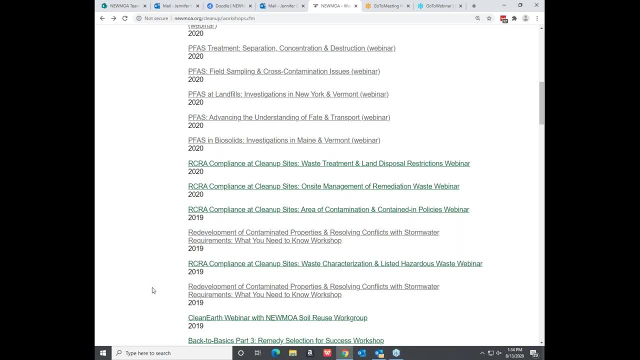 questions that you have at any point I think we'll have. the presenters will take breaks during their presentation and ask if there's any questions and if there are, I will ask them of them. so type your questions in at any point. so I think that is it for logistics. like I said, the presentations will be posted afterwards here on the Nemoa. 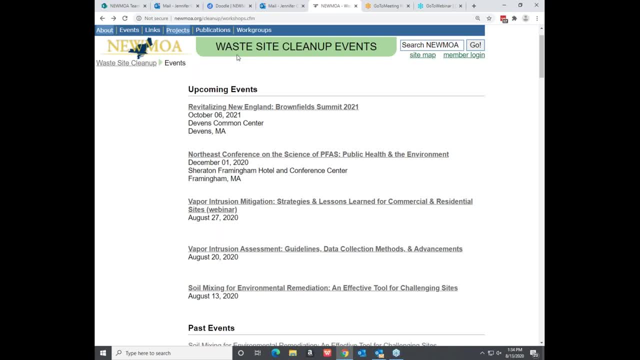 web site. so with that I'm going to introduce our presenters. they're going to kind of go one after one and then I'm going to give them a little bit of time to answer some of the questions each other. so I'm just going to introduce all three of them now, so this might take a minute. 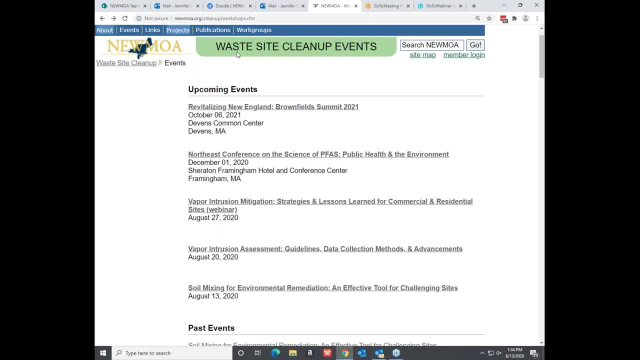 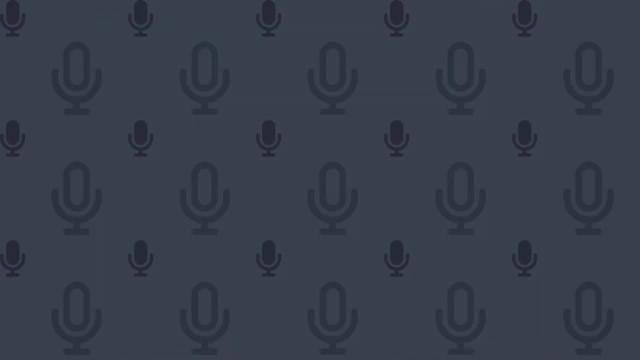 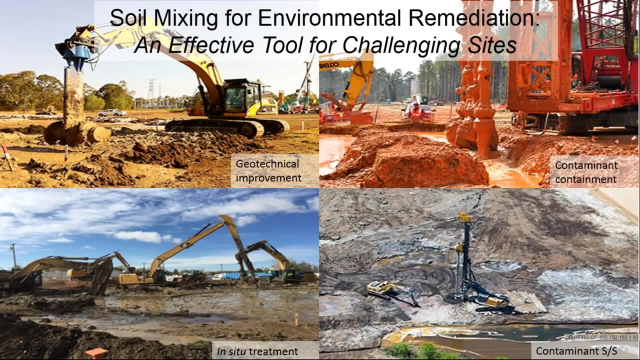 and then I'll turn it over to them. so actually I'm going to turn the slide over to them right now, but let me introduce them first before they get going. so we've got. first up will be Daniel Ruffing. he is a vice president at GeoSolutions, where he oversees his 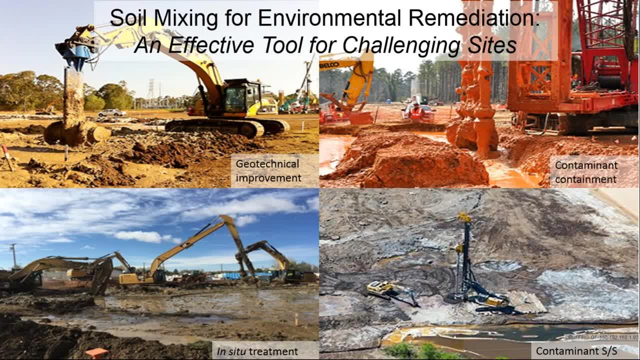 quality control, marketing, estimating and business development functions. Dan has over 10 years of experience in geo environmental construction, including management and oversight of projects involving numerous specialty construction techniques, such as slurry trenching and soil mixing, which we're going to hear about today, and he's authored several numerous technical publications on those topics. 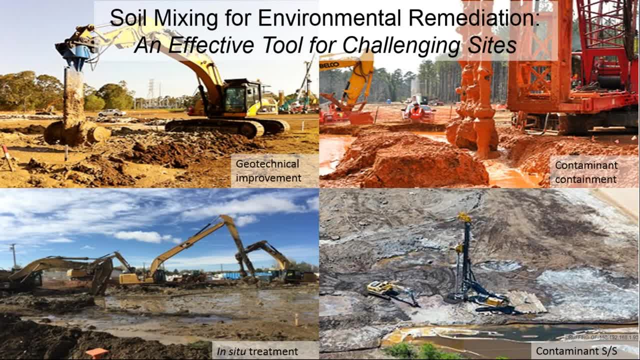 He's based in GeoSolutions headquarters office, which is in Pittsburgh, Pennsylvania, and supports projects throughout the US, as well as in Canada and some other international markets. Dan has his bachelor's and master's degrees in civil and environmental engineering from Bucknell University and he's also a registered professional engineer in Pennsylvania. 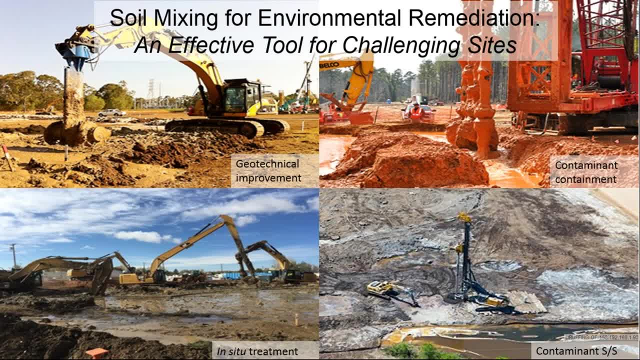 Following Dan will be Chris Robb. he is a senior principal engineer at GeoSyntec in their Wisconsin office. He has over 24 years of experience in environmental consulting, design and field engineering, construction management, quality control and project management of solid and hazardous waste remediation projects throughout. 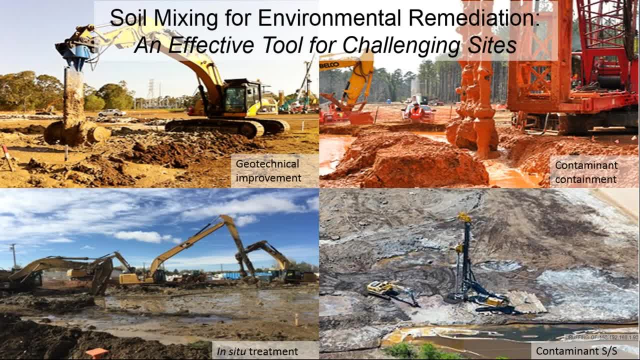 the United States, Australia, Canada and Europe. Mr Robb is a recognized leader in the design and application of in-situ solidification and stabilization technology for Superfund, manufactured gas plant and sediment sites and has authored numerous peer-reviewed technical public presentations and papers, and he's presented at various conferences and industry groups. 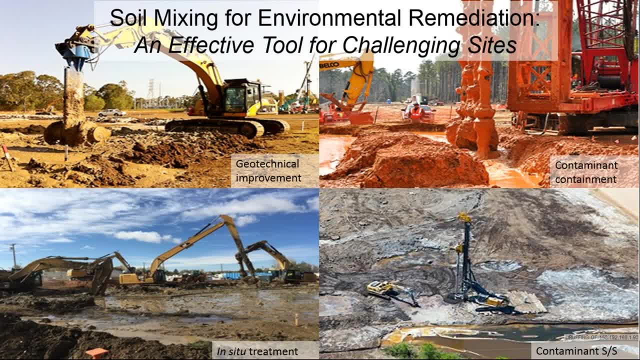 He was also a contributor to the 2011 ITRC, which is the Interstate Technology and Regulatory Council- another organization of states and folks- their guidance document, which was on development of performance specifications for solidification stabilization. Chris has his BS bachelor of science in civil engineering from the University of Wisconsin in Milwaukee. 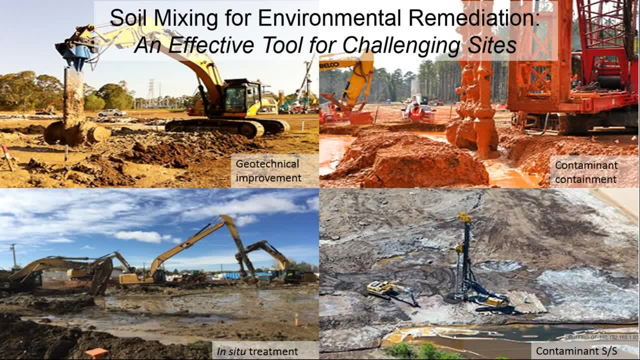 And then finally, we'll have, we'll hear from Darren Payne. he is responsible for oversight of operations at GeoSolutions, including key decisions related to safety, quality control operations and the allocation of company resources. Darren has over 20 years of diverse experience in overseeing all stages of project development for geotechnical and 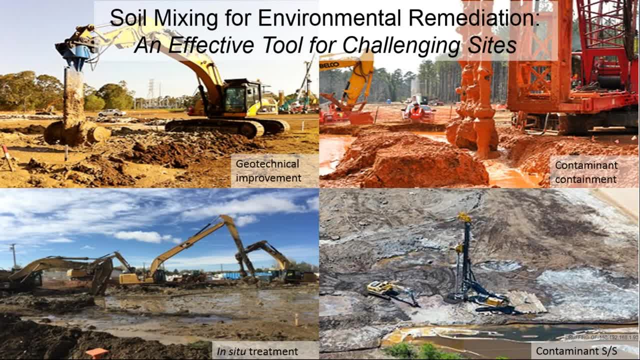 environmental clients. Darren is experienced in various sites for mediation and construction techniques, including soil mixing, in-situ solidification, stabilization, biopolymer and permeable reactive barriers, slurry walls, slurry cut-off walls, engineering, engineered shoring and dewatering, demolition and earthwork. So Dan Darren- excuse me- is based in the St Petersburg, Florida office of 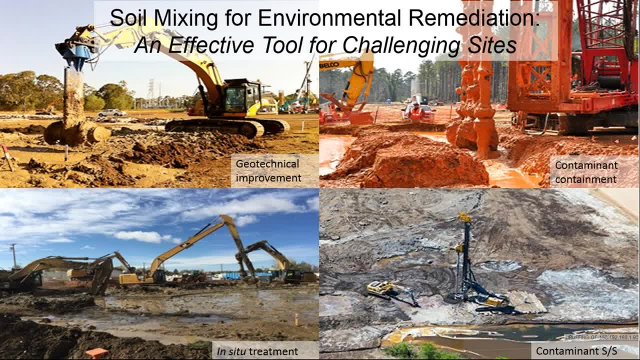 GeoSolutions, and he graduated from the University of Massachusetts, Amherst with a degree in environmental science. So with that I'm going to turn it over to Dan. Take it away, Okay, thanks, Jennifer, and thanks everybody for calling in today. The talk that we're going to do is going to 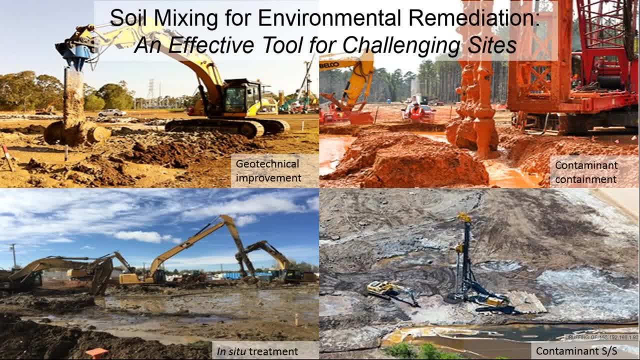 be about in-situ soil mixing, specifically focusing on the application of soil mixing to environmental mediation sites. The four photos that you're looking at right now- the bottom two would be applicable to today's presentation. I included the other two to just highlight quickly some other applications of. 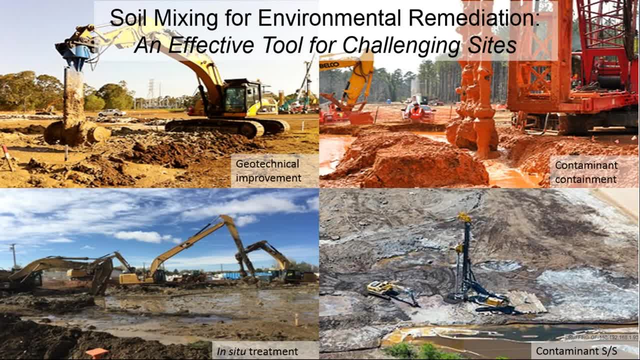 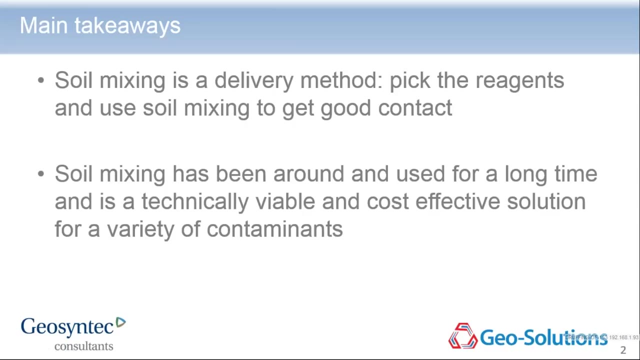 soil mixing, which include geotechnical improvement, which might include for liquefaction control, bearing capacity improvement or slope stability improvement, and then also the installation of containment features on the right there. So we're going to start with the soil mixing. All right, so we've got a couple of takeaways that I would like people to get from this overall. 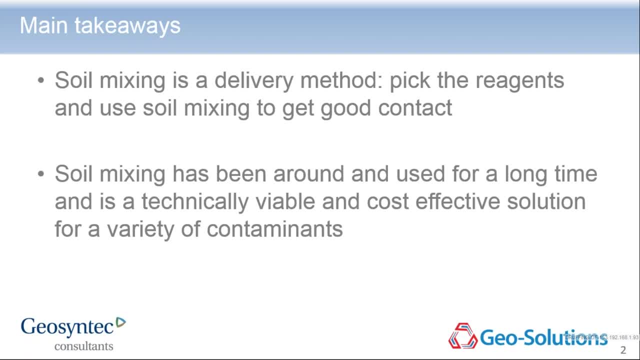 presentation. It's one that soil mixing is the delivery method, and it's a delivery method that's somewhat independent from the lithology that you're delivering the reagents into. It can be performed under the groundwater table, almost independent of soil type, Once a good reagent combination is developed, whether that's an oxidant, a reducing agent, 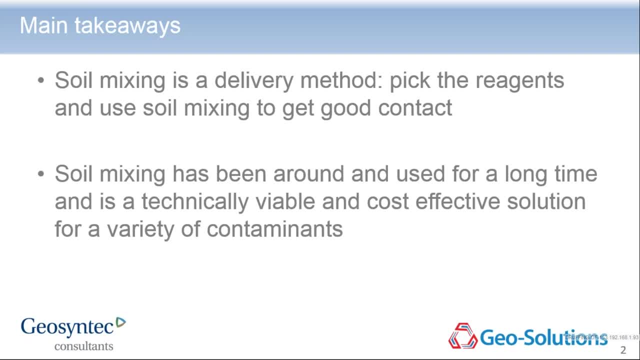 a solidification stabilization agent. the soil mixing is just a way to get it into the ground and get good contact with the soils and contaminants. The other thing I'd like you to take away is that this has been around a while and it's a technically viable and cost-effective solution for a variety of contaminants that's. 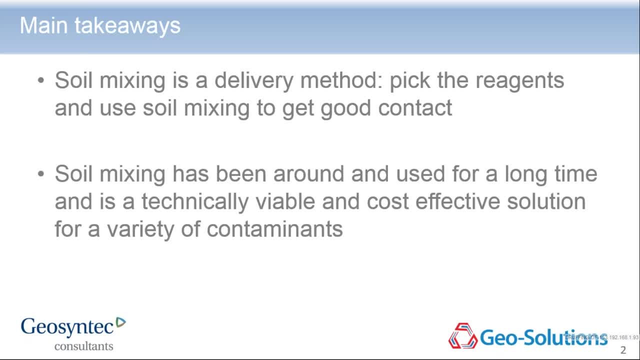 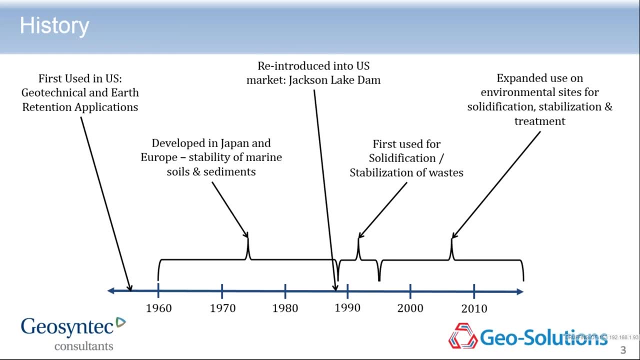 accepted by a number of regulatory bodies and in some cases is the preferred technique. So the concept of soil mixing is relatively simple, You know. basically it's a method of adding reagents to soil. Sometimes it's just a mixing of soils with soils. You know, concrete could be considered a soil mixing technique in that. 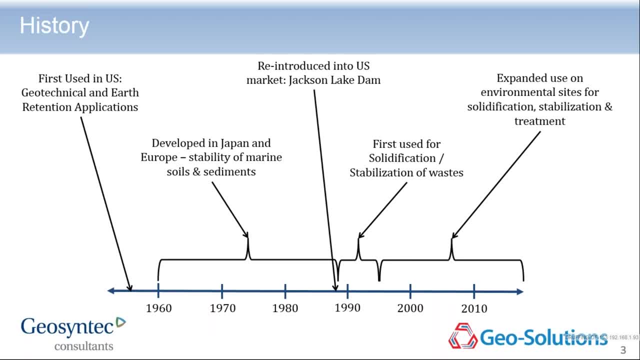 it's Portland cement mixed with a variety of different aggregates and specific proportions. Bricks would be another old application of soil mixing, where you're mixing clay with water. But really our focus today is the in-situ application, So any soil mixing that is performed underground. 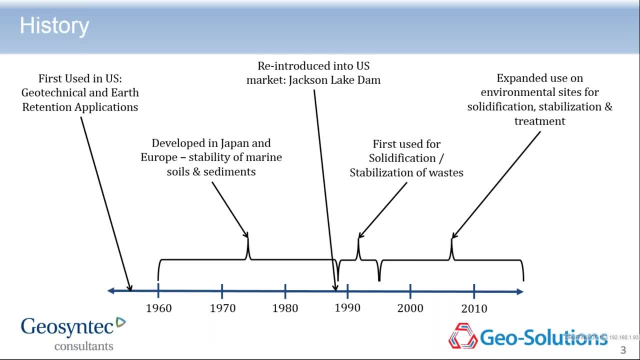 and specifically for environmental remediation objectives. The overall general history of soil mixing is that a patent was filed in Ohio back in the 1950s which was for geotechnical and earth retention applications. A lot of the development of the technique and the improvement of equipment. 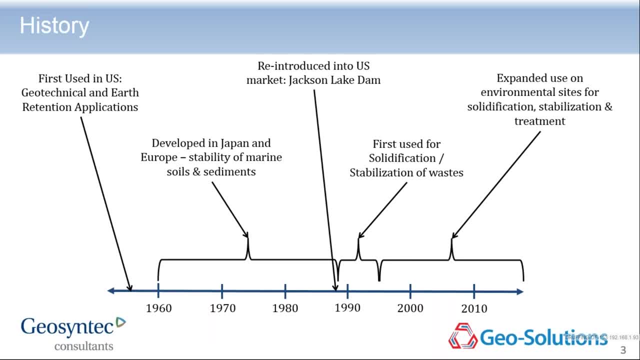 which drives the application of the soil mixing technique to different sites and more challenging sites Was in Japan and Europe and specifically the focus there was for improving the stability of marine soils and sediments through the inclusion of lime and Portland cement. In 1987, through a JV with a Japanese company, the technique was brought back into the United. 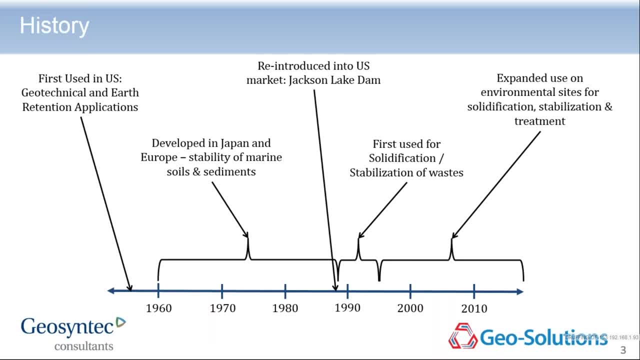 States for a large seismic retrofit of the Jackson Lake Dam out in Wyoming. And about that same time you started to see the application of the technique for the solidification and stabilization of waste. And then you started to see the application of the technique for the solidification and stabilization of waste. 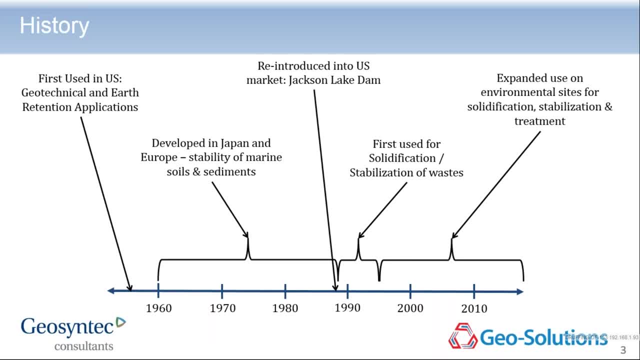 And then you started to see the application of the technique for the solidification and stabilization of waste. And then, more recently, the reagent combinations have gotten more complicated. So we're doing a lot of oxidation reduction, enhanced biodegradation, steam stripping. 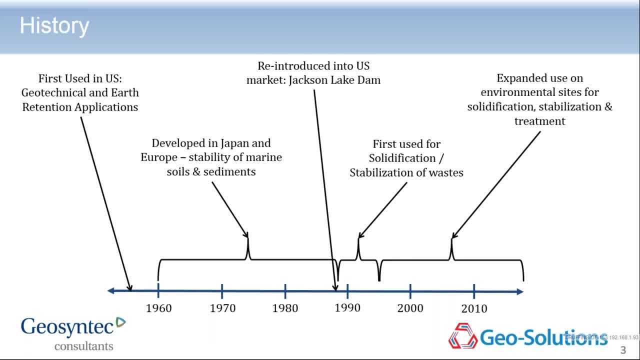 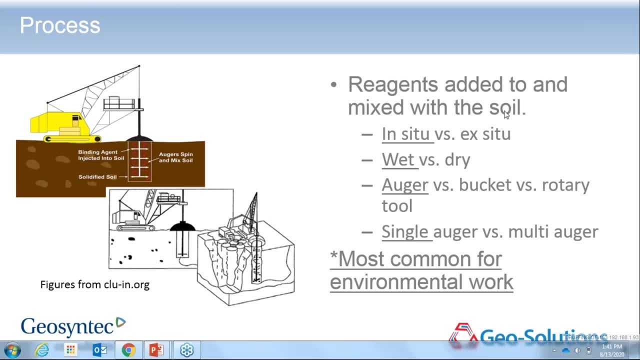 So the technique is the same, the equipment is relatively the same, but the reagents have changed over time. The process can vary from in situ to ex situ. Our focus today is the in situ component of it. You can add the reagents. 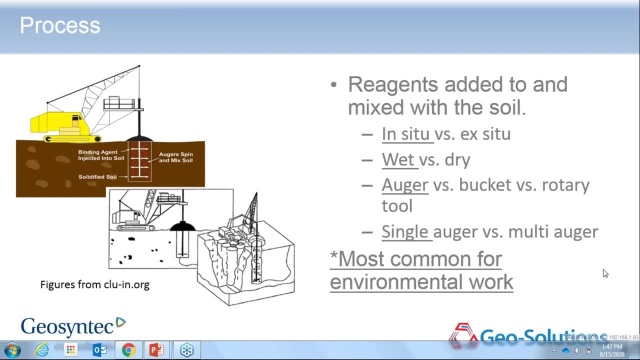 In a wet form or a dry form. Most of the environmental remediations are performed with wet grouts. There are a variety of equipment techniques which we'll talk about later, which include excavator, bucket, mixing rotary tools, which are large rototillers, essentially. 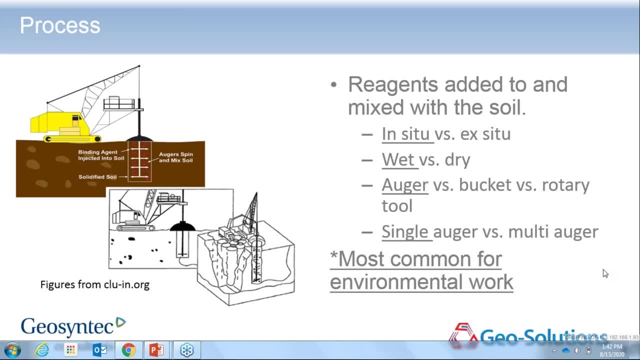 and augers. And then the augers can be in a single auger configuration or a multi-auger configuration, But basically the overall purpose is to get the reagents into the soil and to mix them into the soil. So we're going to talk a little bit more about that in just a few minutes. 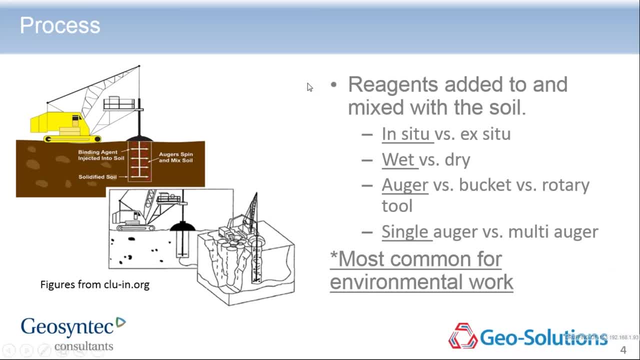 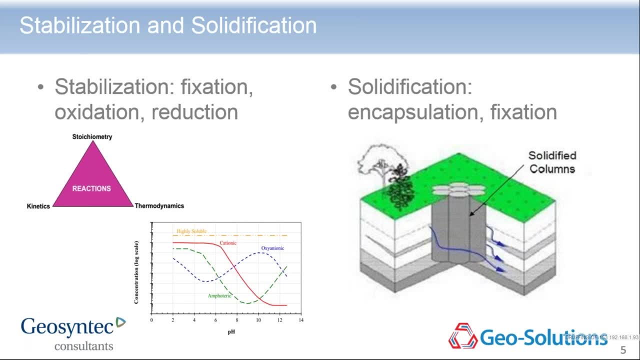 But before we do that, I just want to make sure that everybody understands this a little well. So the EPA defines stabilization and solidification as separate definitions. A lot of times people in the industry use these terms synonymously. That's sometimes correct, because a lot of times if you're trying to target a solidification approach, there's also some stabilization that's taking place. 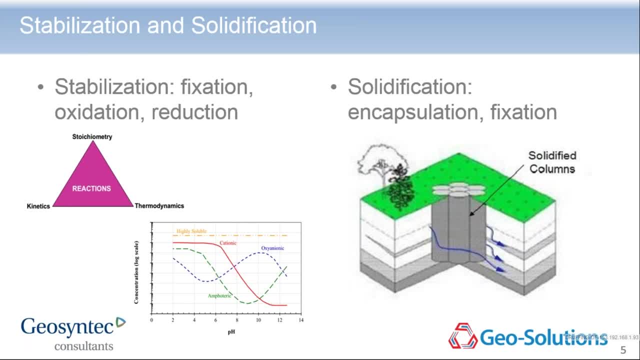 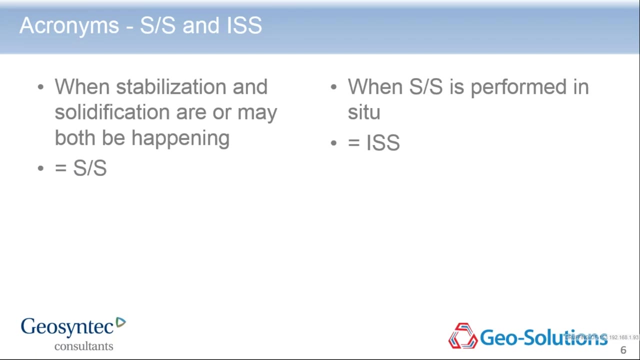 The general distinction between the two is that stabilization causes a chemical change, whereas solidification is more of a physical change, like encapsulation or fixation. So some common acronyms in the soil mixing industry are the SS, that's, stabilization and solidification. 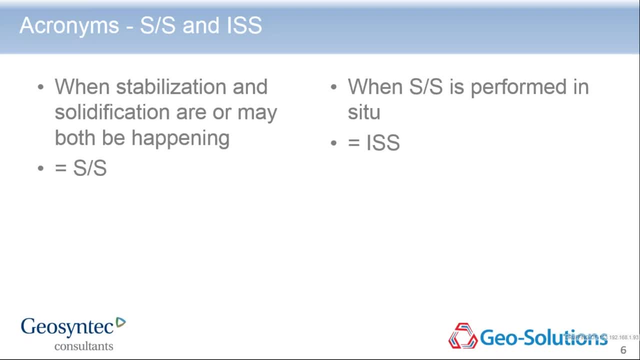 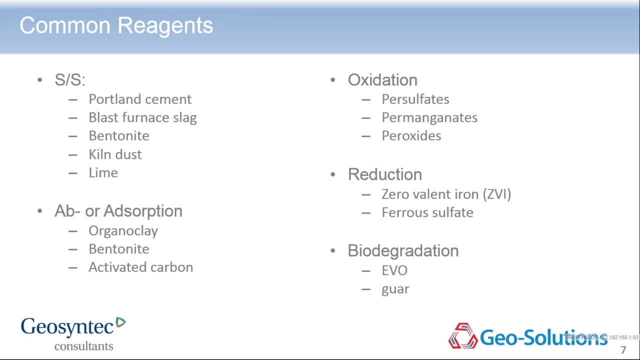 So that's for any technique where you're not necessarily distinguishing between one or the other and it's possible that both are taking place, And then ISS is just in situ: solidification and stabilization, So common reagents that are used for each of these techniques. 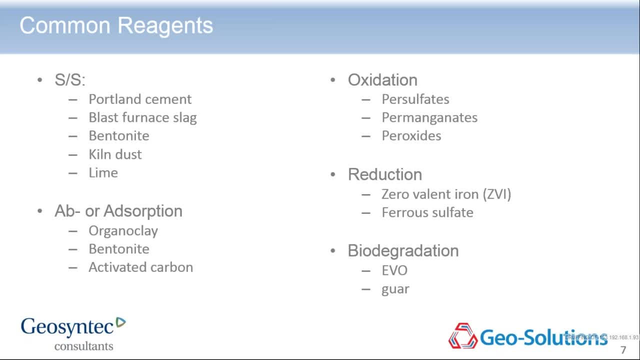 Portland cements by far the largest reagent, but blast furnace slag is probably a close second and has gained a lot of steam over the last few decades, mostly related to the fact that the slag improves the performance and a lot of times it provides a cost benefit. 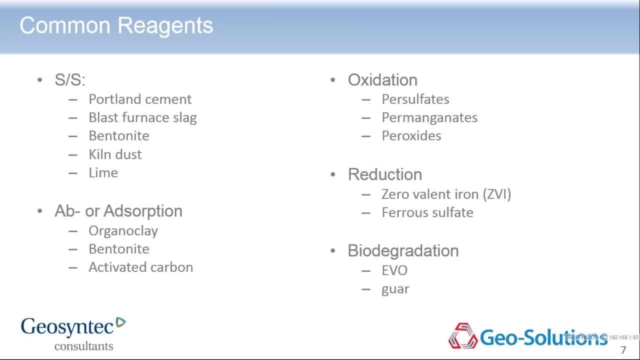 Then there's other reagents Like bentonite, various kiln dusts and lime that can be added for specific purposes. You can add reagents that adsorb or absorb contaminants. Those might include organoclay- Bentonite has some of those characteristics- or activated carbon. 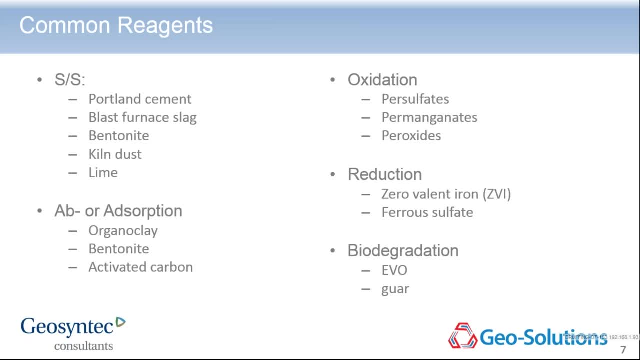 If you're targeting an oxidation reaction, you get into the persulfates, the permanganates, the peroxides and various other oxidants And then reduction would be zero. valine, iron, ferrous sulfate, and biodegradation is often performed as a supplement to a reduction reaction. 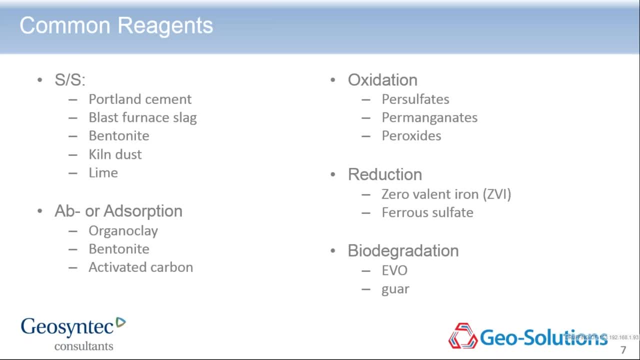 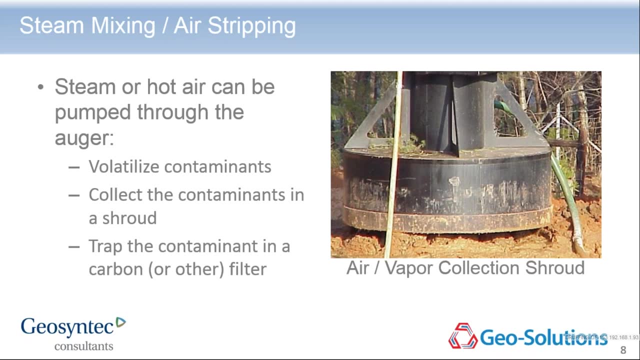 But a lot of times the biodegradation component is either through the addition of air or some sort of carbon source like EVO or Guar. So another application of soil mixing that isn't really a delivery of reagents necessarily is the addition of steam or hot air into the soil to volatilize the container. 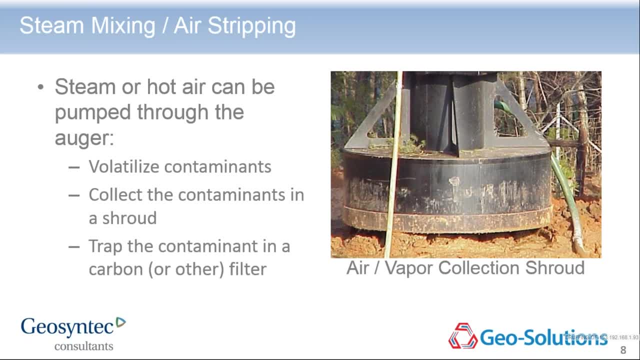 contaminants or strip them from the soil and groundwater, and then those contaminants are carried up with the air or steam to the surface. They're collected in a shroud and then all of the air in that shroud is pulled out and run through a carbon or other filter. 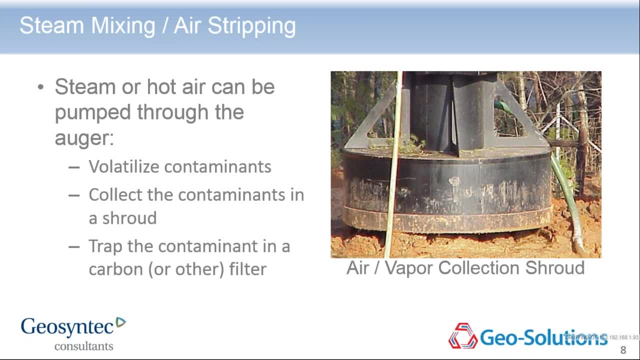 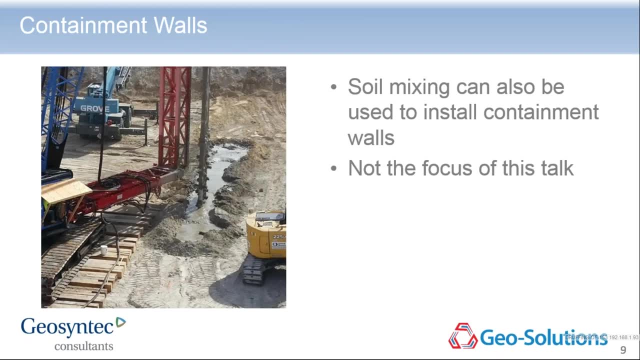 to trap the contaminants in that carbon base, which is then disposed of off-site. So I touched on it briefly in the beginning, but this isn't the focus of this talk. but I wanted to highlight the fact that soil mixing is not only a viable technique for 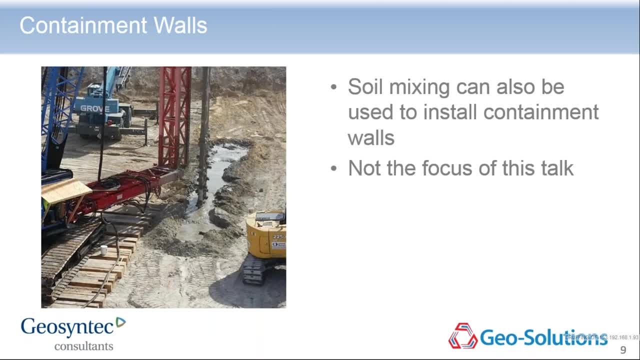 environmental remediation through direct application of the reagents, but it has application for the installation of cutoff walls, specifically on sites where access might be limited for other techniques or the handling of the materials at the surface would be dangerous for the workers and the public, and soil mixing can be used to deliver the reagents and install. 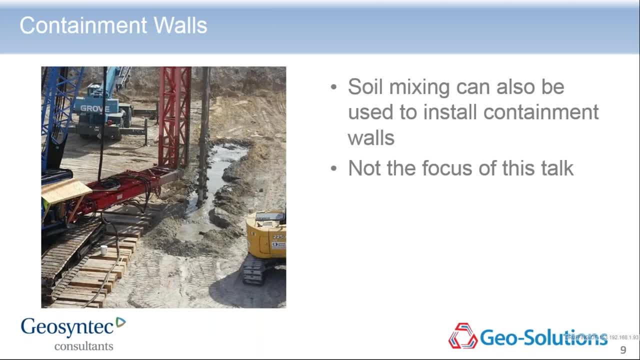 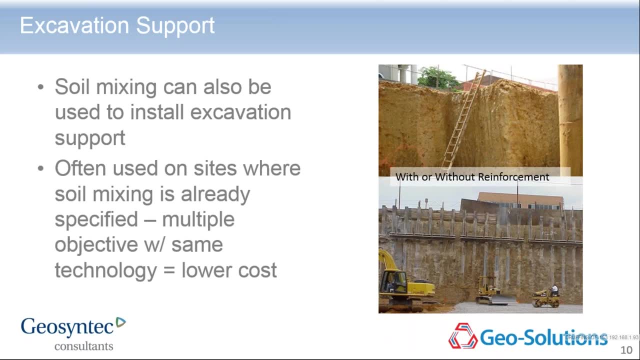 the cutoff wall without significant impact from the contaminated material. The other related application is the use of soil mixing to install excavation support systems. This is often a common application of soil mixing on sites where soil mixing is already being used to perform some other site function and the excavation support is a secondary feature. 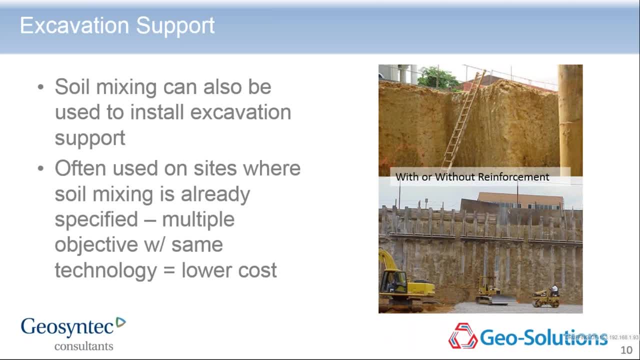 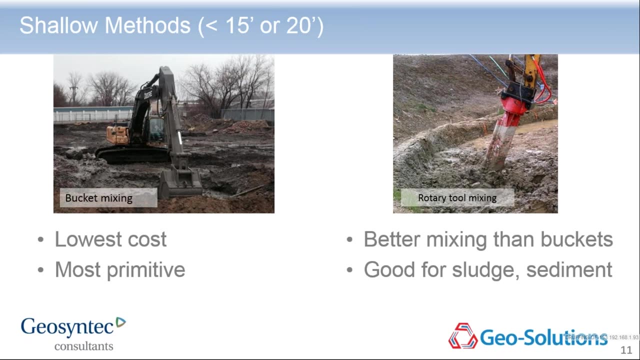 and it saves the project time and money by not having to mobilize a second contractor or having to do a different technique. The soil mixing is just used to accomplish multiple site objectives. Going through some of the methods of soil mixing, bucket mixing is the most primitive method. 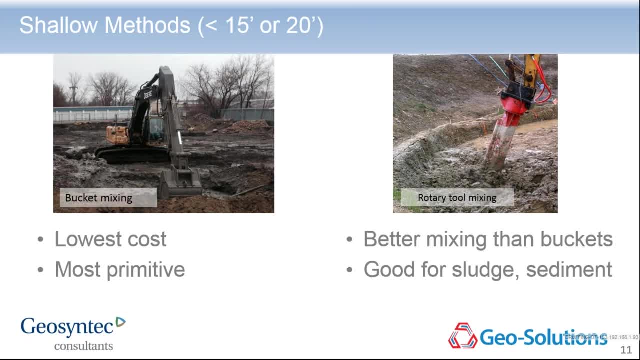 and this is essentially just using an excavator to mix the reagent into the soils, wet or dry. It's the lowest cost and it's applicable for depths up to 10 or 15 feet or so, maybe a little bit deeper in certain conditions. Rotary tools can be used to. 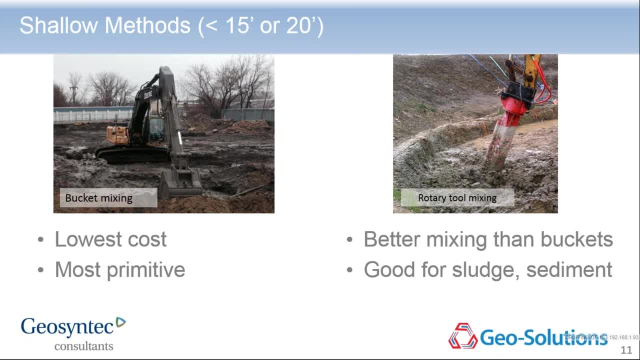 improve the bucket mixing. They impart additional mixing energy. In some cases they can be used to extend the bucket mixing a little bit deeper, but these are essentially large rototillers. Most of the commercially available units are not suitable for mixing virgin soils, so they're really for additional mixing after the bucket has already been used. 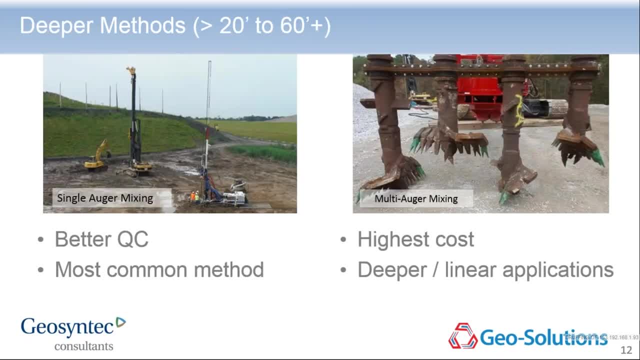 to loosen the soils. As you get deeper than 20 feet or so, get into auger mixing. single auger mixing bucket mixing is the most common technique and this is with large-diameter augers up to 10- or 12-foot diameter. 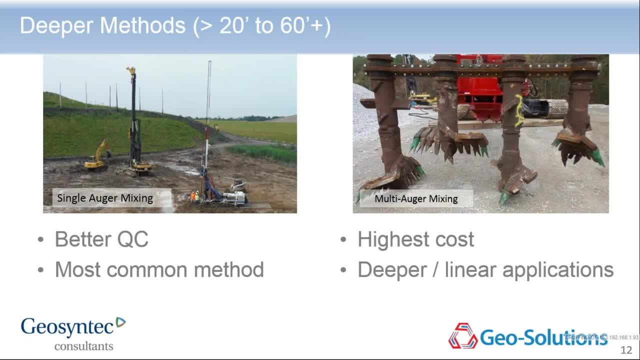 Much better QC than you would get from bucket mixing, but at a slightly higher cost. And then multi-auger mixing can be used for really deep applications. It's also efficient for the installation of linear elements, like the containment walls that we were just talking about, but it comes at a higher cost. 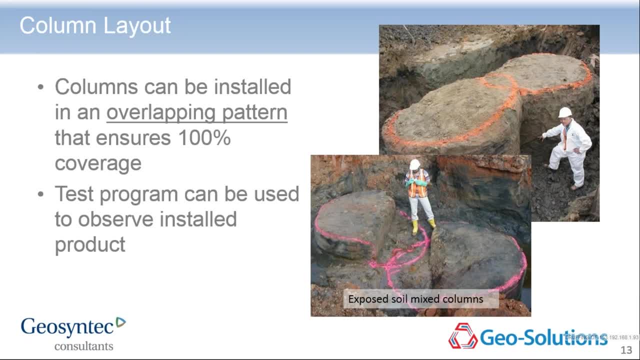 So on environmental sites, a lot of times we're trying to apply the reagent evenly over a large area. So you take all these circular elements, you put them into a grid pattern that provides 100 percent treatment And on some sites the owner or engineer would like to see the soil mixing column. 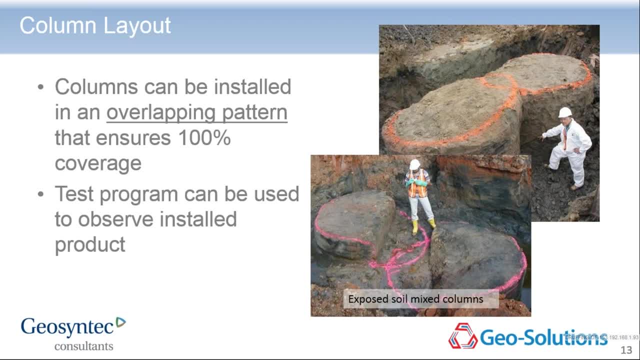 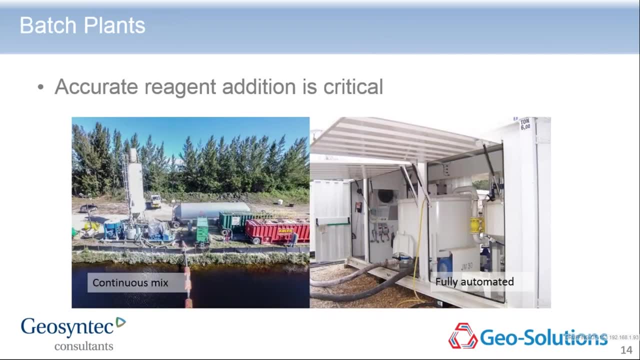 So these two photos on the right are from test programs, where the elements were installed and then they were exhumed so that the overlap could be observed. Okay, This is just a couple example batch plants that are used. Reagent addition is very important. 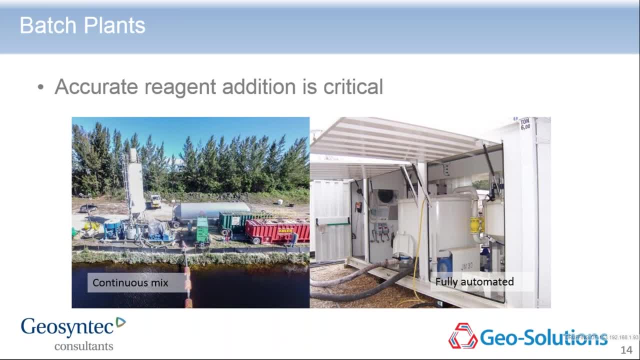 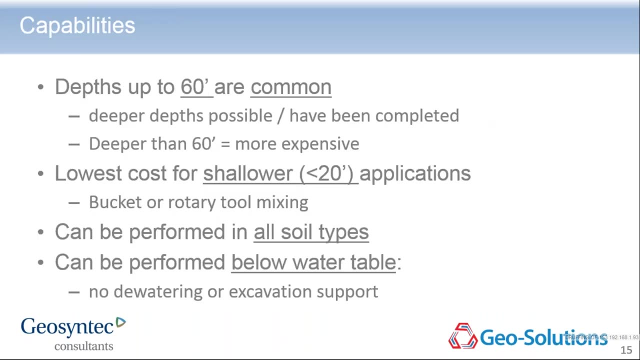 A lot of the reagents that are used for soil mixing are 30,, 40,, maybe even 50 percent of the overall cost of the implementation. So making sure that those reagents are added accurately is a really important part of the project, and you don't want to over- or underdose, for obvious reasons. 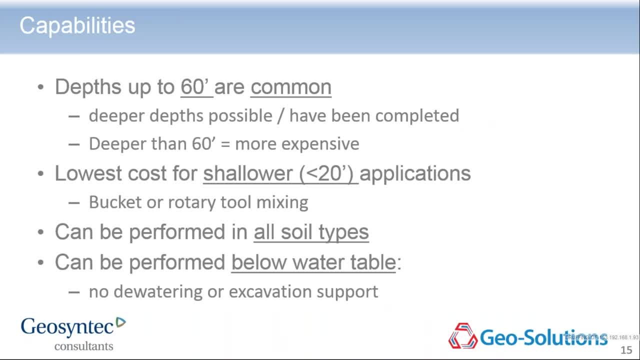 So the general capabilities of soil mixing Depths up to 60 feet are common. The deeper depths have been completed- I think we just did a pilot study last year- down to 97 feet, for instance- But it gets significantly more complicated and more expensive as you go past about 60. 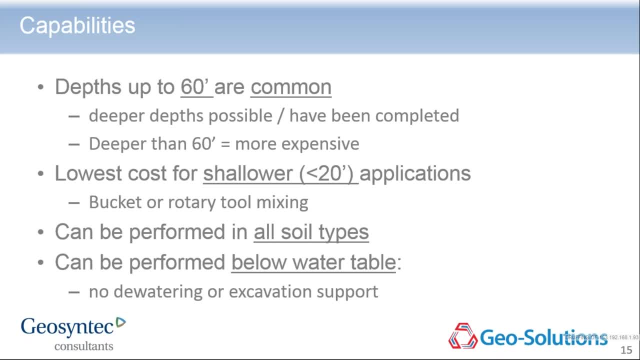 feet. The lowest cost applications are the shallow applications. I put the breakpoint at 20 feet, but it could easily be set at 15 or maybe even as deep as 30 feet, And the reason that the lower cost is possible at those shallower depths is because the more 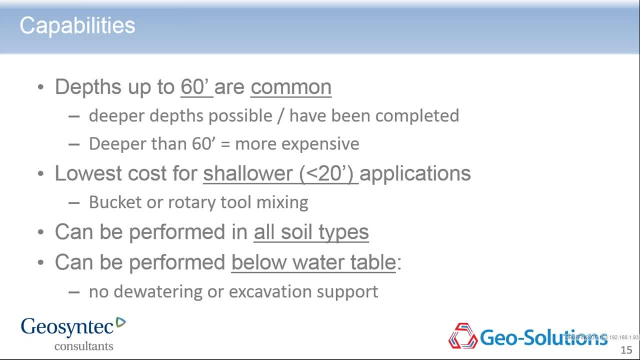 primitive methods. The bucket, the rotary tools can be used at that depth. Soil mixing is generally applicable to all soil types. It has – there's certain things you need to consider in specific types like clays, but it can be used in all soil types. 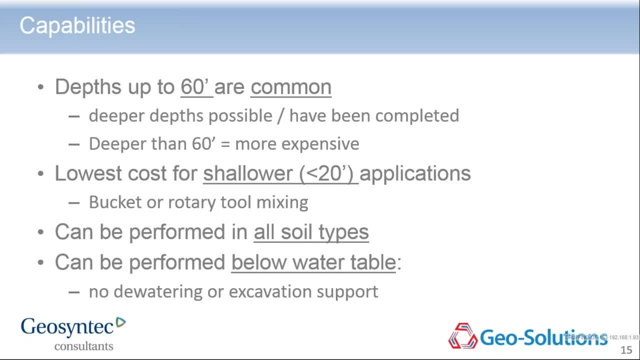 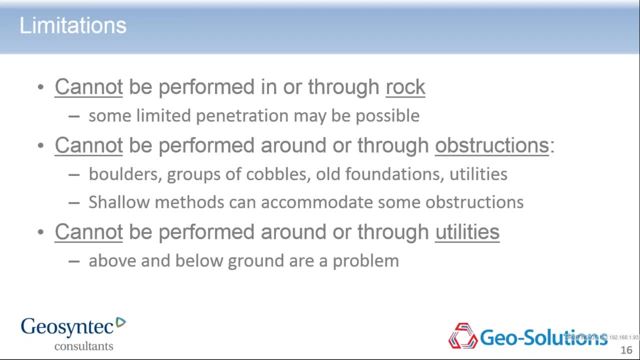 And it can be used below the water table without the need to dewater or support the excavation. Some of the limitations of soil mixing: it's not rock mixing, You know we often get asked: can you put soil mixed elements through soft rock? 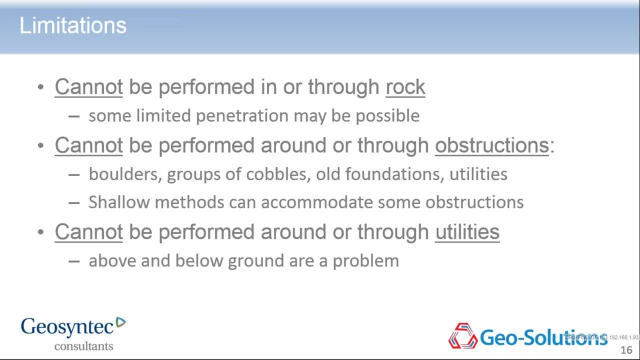 Or tie them into soft rock, And the answer is generally no. There are some tooling configurations that can be changed so that you can get some penetration into rock, or maybe mix through a small layer that's more of a mudstone, But in general soil mixing is not applicable for rock. 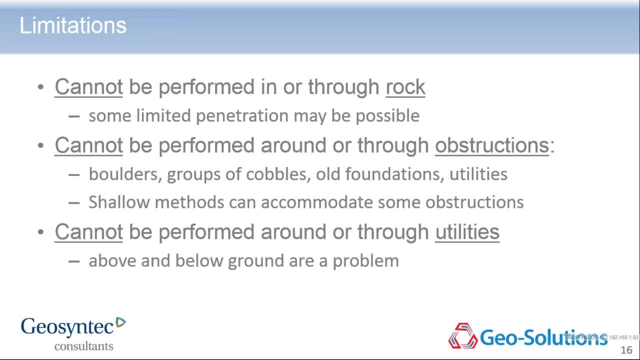 It also cannot be performed in and around obstructions which might include boulders, nested cobble groups, old foundations or old wall structures and utilities. So it's not applicable for rock. It also cannot be performed in and around obstructions which might include boulders. 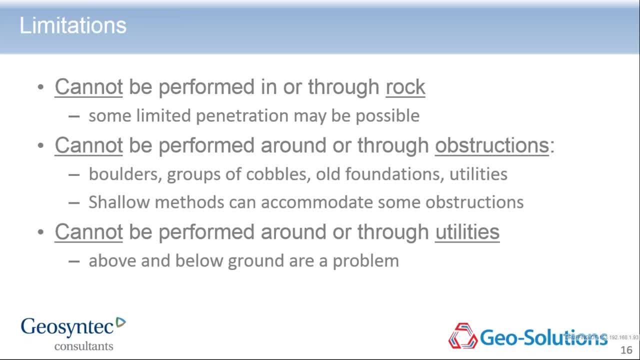 nested cobble groups, old foundations or old wall structures and utilities. Some of the shallower methods, specifically bucket mixing, can be used to accommodate some of these obstructions. You can pull some things out during the bucket mixing process or work around shallow utilities. 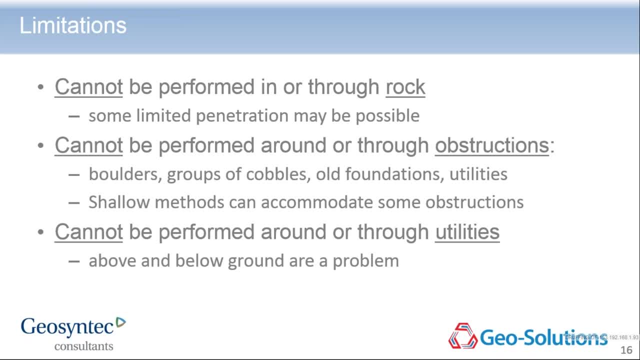 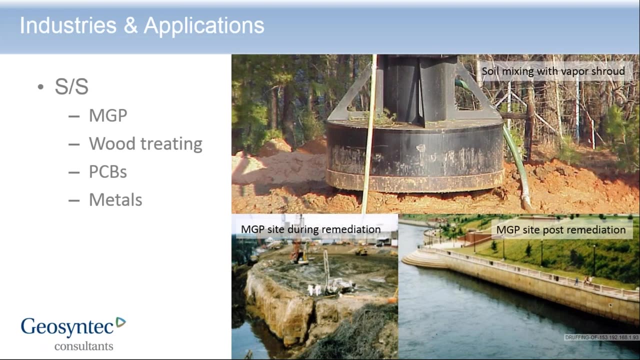 And utilities are a problem both above and below ground, because whatever the depth of soil mixing is below the ground, there's likely going to be equipment that extends at least that height above the ground. So just highlighting a few. Okay, So just a few of the industries and applications where soil mixing is commonly used. 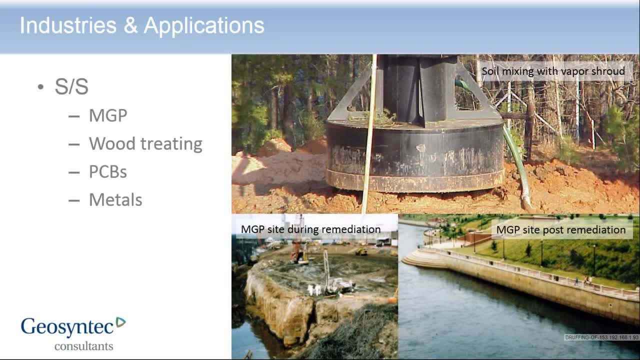 Manufactured gas. plant site remediations are probably the largest application of soil mixing, specifically because the contaminant there being- coal, tar and dean apples- is very challenging to remediate using other techniques, So ISS is a preferred technique for those sites. For the same reason, wood-treating sites are commonly dealt with using soil mixing and 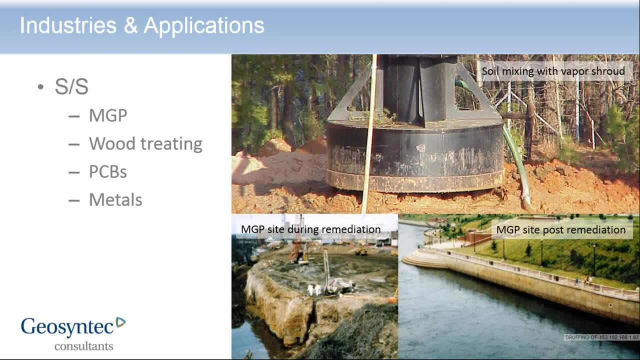 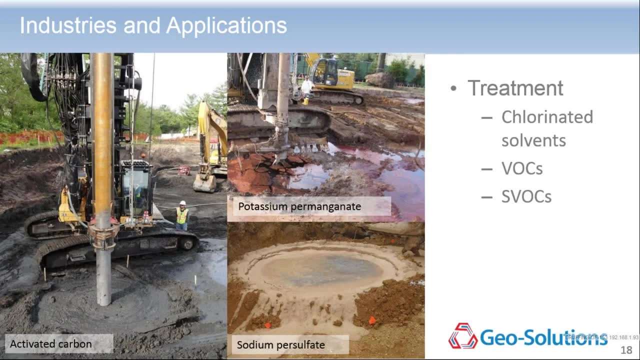 in lesser application, but for specific reasons at specific sites. It can also be used for PCBs and metals, And then for the treatment of VOCs and SVOCs. you can use the soil mixing technique to deliver nutrients, carbon substrates, oxidants, reducing agents, variety of other reactive reagents. 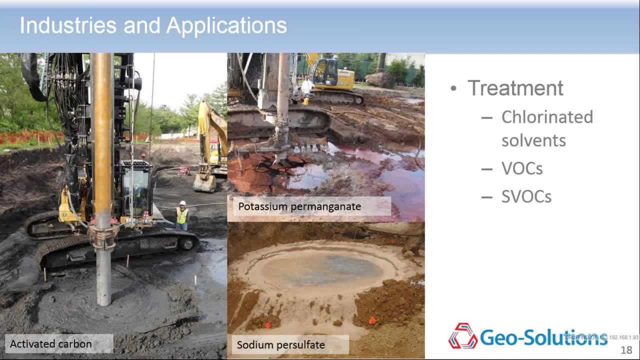 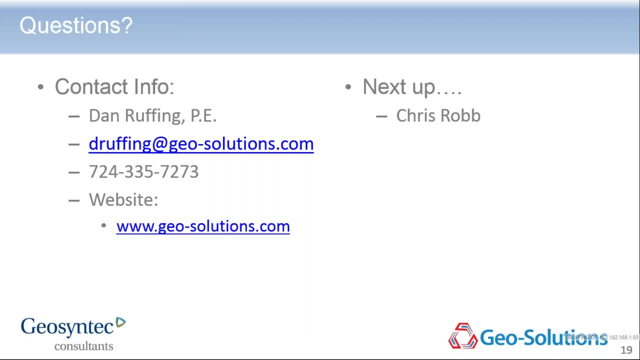 that can be used to physically destroy the contaminants in place. So, Jennifer, any questions before we move on? No, Okay, Before we jump over to Chris or Rob. Excuse me, Sorry, I was just eating a little lunch, No. 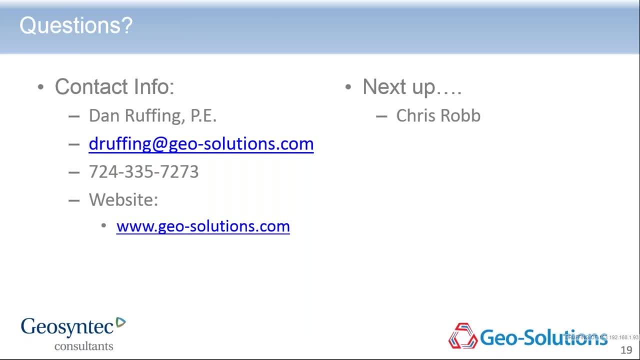 There are no questions at this point, but just a reminder to folks to use the question pane in the control panel that you have for go-to and type in questions at any point. Okay, Great, You can switch over to Chris now. Jennifer. 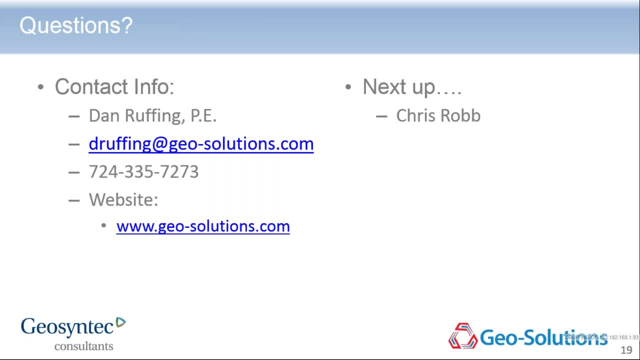 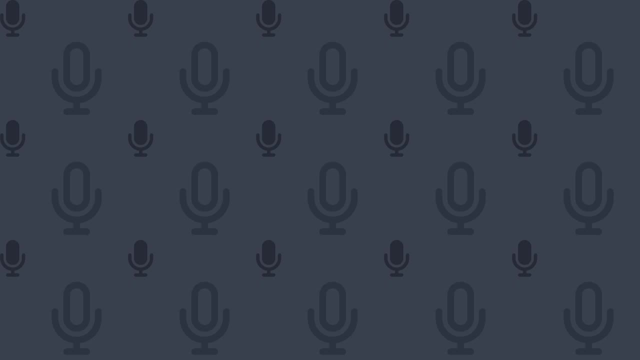 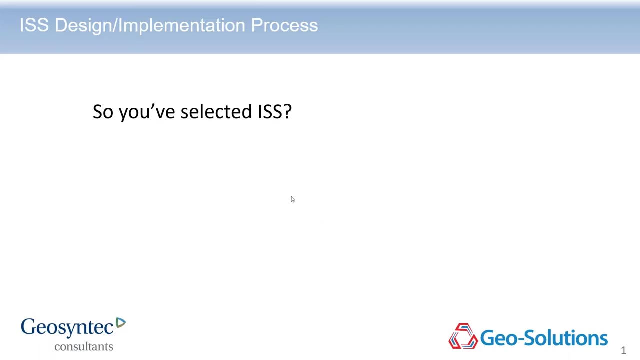 Okay, Great, Great, You can do that. Okay, Perfect, Great. There we go Back to work. Perfect, Pick it up by Chris. Thank you, Thanks everyone. Thanks everyone. we don't have your voice. okay, I'm here now. I had an unmute. thank you so much, Jennifer. yes, and and. 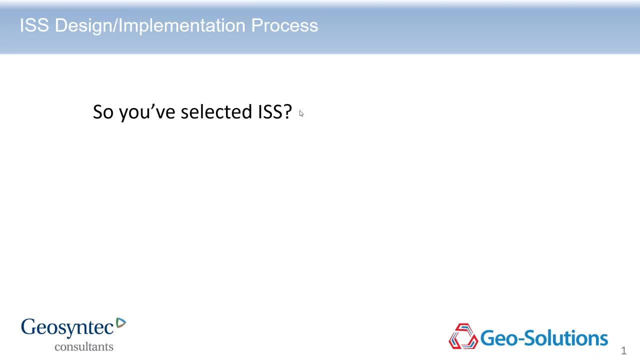 thank you everyone who's attending today's webinar. so really, the focus of the slides and the next things that I'm going to present are really around. you know how to design- and I am an ISS remedy- but also how to design it in such a way that your contractor is going to be able to successfully. 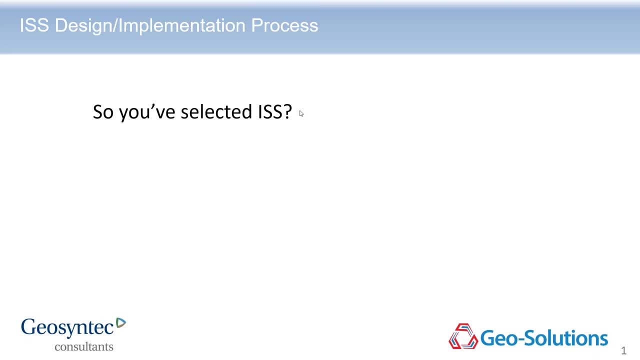 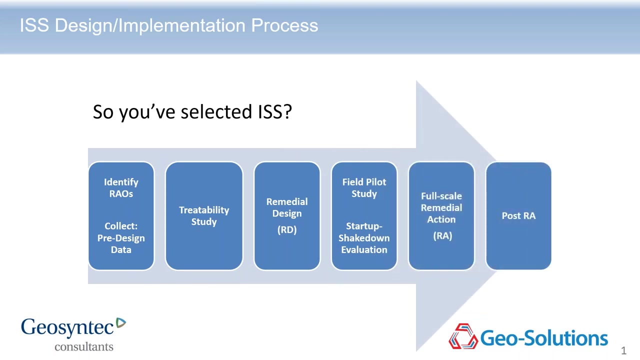 implement it. there's going to be some features of how I talk about ISS in that regard today, and when we talk about the design process, there's various steps that we need to go through or make your you may want to go through, and this is just an example of the various steps you might see in. 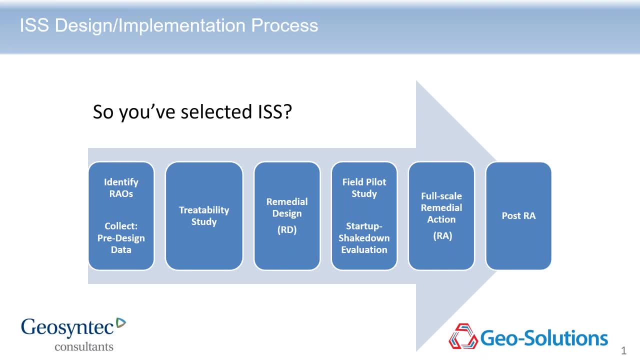 the design process. they're not always necessarily all required. you may not need a field pilot study. it may be a smaller job and you go straight to full-scale remediation. so today I'm really going to focus on these first three boxes: understanding your, what you want to do, your remedial action objectives. 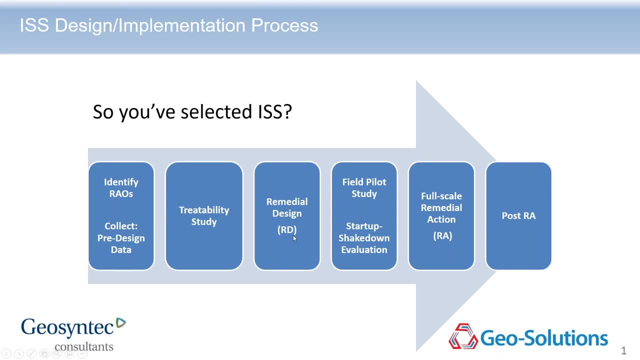 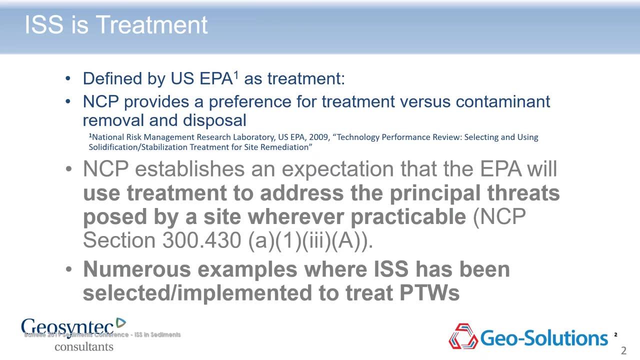 treatability study and then the remedial design itself. but before we jump into that, I just wanted to remind everyone that the US EPA does define ISS as a treatment and if you're looking for the reference for that, the National Contingency Plan has that documented in the in the publication that is highlighted here on the screen. 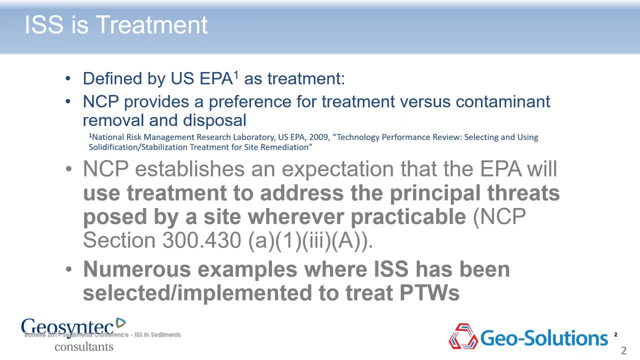 in addition, the NCP establishes an expectation that the EPA will use treatment to address the principal threat waste posed by a site wherever practical. now, 20 years ago, when I first started working on circular sites, the principal threat waste concept was not as commonly used, but we're. 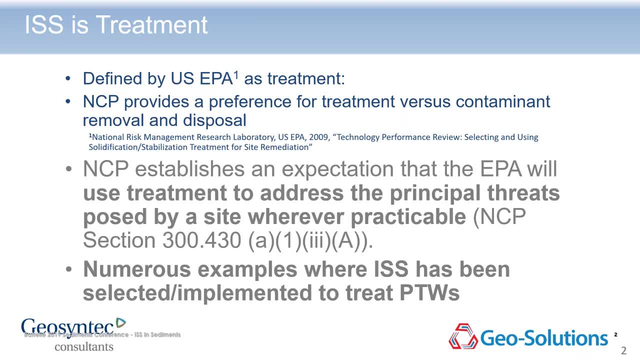 seeing it more and more incorporated into site cleanups and the. the takeaway I want you to have on this particular slide is that ISS is a treatment it is appropriate for addressing principal threat waste and there are numerous examples where ISS has been directly written into records of decision. 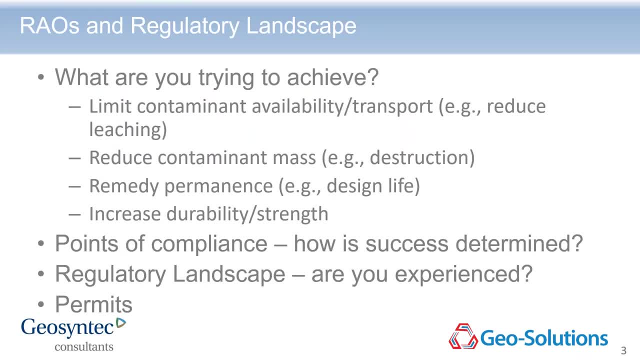 to address principal threat: waste. so, first and foremost in design is think. ask yourself a question: what are you trying to achieve? are you trying to eliminate, limit contaminant availability and or transport to the environment? do you want to reduce contaminant mass? uh, what considerations for remedy permanent permanence? or are you looking just to increase? 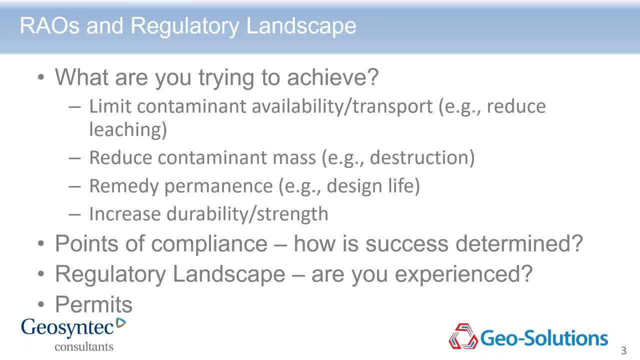 the strength. but understanding your remedial action objectives is key. before you go out and even do any pre-designed data collection, you should also think about how you're going to determine success. how are you going to measure success of this remedy, how you're going to demonstrate it, meet these remedial action objectives and you need to understand who. 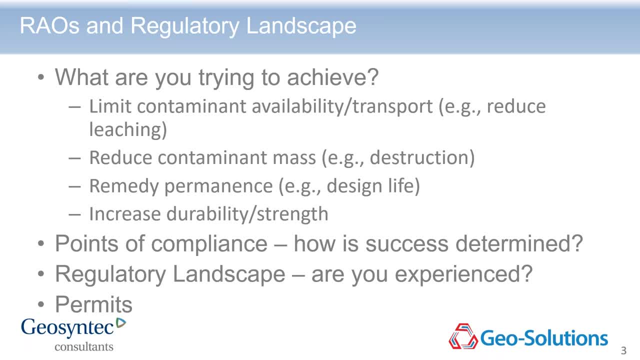 you're working with, um, not just you know the various regulators you might be working with and what a state or another agency's perspective might be on the technology and if they have experience with it, but also, um, you know who you're talking to to help you with the design and and part of that, part of that aspect is: 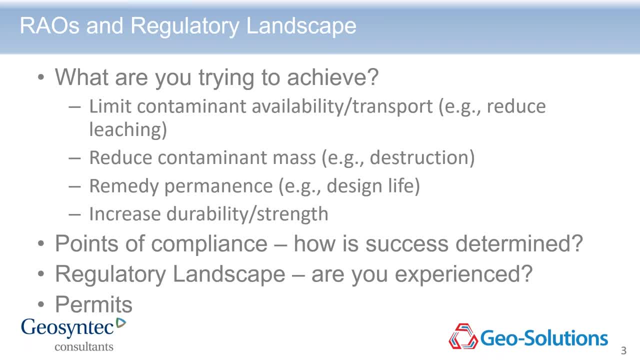 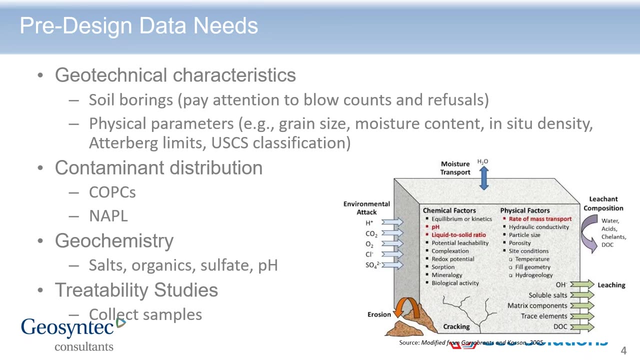 understanding what permits may be required. they can vary from state to state, and a quick example: some states may require an injection permit, some states may not, so it just depends on where you are. for pre-designed data, there's a couple of main areas of data that you want to collect. you want to 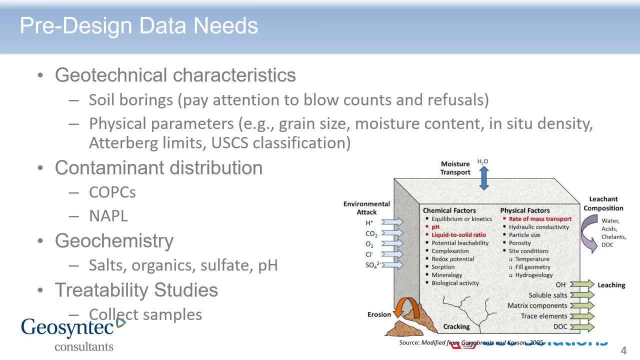 understand the geotechnical characteristics of the soil that you're going to be treating and usually that's first done by doing some soil boring, so I'm sure there's been some pre-characterization done up at the site. when you look at those boring locks, pay attention to blow counts and if a driller hits, 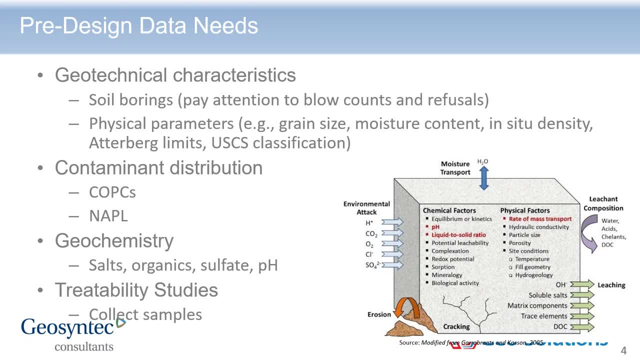 refusal and moves on to another location. really explore that, because refusals can be indicative of an obstruction and, as Dan highlighted, that is problematic or can be problematic for implementation of in situ stabilization solidification. there's a few things you want to understand about the physical parameters of the soil. I want to talk. 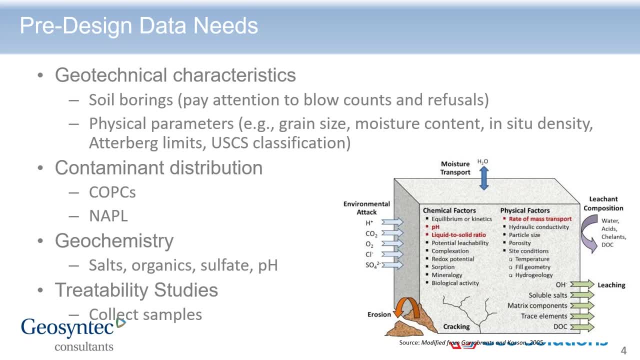 more about that in a future slide. contaminant distribution: what are your contaminants of potential concern? different contaminants and or, if you have non-aqueous phase liquids, may require slightly different mixes or reagent additions to address understanding your geochemistry and, in particular, understanding things that could potentially attack or inhibit the 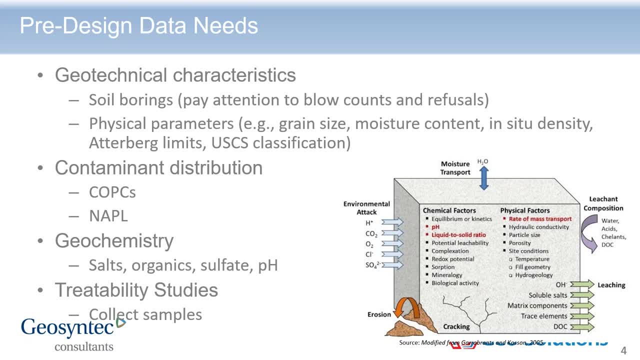 cementitious reactions or cause long-term degradation of the ISS. all of these things can be overcome. it's just a matter of understanding it up front, and and the figure that you see here is just an example of all the different things that potentially you may need to consider. 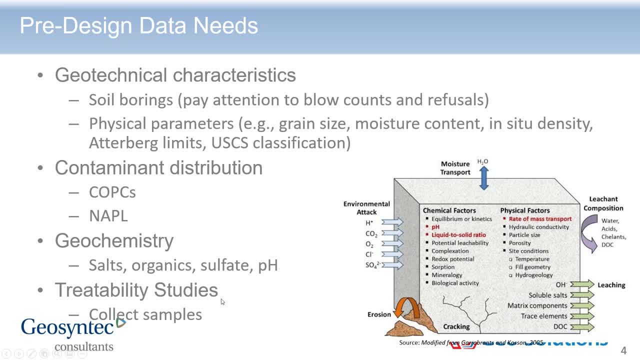 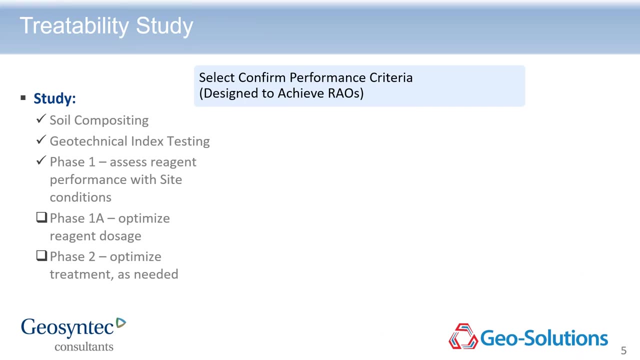 um, overall, and then finally, uh, doing treatability studies to understand and uh, the efficacy of ISS and collecting those samples for the treatability study. I just have a quick slide on treatability studies. I'm not going to dwell too much on this topic. 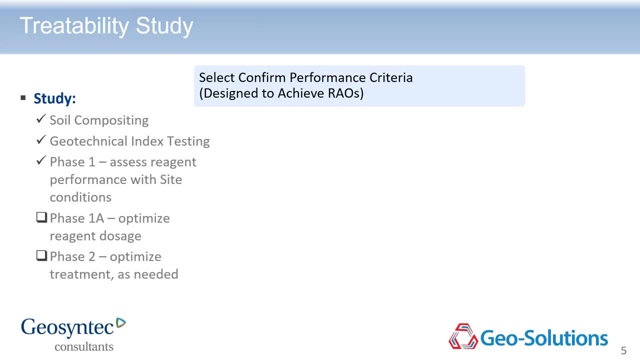 But in general, a pretty common framework that is successful for design is, first of all, once you understand your remedial action objectives, identify your treatment regimens and select the mixed designs you want to test. Then go on and identify the physical performance. 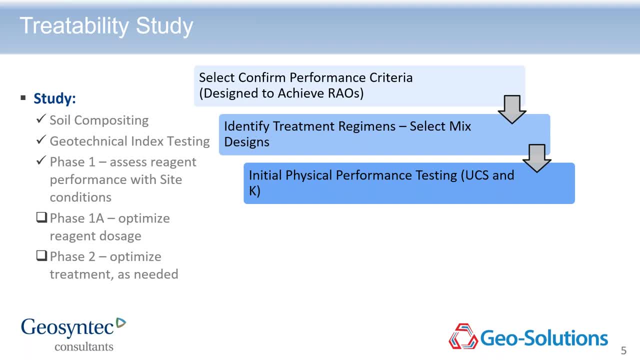 testing characteristics you want to look at. And I want to stop here, pause here just for a second, because if you're going to be screening lots of different mixed designs, you probably want to keep your costs low. Just look at the mixed designs for strength and maybe. 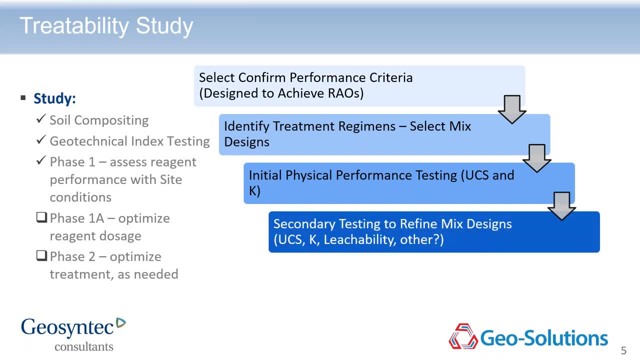 hydraulic conductivity first And the ones that do better. then move on to some secondary testing to refine the mixed designs: strength, hydraulic conductivity, And this might be a stage where you want to look at leachability or perhaps some other characteristics of interest. 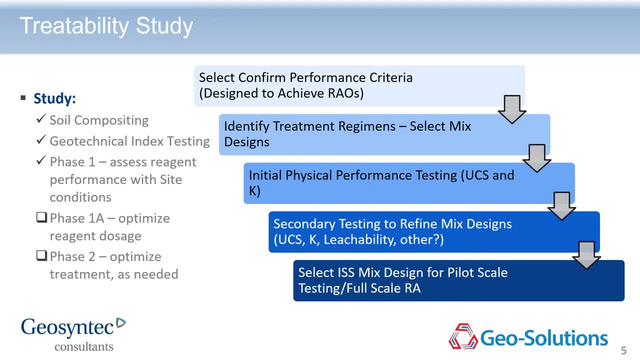 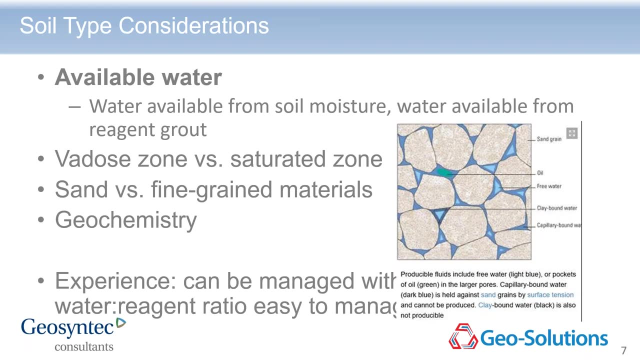 And then finally select that ISS mixed design for pilot scale testing, or maybe just roll right into your full-scale remedial action. Like I said, that all depends on the project. So for soil type considerations first and foremost- probably one of the most important- 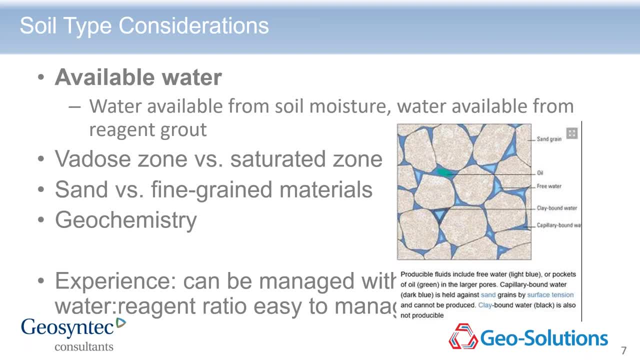 characteristics of soil is understanding how much water is available, not just from the soil moisture, but the water available from the reagent grout. Typically ISS for environmental applications is applied using a wet grout mixture, a cement grout mixture. So that's water and cement And you can. 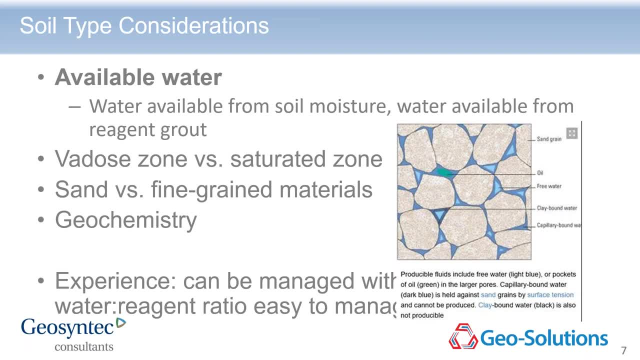 control the water content you're adding to the soil by varying the water to cement ratio. You can make it leaner or you can make it a little more wet. However, if you're going to be doing treatment in both the veda zone and the saturated zone, 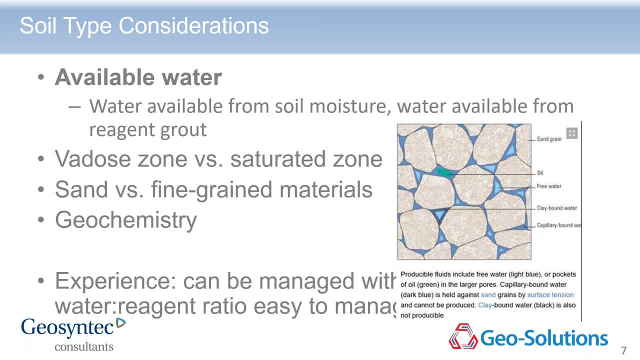 those two zones are going to have a different amount of water that is available to participate in the cement hydration reactions, So you may need to vary your water content And as long as you understand that up front, a contractor or an experienced engineer can help design those mixed. 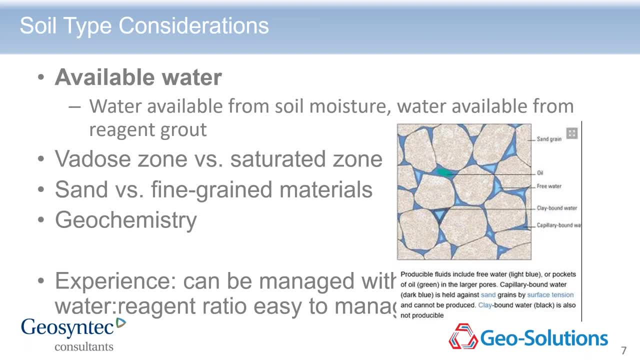 designs to account for those changes in the available water. You also see differences between trying to do ISS in the sand versus a fine-grained material, And oftentimes with fine-grained materials, especially clay particles, we find that the water is not as good as it used to be. So you 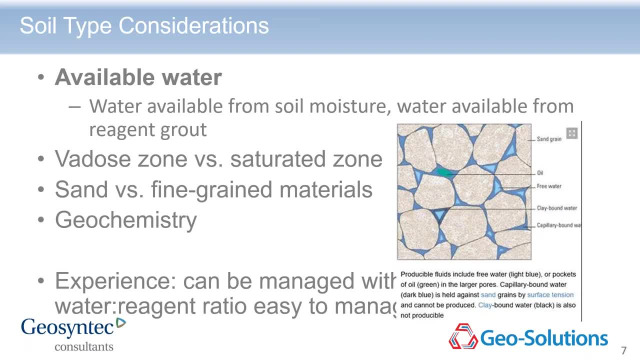 may find that they may have very high moisture contents, but because of the capillary action of those tight clay particles and you find that a lot of that water gets bound to the clay and you actually it's not available to participate in the cement reactions. So the final point here: 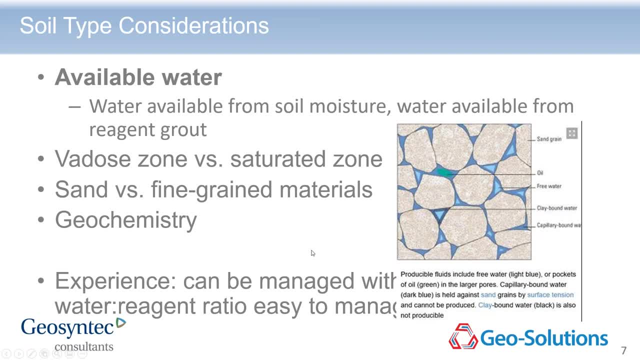 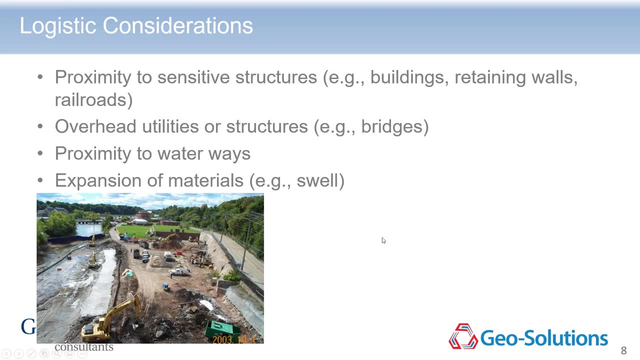 is experience. This can be easily managed with appropriate water reagent ratios. Okay, So some logistic considerations, And Dan touched on this a little bit. I'm going to touch on a little bit more. but when you're designing ISS, you want to consider your proximity to sensitive structures. 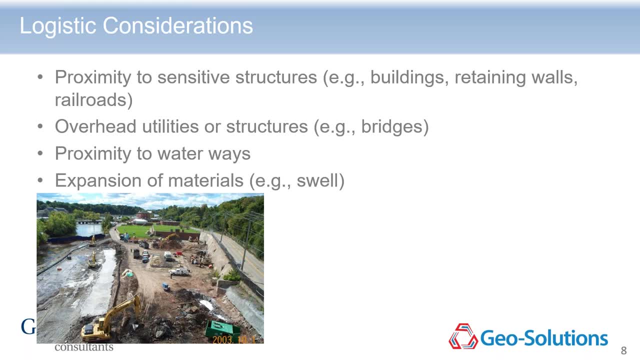 could be buildings, retaining walls, perhaps a railroad, Overhead utilities or structures. perhaps you have a bridge that goes over the site, like in the picture that's shown here, Proximity to waterways And also considering that when you're adding cement and water to the soils. 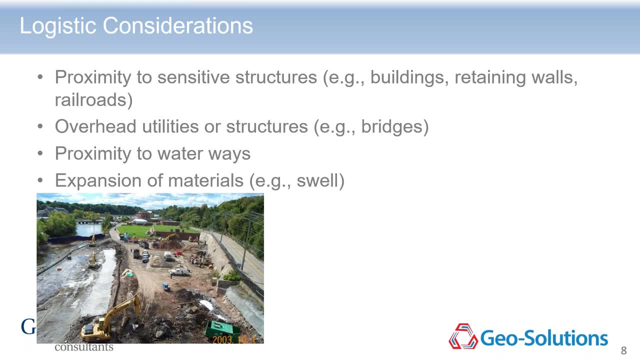 to treat it. it's going to expand. So you want to consider that And then you want to consider the ability to expand depending on the soil type, And you need to account for what you're going to do with that, those expanded materials. Are you going to dispose of them offsite? Are you going to 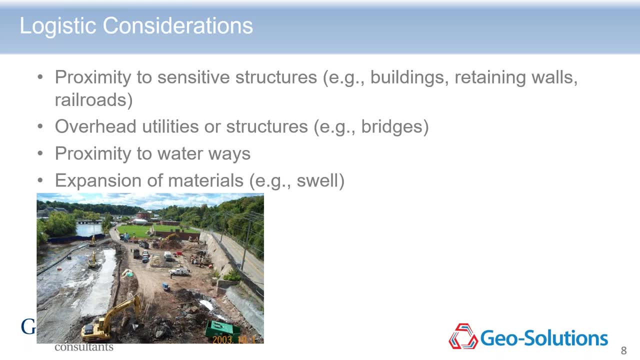 incorporate them in some new site grades. You just have to work with your contractor and your engineer to figure out how you want to address those materials. I like this picture here because it highlights several logistic considerations. We have here a gravity retaining structure. We 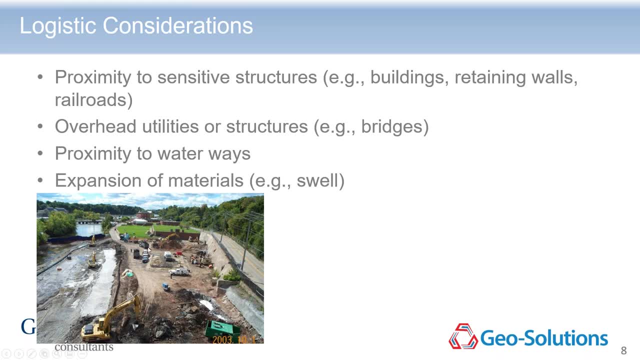 have here a river that's temporarily dammed, that we're, and we are preparing this site to receive ISS, And we have a former water treatment plant with sensitive structures as well. So we have a lot of different things going on here And then fast forward to when we started. 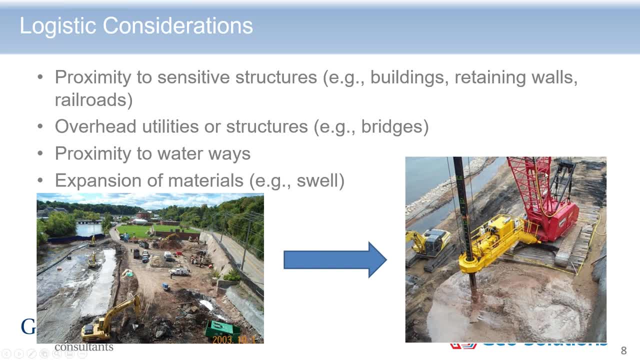 the ISS project. This is the same site You can see here. now the riverbank's been restored and is now functioning as an engineered control to prevent the ISS treated materials from entering the river. It's a berm with a ditch here And this is the actual waterway, So you can see. 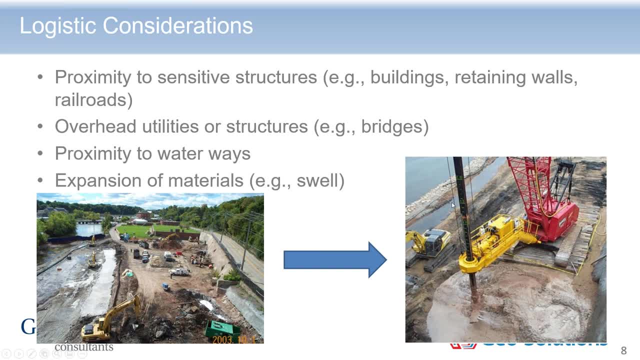 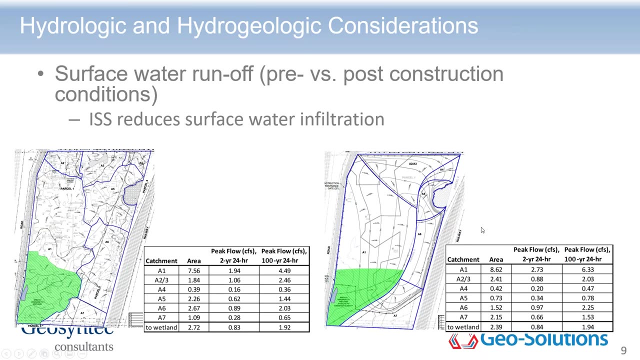 even though this site is very, very tight or narrow logistically, you can still get this equipment onto the site with just some appropriate logistic considerations and design Hydrologic and hydrogeologic considerations. Many municipalities and states or counties have requirements for pre versus post-construction. 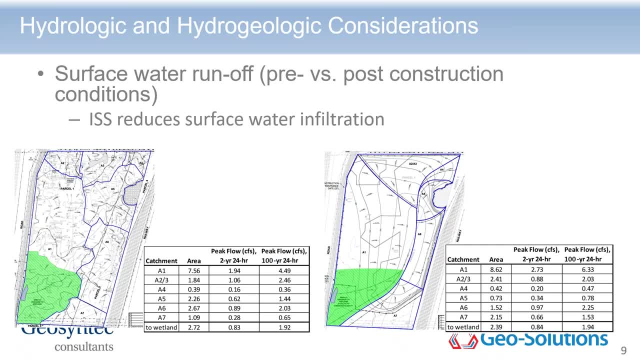 surface water runoff And you may have to have a. you may not be allowed to have increase in pre to post construction runoff. so this is just an example of that consideration. the thing to remember is that ISS is a relatively impermeable material. typically it will reduce surface water infiltration in most. 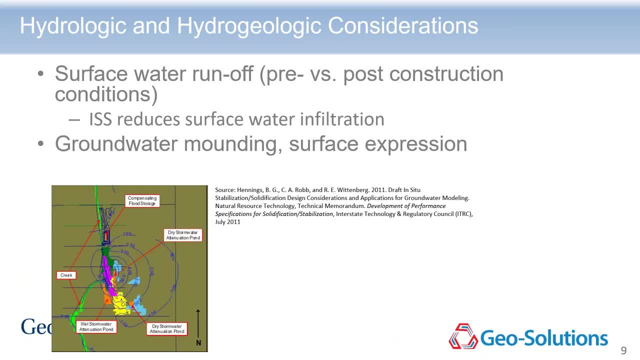 designs, and so you need to account for that in your surface water runoff. also, you may need to think about groundwater mounting or expression of groundwater at the surface, in case the ISS interferes with the natural flow of where the groundwater formerly wanted to go. this is not a consideration at all sites, but 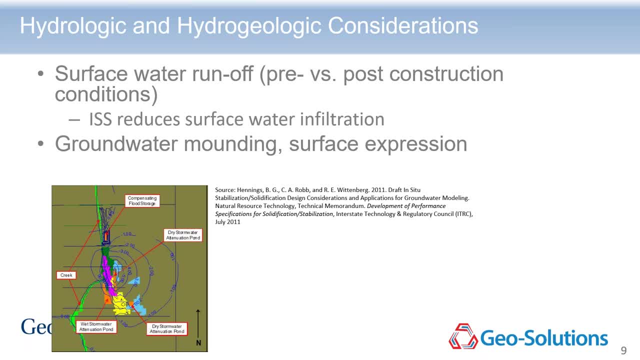 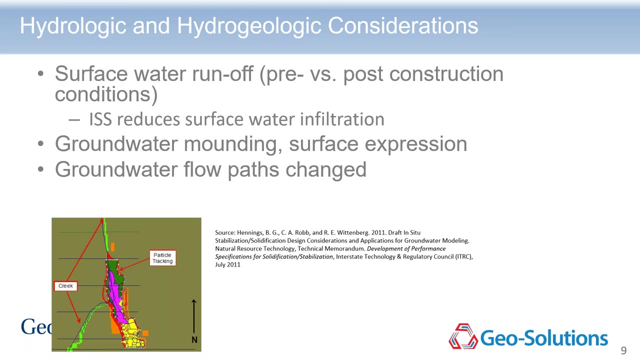 if this was a site that was in Florida, the very shallow water table and we actually had to engineer a groundwater relief drain to provide groundwater path to get around the ISS treated area. also, it may be important to assess- perhaps you want to have surface expression, but the groundwater flow path you will. 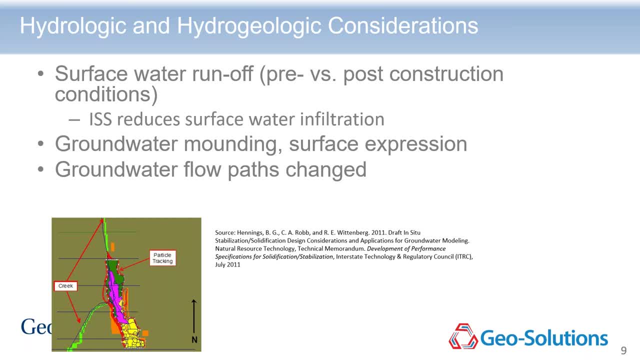 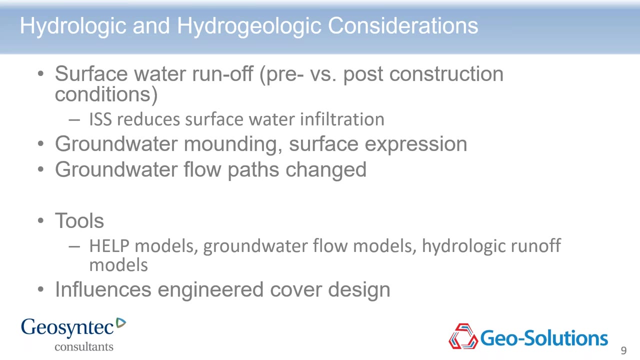 likely change that the groundwater flow path, and it's good to understand that. but then you can use something like a particle trace to help you identify, hey, where the best places to perhaps install a monitoring network to do long-term monitoring of the ISS, and there are lots of tools to help your, the engineers and designers, figure this. 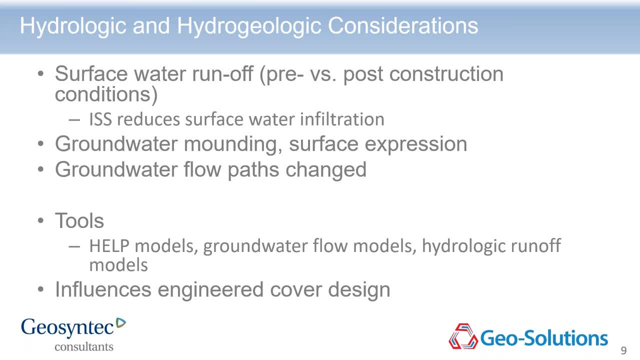 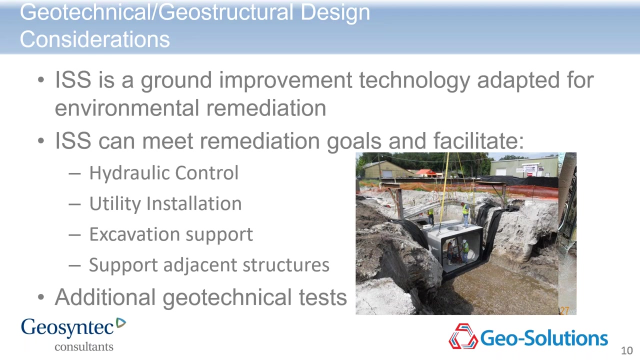 out. there's the help model for cover designs, groundwater flow models and hydrologic runoff models, and all of these can be combined and can help influence any engineered controls you may have to install with the ISS, most typically like an engineered cover or direct contact barrier, geotechnical and geostructural design, as Dan highlighted. 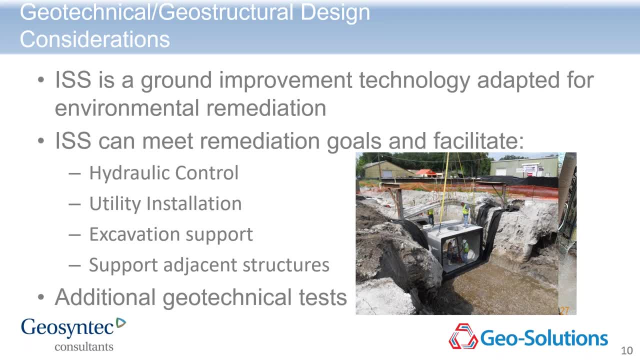 earlier. ISS is a ground improvement technology adapted for environmental remediation. it can meet lots of remediation goals, facilitate lots of different things, but secondarily it can be used for hydraulic control, utility installation, excavation support and support for environment measurement precautions. I'll leave that out to you next time if there are other materials that you follow. 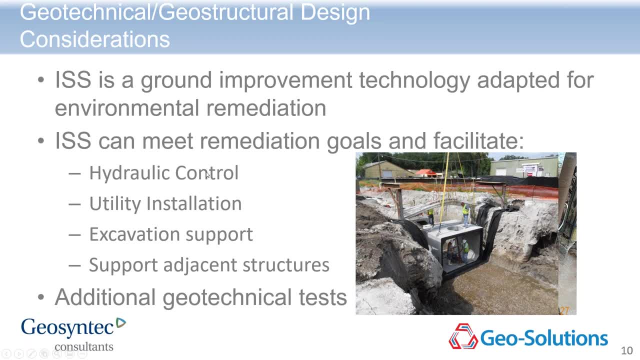 of adjacent structures, and this picture i like because it hits on these first three. right here we are installing utilities. this is a site in florida with a very shallow groundwater table, roughly two feet below ground surface, where we used iss to actually create a retention structure and eliminate dewatering requirements. to install these seven by eleven foot box culverts and you. 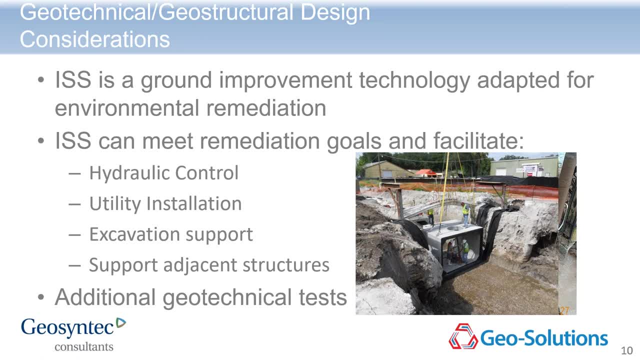 can see. it also provides a safe excavation for workers to work in. and another feature of this is- and it also provides a way to- we're actually installing these box culverts right below a fiber optic bank to evaluate other geotechnical and geostructural design considerations. 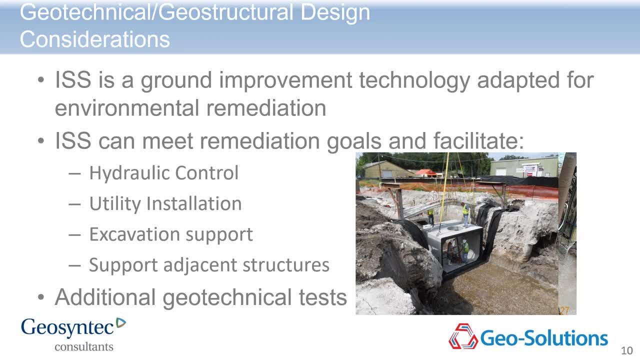 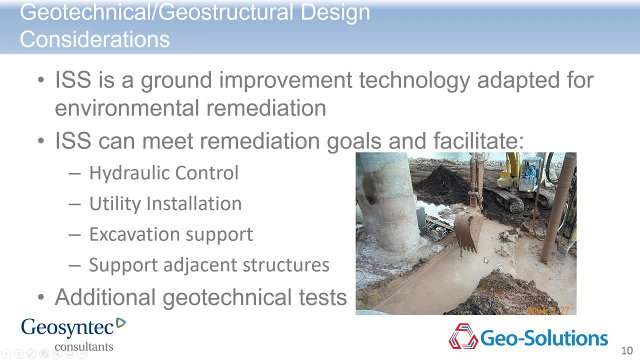 you may need additional geotechnical tests, things like triaxial shear testing, bearing capacity or special density tests for soil cement samples. and then this picture just shows another example of doing iss directly adjacent to bridge pier so it can be used to help facilitate and support adjacent structures iss treatment limits. so this is where 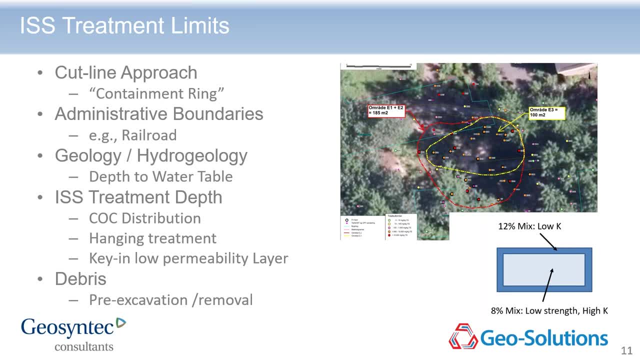 one of the aspects really meets the road for designing iss treatment. typically, what we, what is often done and what we see most often is a cut line approach, where your designer, your engineer, designs a cut line and selects an area that is required for iss, typically limits and depth within the designing the cut line. they may. 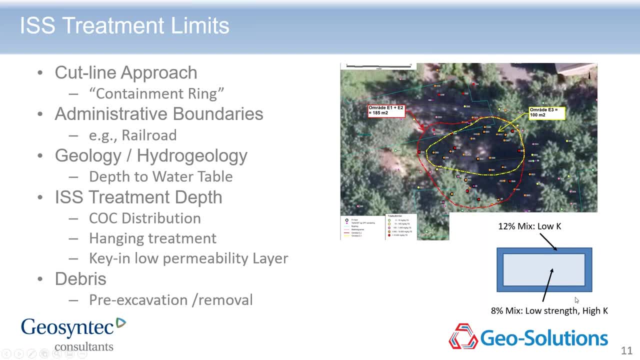 incorporate some special design features. one of those might be a containment ring to help save costs or ease construction. perhaps you want to consider like a low permeability mix on the exterior of the treatment area and a higher permeability mix on the interior of the treatment area that still meets all of your remedial action objectives. 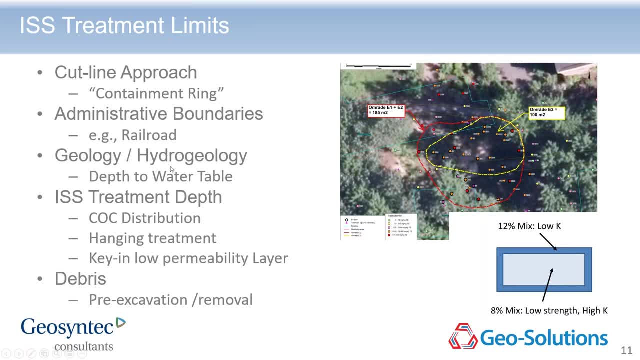 um, what administrative boundaries could there be, like a railroad? what about geology and hydrogeology? very important. understand your depth, water table, and then iss treatment depth. understanding your um contaminant of concern, distribution. are you looking at a hanging treatment where perhaps you only have to treat to a certain depth because the cocs have not, you know, permeated deeper? 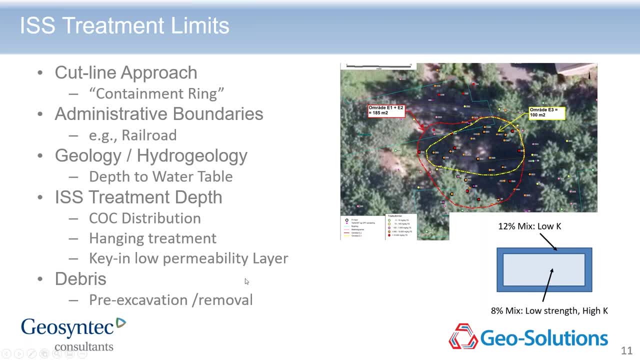 or do you have a low permeability layer that you can key into? and then, finally, understanding how much debris you may have, and especially on a project like an old manufactured gas plant site where many of the foundations still remain in place, you may have to do some. 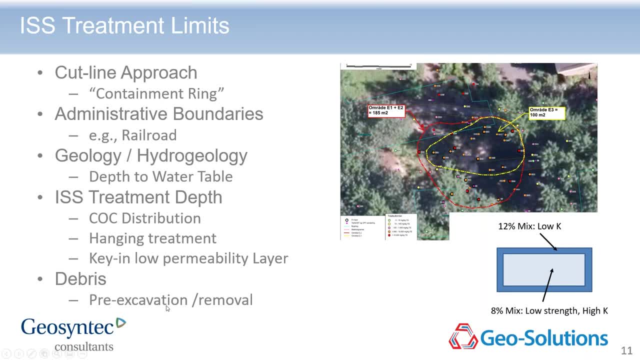 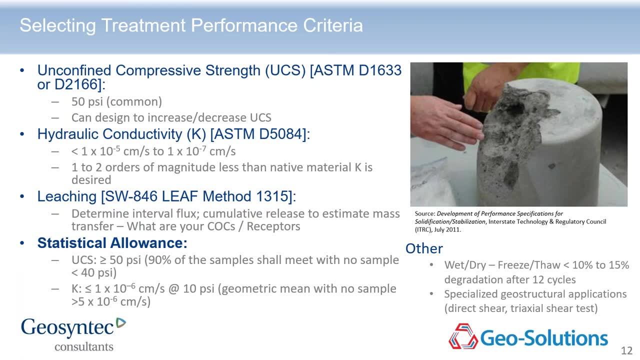 pre-excavation: removal of those structures before the site is really ready and prepared for ISS. Selecting treatment performance criteria: What's shown on this screen? there's a lot of information here, but these are just fairly common ranges And the three most common. 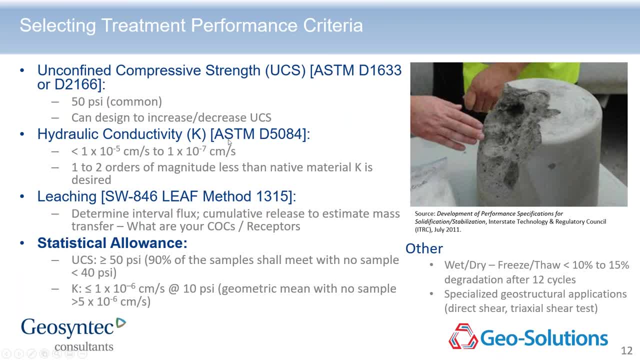 performance criteria are unconfined: compressive strength and hydraulic conductivity. During the treatability study, oftentimes owners and regulators want to see some sort of leaching tested to evaluate how the cumulative release or mass flux has changed in the environment. However, one important point here is: 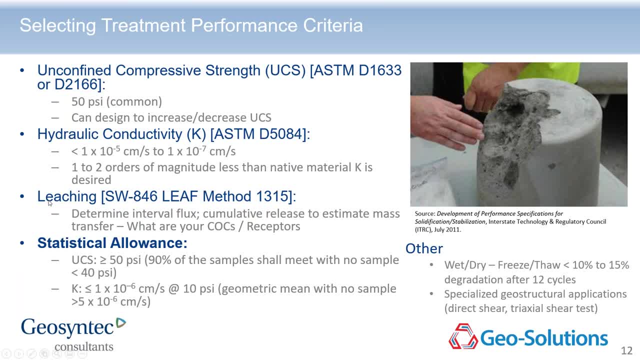 we do not recommend leach testing during full-scale construction. It's best to check these three at the treatability study and correlate the leaching performance to the physical performance that you want to see in the field. And why that's so important is some of 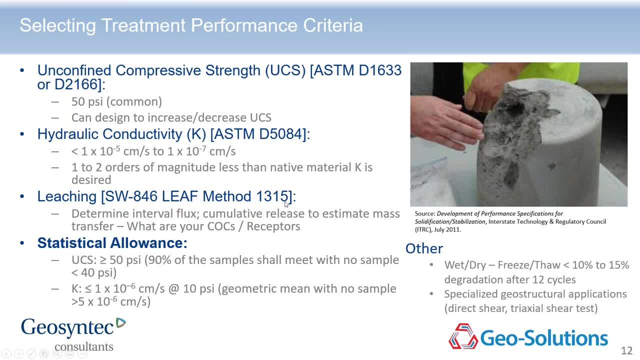 these leaching methods like 13-15, if you do the full method, by the time you get the data or you cure the samples, you do all the leach steps and you get the data and interpret the data, you could be out at least 90 days minimum and closer to 120 days, And it's not practical to 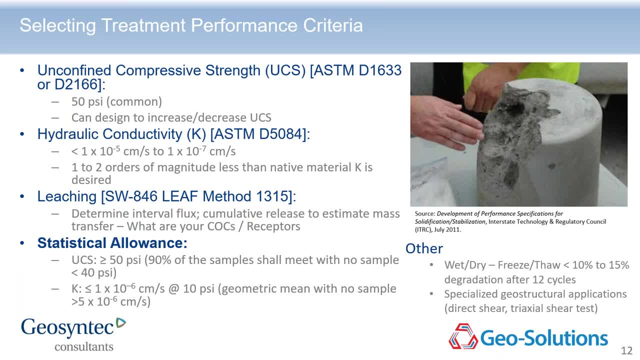 have a contractor wait 120 days to see if they've successfully met a performance criteria. I'll talk a little bit more about that in a moment. When you're considering, though, crafting specifications for performance criteria for a contractor to meet, we always recommend you include statistical 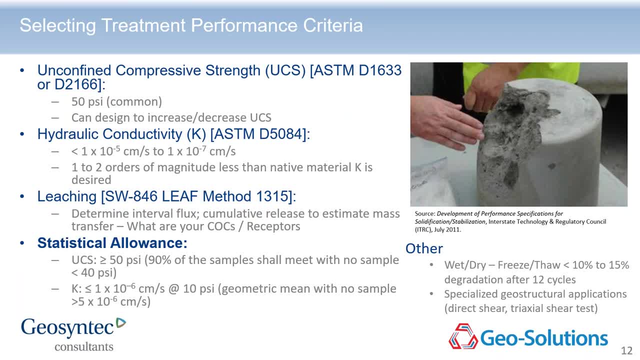 allowances for very, very high performance criteria. So if you're considering, for example, in the material- because the reality is we're building a monolith out there, We're not building individual columns: this one passed, this one fails, They're interlocking like the photos. 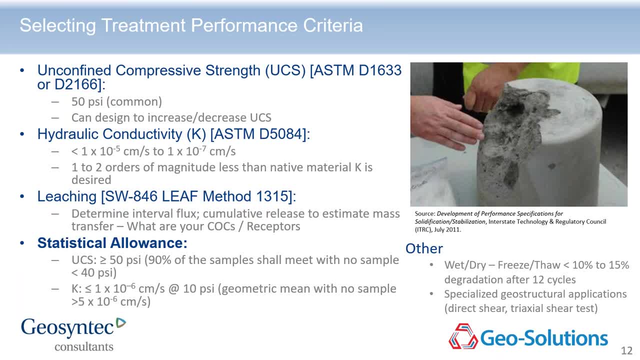 that Dan showed earlier and it's really going to behave as a monolithic structure. So you're looking for, if you want the behavior to be close to 50 PSI, you know perhaps, like 90% of the samples shall meet 50 PSI, with no sample less than 40 PSI. Similar with hydraulic conductivity. 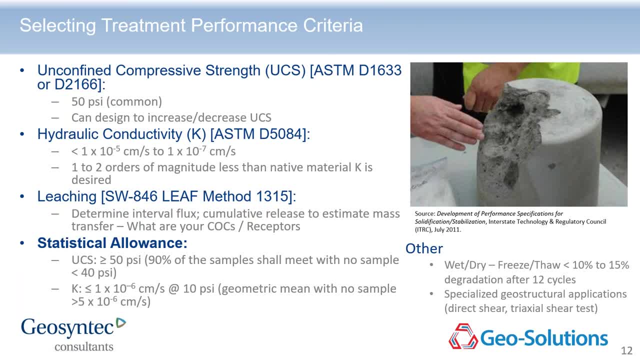 it's going to behave as a monolithic structure. You really want to assess that behavior based on the geometric mean of the hydraulic conductivity samples, with perhaps a floor or a ceiling for how high the hydraulic conductivity could perhaps get. And then, finally, there are some other. 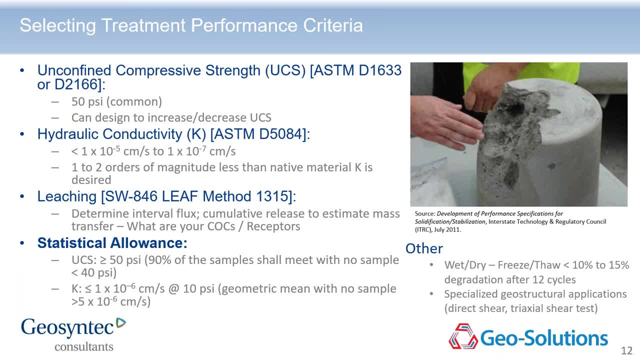 we are finding in other states. there are some other tests that they like to see. One of them is durability testing, like wet-dry and freeze-thaw. We find that the interesting thing about this is that it's not just a matter of how high the conductivity is. it's also a matter of 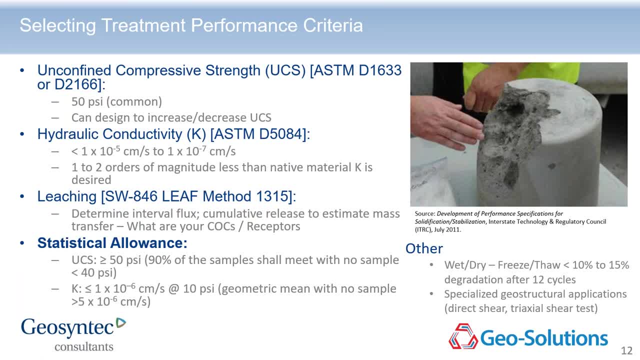 about this test is they're very, very aggressive. They're not as representative of what types of conditions these treatments will experience in the field, And particularly with something with freeze-thaw. if it's a problem, just design around it. Don't allow any ISS treatment to. 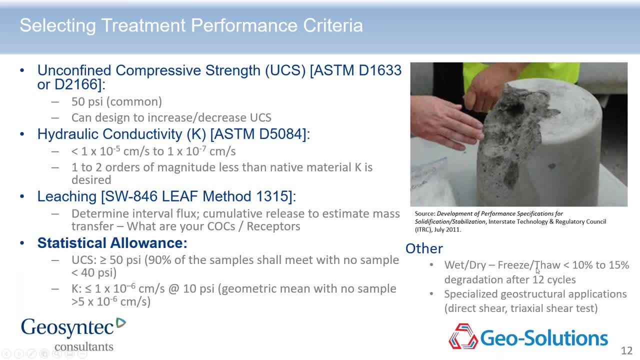 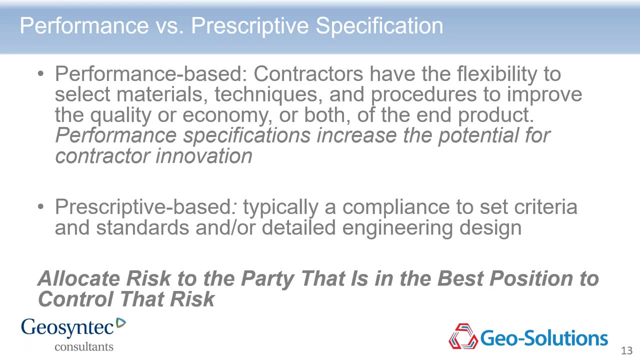 stay above your frost depth. So there are very simple ways to address this without getting into an onerous requirement that's difficult to meet because the test is so aggressive. Performance versus prescriptive specification. So the advantage of a performance-based specification is it allows the contractors to have the flexibility to select materials. 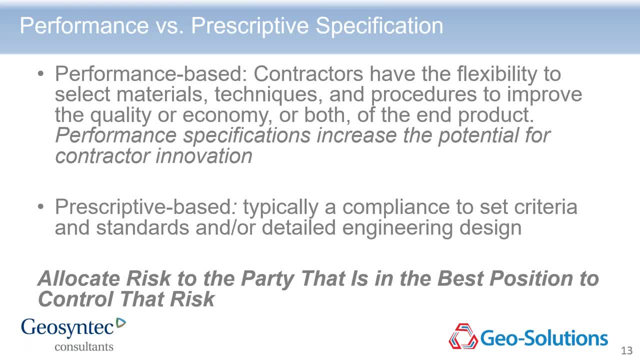 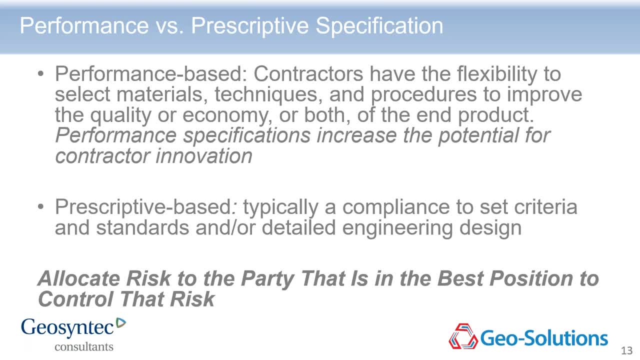 very, very, very, very, very, very, very difficult to achieve. So it's typically where you want to prescribe a set of criteria and your standards that are critical for success of the detailed engineering design. So an example of what that might be on an ISS project is: you've got to have 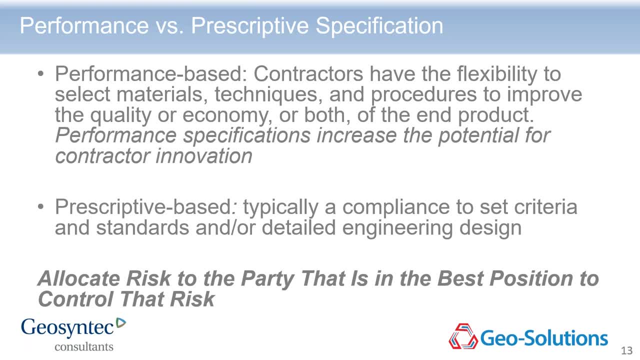 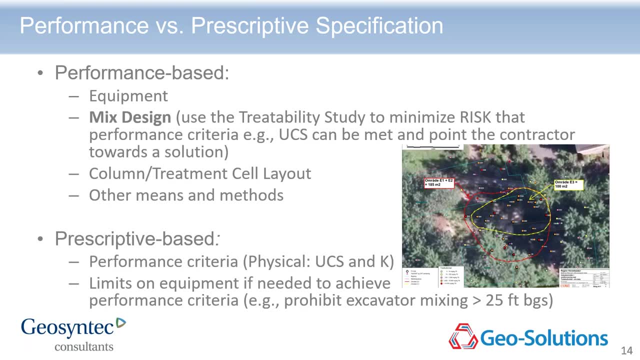 a hydraulic conductivity that is no greater than 5 times 10 to the minus 6 centimeters per second. Perhaps that's something you prescribe, But in general we recommend doing a performance-based specification and allowing a contractor to set up a proper specification for the project. 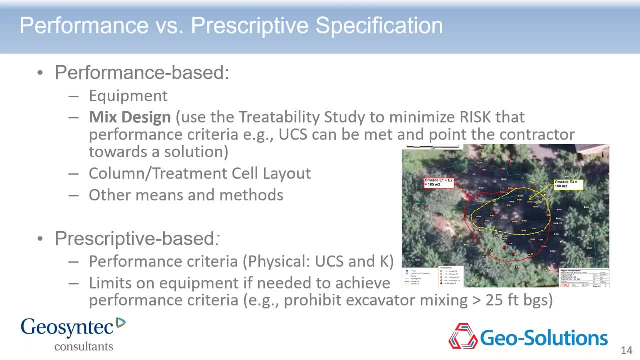 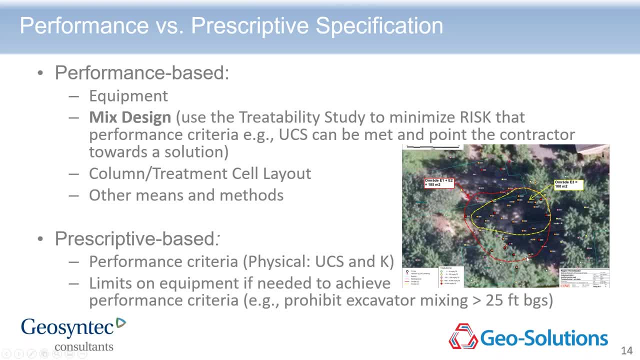 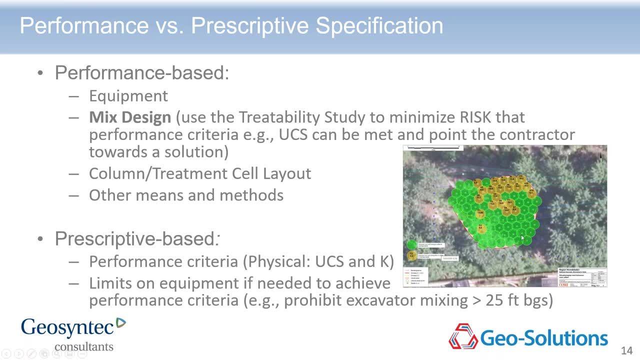 methods. So let me hit on a couple of those real quick. You give them the cut lines. allow them to create the pattern of how their equipment is going to fit into those cut lines. Don't give them a column layout, because they might want to use a different size auger, for example. 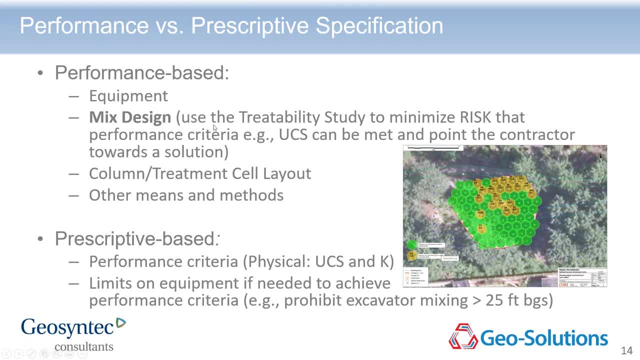 Mix design. I just want to highlight this real quick. We recommend using the treatability study to minimize risk that the performance criteria that you need to prescribe- perhaps strength and ideal conductivity- can be met And you can point the contractor towards a solution And to take it. 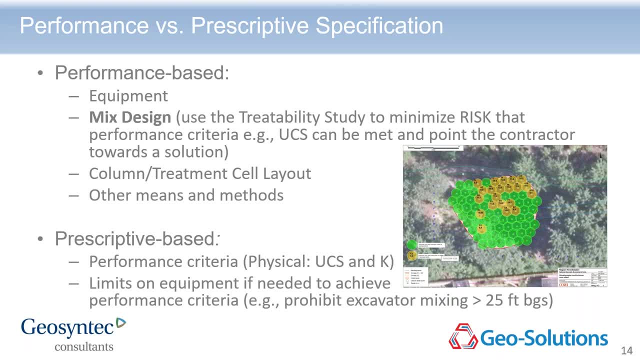 a step further. we often, then, may require the contractor to provide pricing for that mix design. However, we also allow them the opportunity with their experience, Perhaps they know something that may work for them, And we can also allow them to provide pricing for that mix design. 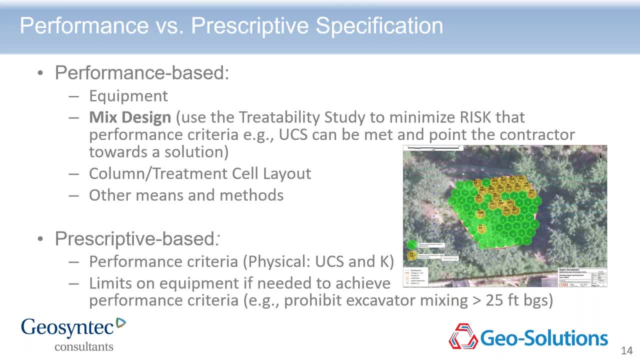 Better. Allow them the opportunity to provide a price for it and to demonstrate it. you know, if they want to, You know. let them use their knowledge and experience to help the project be successful. The only other prescription thing that we sometimes prescribe if there's a limit. 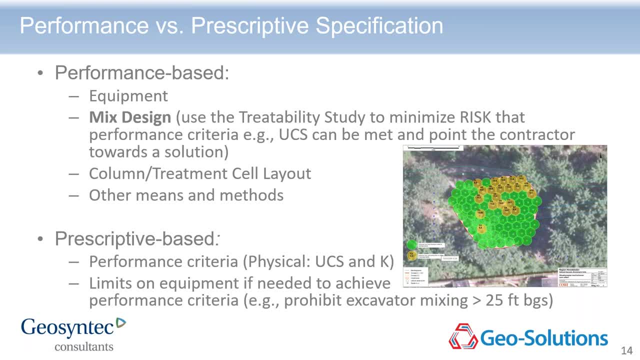 that we need to place on a certain type of equipment. for example, let's say you got a treat to 40 feet. Well, you don't want to get a. you don't want to get a, a bid back where a contractor's proposing to do bucket mixing to 40 feet. I think. 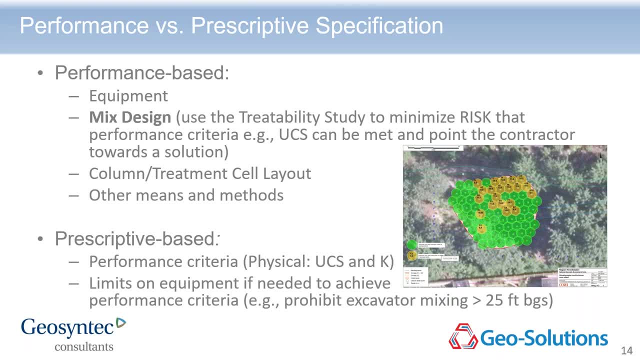 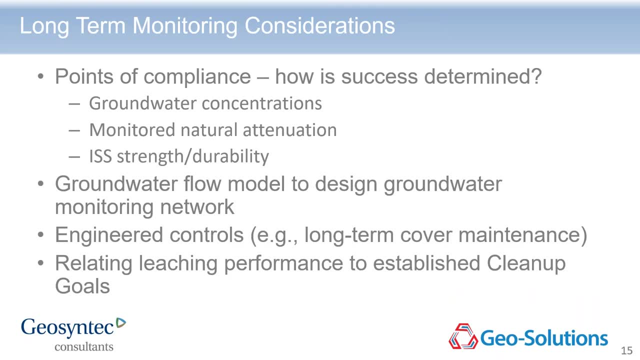 both Darren and Dan would agree with that, So you might want to put some restrictions on that, But other than that, allow the contractors the room and flexibility to use their experience. Long-term monitoring. Go back to one of the first points that I had. What's your point of compliance? 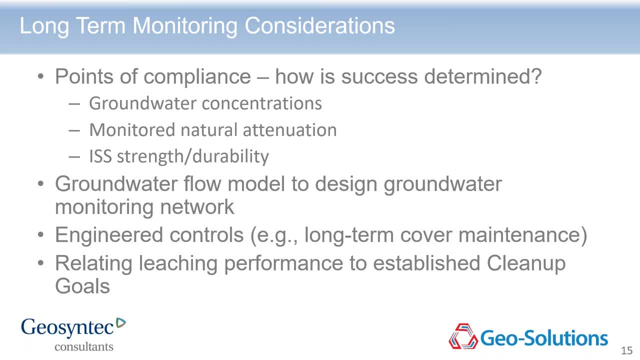 And how are you going to determine success? Is it groundwater concentrations? Are you looking to facilitate monitored natural attention? Is it groundwater concentrations? Is it groundwater simulation? Is it something with strength? You can use a groundwater flow model to design your groundwater monitoring network Engineered controls. Are you going to have long-term 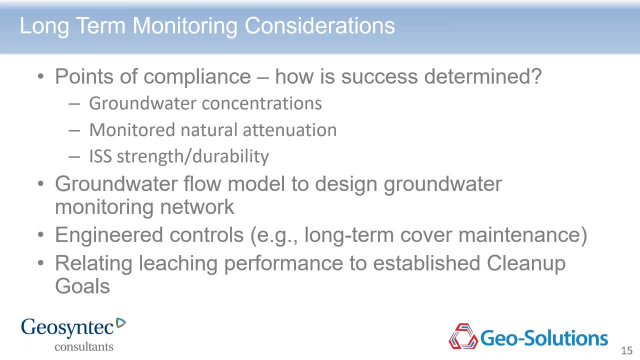 cover maintenance for a direct contact barrier perhaps. And then relating leaching performance to establish cleanup goals. And perhaps the most important point on this line and that we see a lot of is: leach data does not equal groundwater concentrations. What leaching provides you do not gain ground water. What leaching provides you do not gain ground water, And that is long-term cover maintenance. And what the utility of a lead ditch is to use, especially to clean- provide clean water for any type of 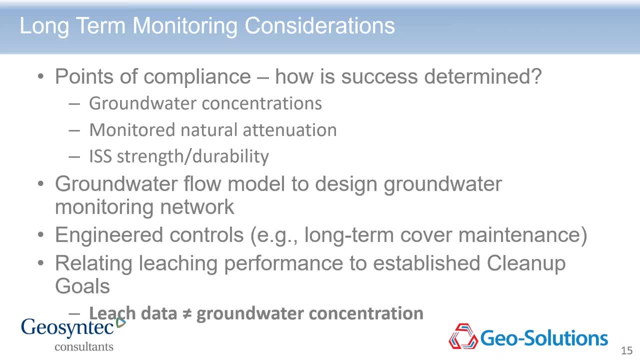 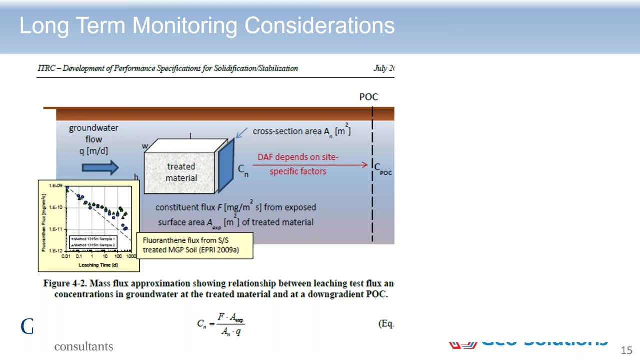 equal groundwater concentrations. what leaching provides you is cumulative mass release and mass flux type of information and a more appropriate way to use this information is provided in the itrc document. development of performance specifications for solidification and stabilization and, very simply, if you know what you want your groundwater concentration to be at your 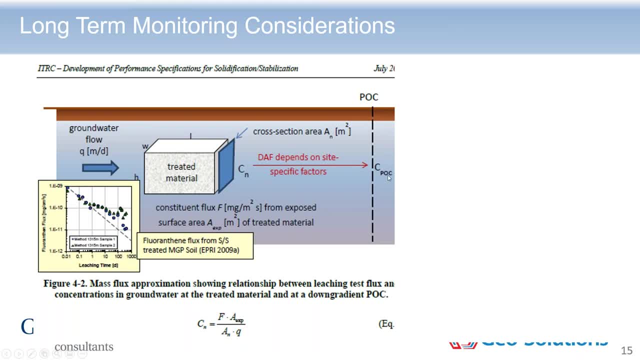 point of compliance. let's say it's a- uh, you know some sort of tier one groundwater level, groundwater control target level, whatever your state calls it. you can plug that in here. you can back calculate, you think, considering site-specific factors such as a dilution attenuation factor. 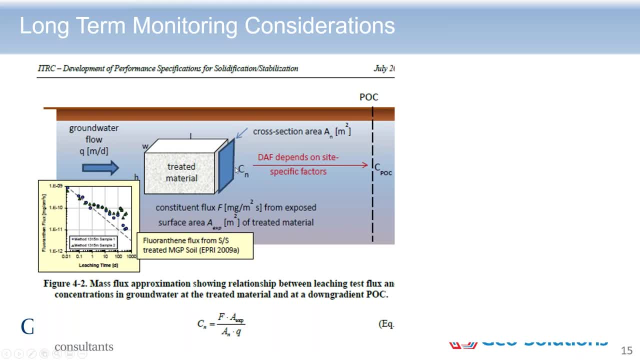 to what that concentration needs to be directly adjacent to the monolith and knowing the flux data. or then you can use a simple equation like this to establish what type of flux is allowable to come off of that treated material and then directly correlate flux to a performance. 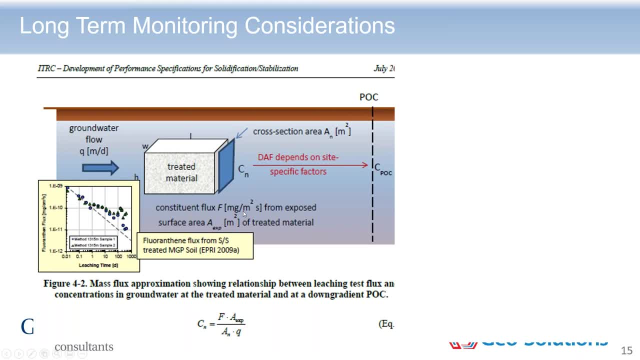 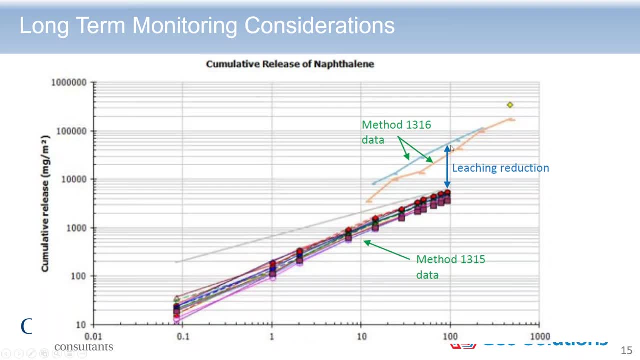 standard, if necessary, for the treatment. the other way that we're seeing leach data used more and more- and this is a more complex analysis- is where you establish the leaching of the material before it's treated and the leaching of the material after it's treated, and doing an analysis like 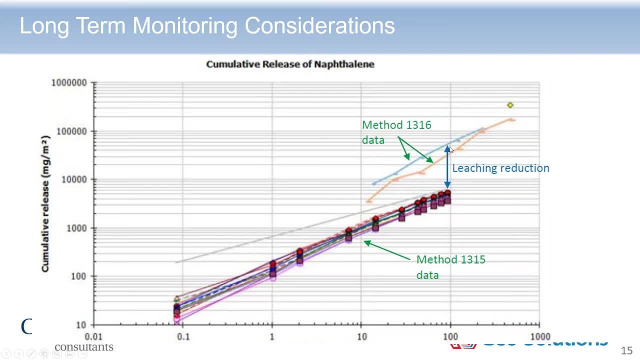 this does require some data transformations, but what you're really looking to establish is: how much have you reduced the leaching pre-treatment to post-treatment? and perhaps a target that you may set as an owner of a goal or that a regulator may desire to see is, let's say, 90. 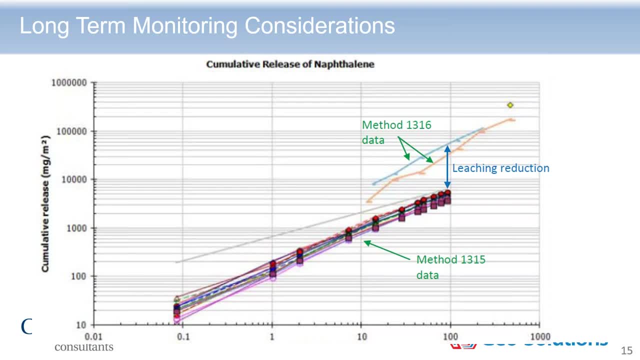 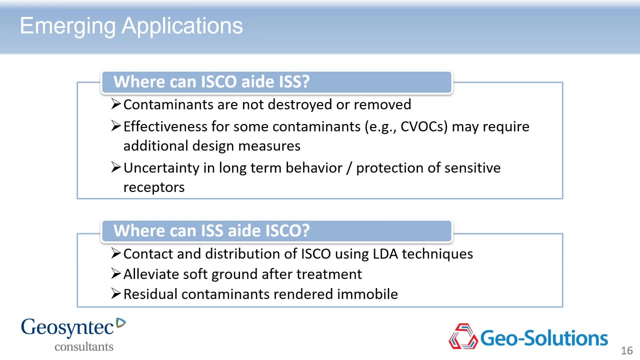 reduction of leaching. so this is the second way that we're often seeing leach- data use. and finally, i want to talk just a little bit about emerging applications and, in particular, what we're seeing more and more of is in-situ chemical oxidation being blended with iss. 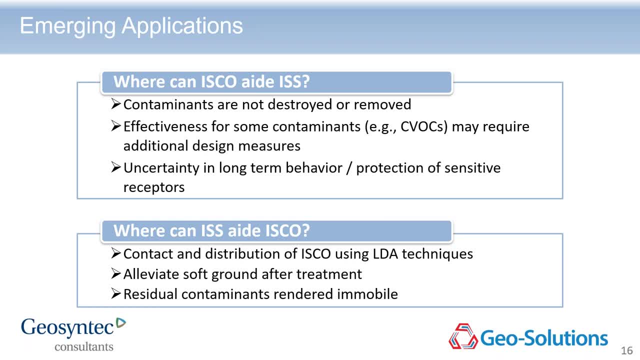 and they're really companion, companion technologies and it can. isco can really aid iss where you have contaminants that need to be destroyed and you have too much uncertainty in the long-term behavior. and iss can really aid isco, especially using these large diameter auger techniques to alleviate soft ground conditions after treatment. and this is a. 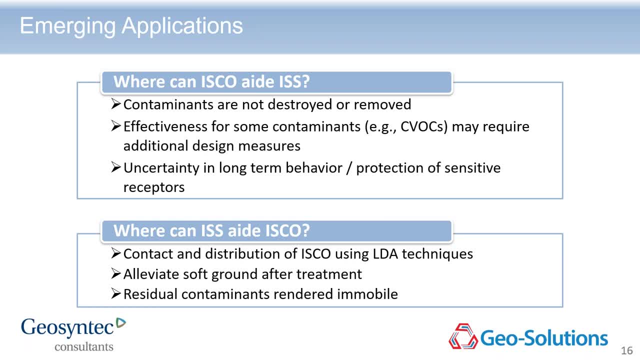 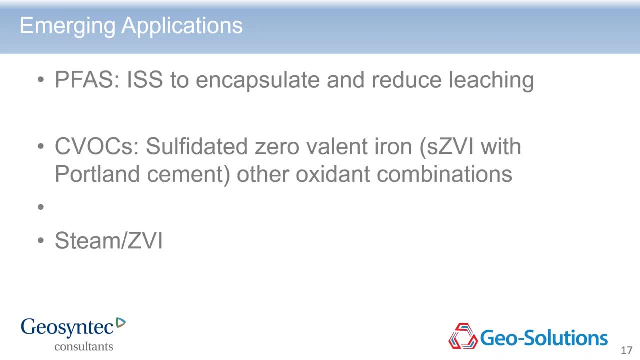 very, very common problem over in europe that i will touch on in one of our case studies. finally, for some additional emerging applications: um, people are beginning to look at iss to encapsulate and reduce leaching from pfos, contaminated soils and chlorinated uh bocs. now this is already being done with some reagents like potassium permanganate, uh and persulfate. 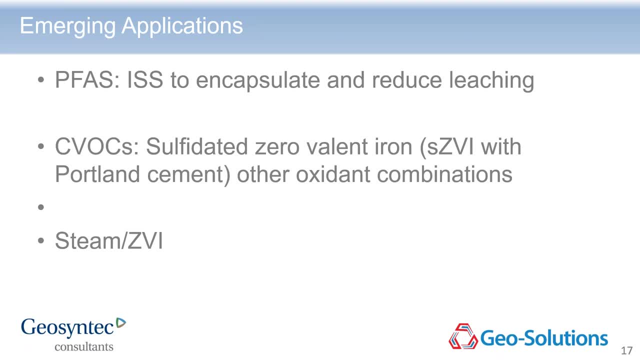 but there has been. there is some more recent research that's being done over in europe on a whole new set of zero valent irons called sulfidated zero valent irons, uh, in combinations, portland cement, and they are starting to have some success. and then, finally, uh, steam zvi has 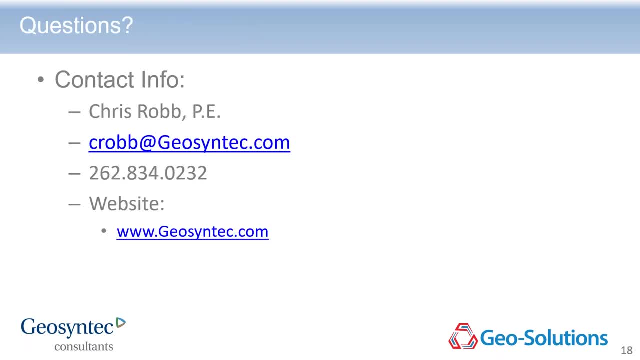 become. we're seeing more and more of those types of projects, um, so i wanted to pause here and see if there are any questions. yes, quite a few have come in. um, some of them are maybe more for for darren. so i i've been dan, so i will wait till the end, but, um, uh, i'm going to pose this one, which is: 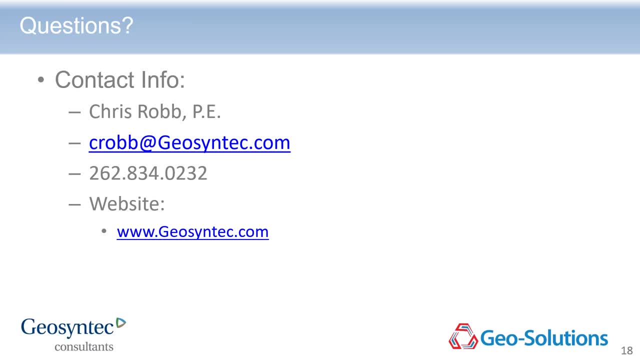 a little bit more to the side of creative thinking here. um, so wondering about iss: if you've got a lan, an old landfill that's maybe leaching some metals to groundwater, so can you mix it up and do iss on like an old closed landfill? so is the question: can you do iss on an old closed landfill? 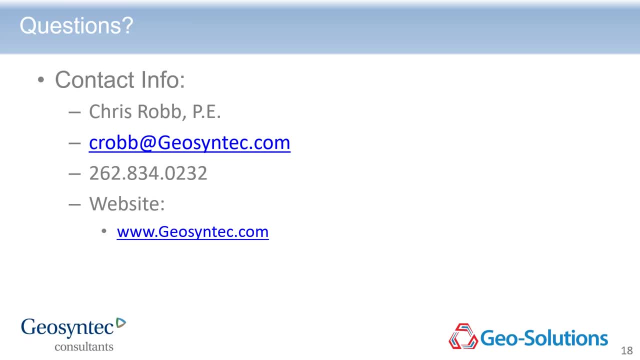 or any any experience with it too. i guess you don't want just a theory, but practical. yeah, yeah, i can, i can take a shot and then, dan, if you want to chime in. so iss is excellent for metals, um, especially the cationic metals, um, and for a lot of the metals that you might see in a landfill. 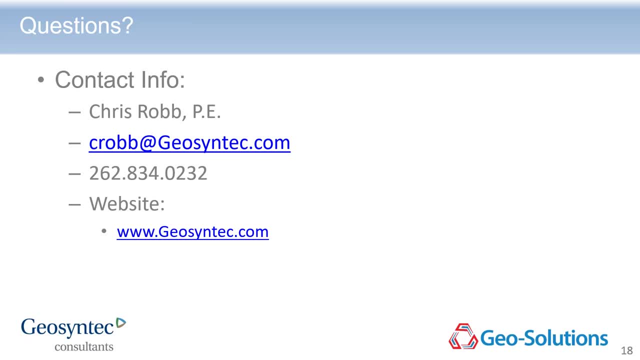 leachate it's, and then actually some of the first iss products, before they moved on to organics, were done for radioisotopes and for a metal stabilization, and so it's, it's a really interesting feature. um, and it's, it's certainly a very interesting. 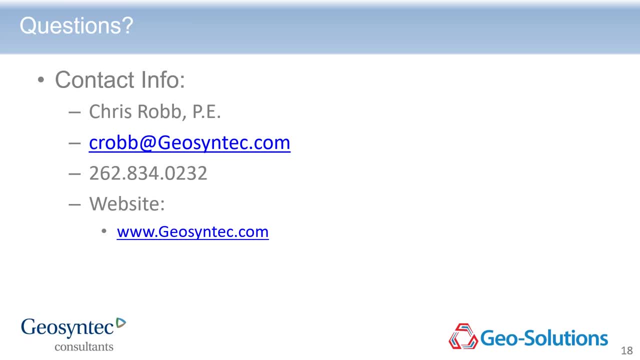 feature um, particularly things like lead um are super, super easy to stabilize. we are looking at a couple projects right now for doing this on landfills, but, um, i have, i don't have any recent experience with doing this on a landfill. um, dan, do you that those geosolutions have any recent? 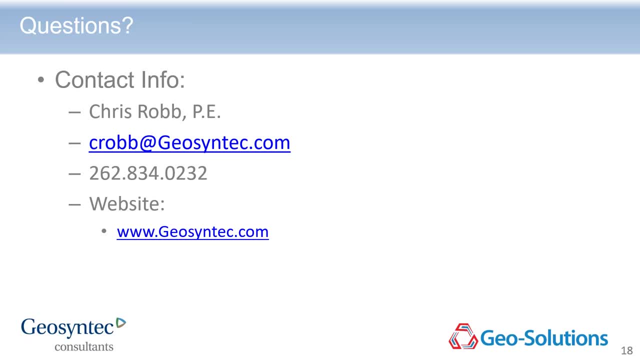 experience? yeah, so in general i would agree with what chris said. you know, technically speaking, it's to handle the contaminants that would be coming off of a landfill. My concern would be what was put into the landfill and how long has it been there and is. 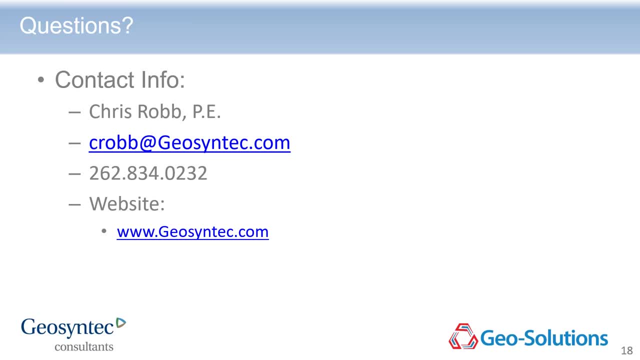 it still in its original form or some degraded form? You know there are a lot of things that are put into landfills and sometimes they're not properly shredded, so there could be situations where the materials bind up the auger or limit the distribution of the reagent, which would make it less efficient, or 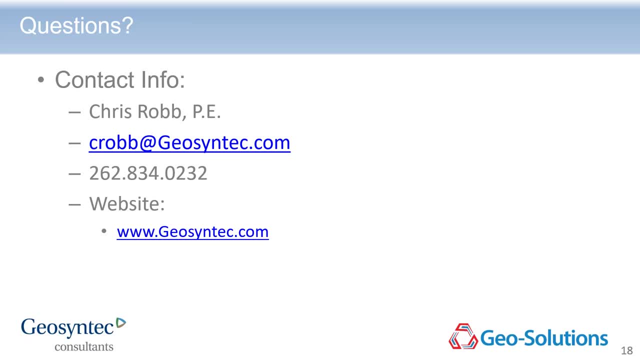 maybe impossible, and if you don't really have a good sense of what the makeup of the waste is and what state of degradation it's in, it could present considerable risk in terms of problems when you take it to the field. Okay, all right. so, since Dan is on, there was a question and actually I had one too. 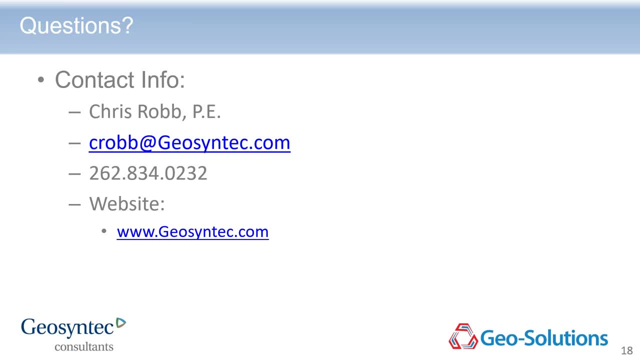 about you mentioned using blasphemy slag and wondering if you could talk a little bit more about what you're doing with the slag in soil mixing. First of all, from what type of manufacturing process? but also, or is that steel? and- and is there a reference, do you have some sort of? 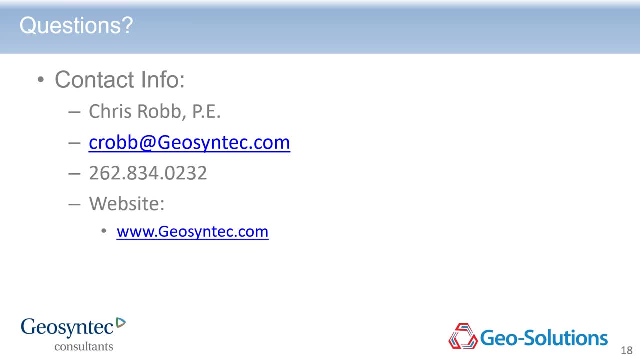 reference you could give people for how it's beneficial and documentation Sure. so there's lots of references for the use of slag in soil mixing applications and just in theory. you know, in a lot of places slag reuse is considered beneficial for sustainability objectives in some cases. 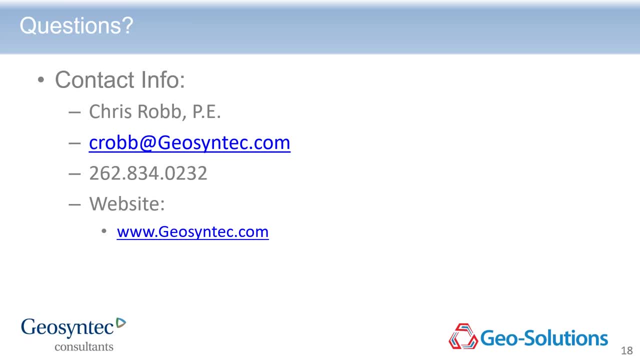 it provides a cost benefit, which is the main driving reason why slag was used in soil mixing applications in the first place. but there are also technical benefits for using slag in certain chemical conditions or soil types, like soils with or high organic contents. and then the other thing is: is that the slag 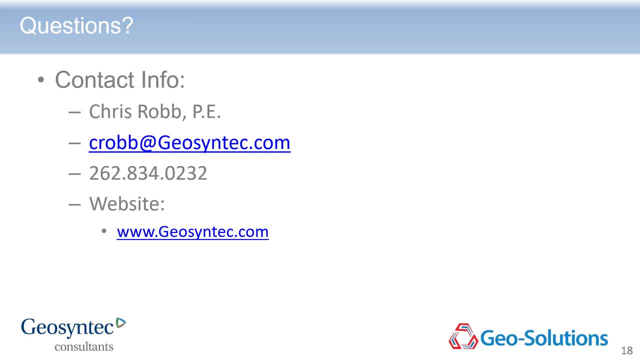 particles are finer than the Portland cement particles and over the long term, mixtures containing slag tend to have better hydraulic conductivity, ie lower and higher strength. so there are technical benefits to it as well. but yeah, we can certainly provide some some reference papers and case study examples. 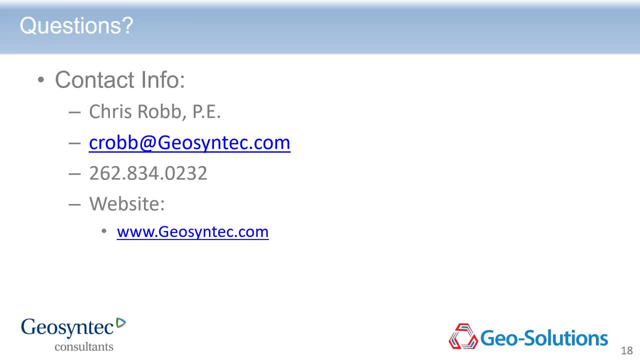 of where slag was used in combination with cement. Okay, yes, so maybe, or if you, if there's any reference studies that academics have done or something and that you could put, maybe put them in the slides so that when we post the final presentation, some references could be in there. 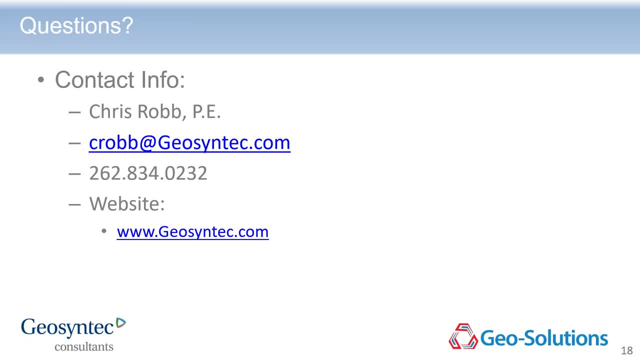 Sure, Jennifer. Okay, we have another question, a more technical one, and then I'll ask one more after that. So can soil mixing be effective in poorly permeable, filthy clay soil? that does have some moisture, but there's just. you know, when you have a well, the recharge is very 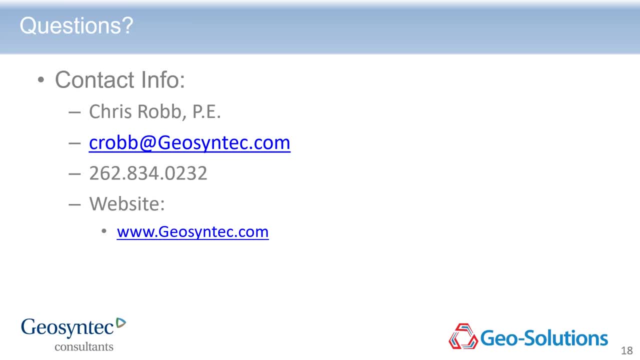 poor. Yeah, I can answer this and I'm sure Chris and Darren would probably have opinions as well. But you know, we've applied soil mixing in very tight soils, fat clays, tight silts, dense clays, so it's certainly applicable. it's just back to Chris's point. there's 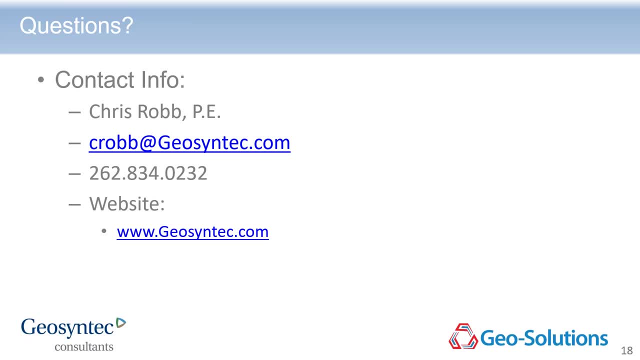 considerations there. You know it may have a high moisture content but most of that moisture may not be available for the hydration reaction so it may require additional mixing energy or additional water added with the grout to make it effective. But I think the greatest benefit of soil mixing in that sort of soil type relative to another. 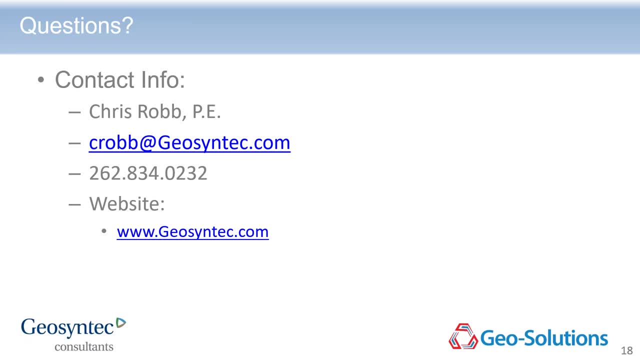 technique like direct injection is, you can absolutely get good distribution of your reagent throughout the soil matrix, almost independent of what the soil matrix is, as long as it's properly designed and you give all the proper consideration for that situation during the treatability study and in the pre-design. 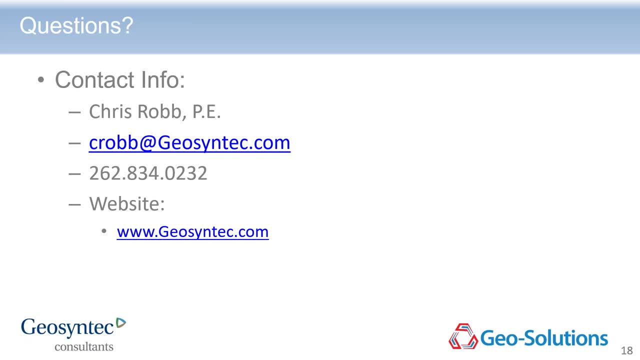 Okay, actually there's two more questions, since we're taking a break here. How about pH issues with when you put cement in, when you're adding cement into the soil? Yeah, If I could, Let me tackle this one, This question, and the previous question I can actually even better address in the case. 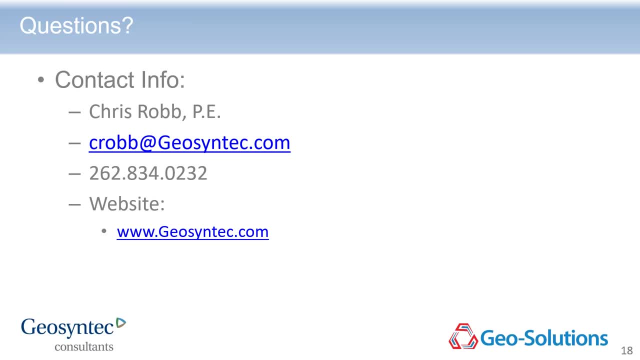 study that's going to follow these two questions. So I find that I have found that over a wide range of pHs you can successfully treat the soils and, in fact, this next case study, we had an acid spill of about 5,000 gallons. 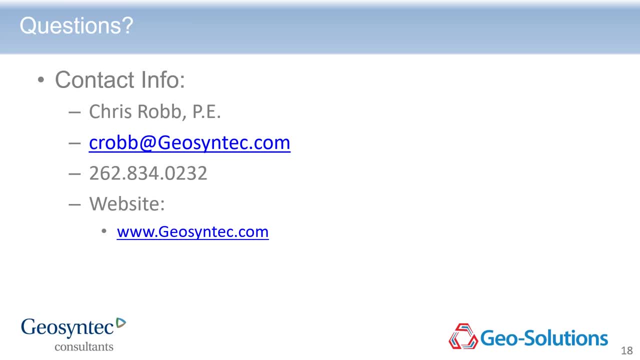 of acid or acidic material that had a pH of less than two, and it still did not interfere with our ability to do so. the cement chemistry takes over even in a very, very low pH environment. One area where it could get challenging, though, is if you're dealing with acid tar lagoons. 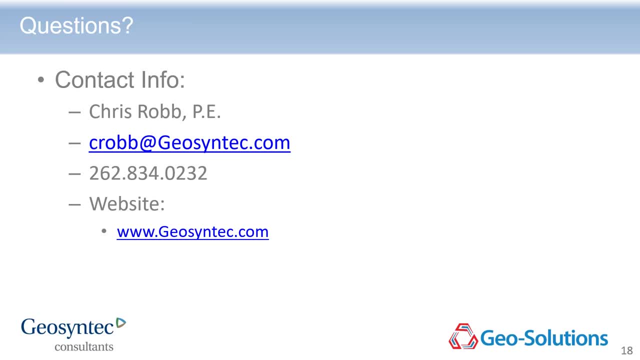 and acid sludges. but, Dan and Darren, I think you guys have some experience with finding those types of in those types of environments as well, correct, Yeah, So to Chris's point: you can come up with ways to deal with different pH conditions. 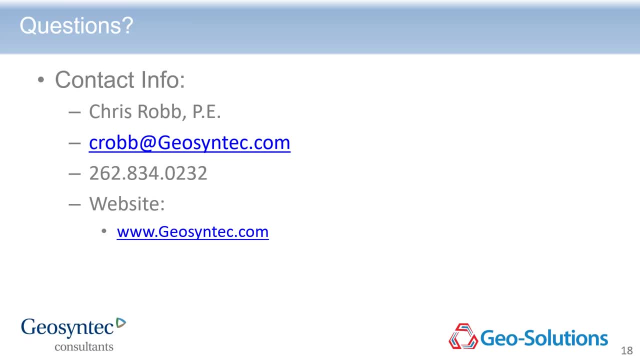 That's also going to play into the discussion about how the material is behaving in the short and long term through the leaching. Obviously different pHs are going to leach things at different levels and cause changes in how the material interacts with the groundwater over the long term. 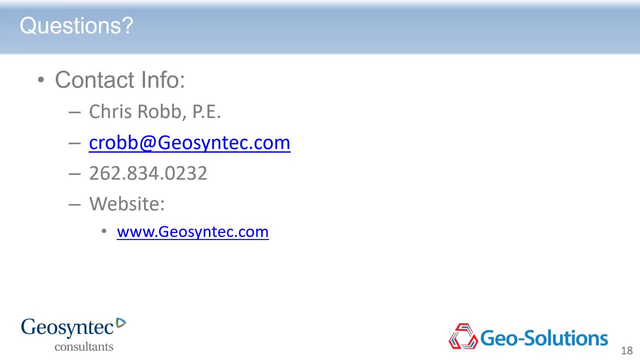 But yes, there's typically ways to design around those sort of things And we have, And we have applied soil mixing in both very acidic and basic conditions. And does the cement itself affect the pH of the existing conditions, Like, does it raise or lower, whatever it would what it normally is? 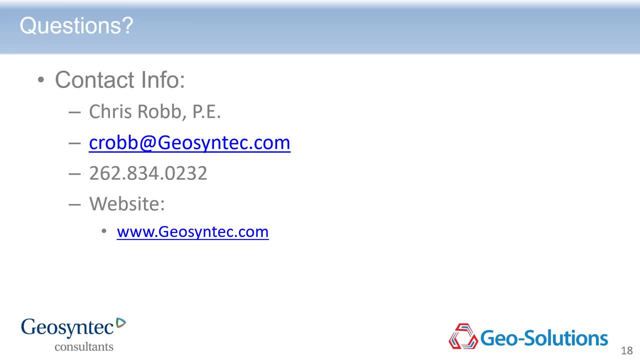 Yeah, Yeah, I mean. cement has a pH of 11 or 12, and so a lot of times when you mix it with the soils, even at low concentrations, it can raise the pH. All right, Thank you, Thank you. 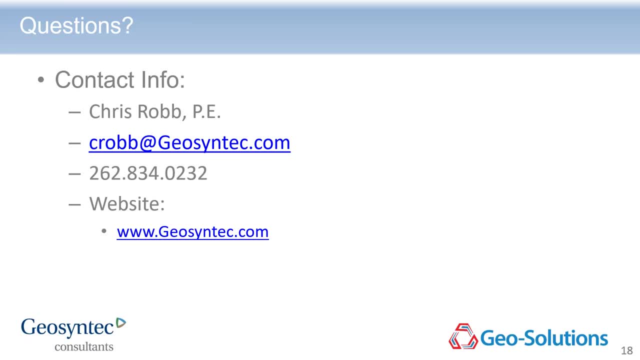 All right, So Okay, So that may be a benefit. In other cases you may have to do some sort of perimeter control to deal with that issue. Chris, I don't know if you can speak to that. Okay, Oh, go ahead. 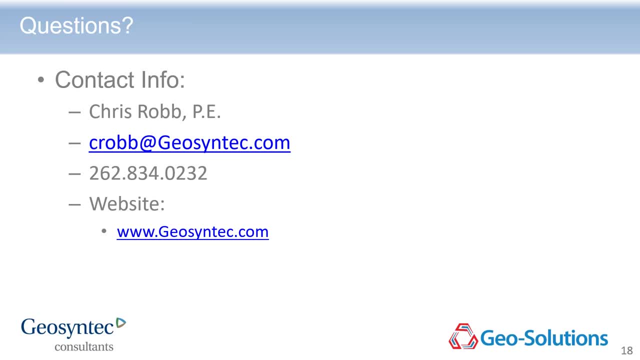 Yeah, It's going to be. you're going to create an out-the-line environment around where we do ISS treatment And the conditions will stay out-the-line until most of the cement hydration reactions are complete, And then the and, then and the environment finalizes. 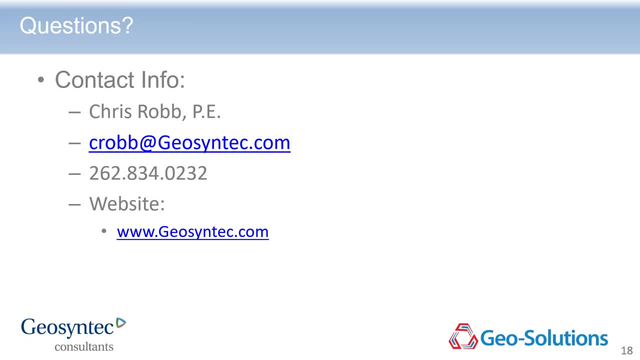 And then the environment finds its new buffering capacity, or it just buffers out the pH over time. So Okay, So some folks are hoping that there will be some more discussion about some of the treatment methods that you can use: the injection of the reagents and that sort of thing. 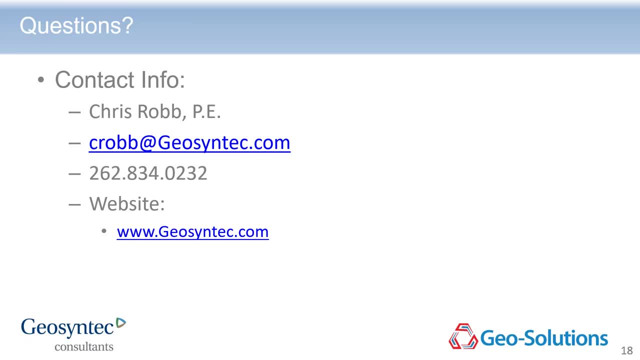 So hopefully the case study will touch on some of that. It gives some practical advice And then also wondering about state regulators and ongoing O&M to make sure that these things remain protective over time. If anybody can talk about that now, or do you want to wait until the end? 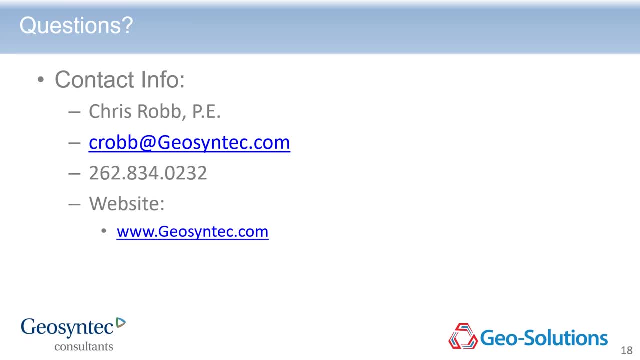 I think that one's you, Chris, if you want to talk about. I mean, in my opinion, it needs to be assessed at a site level. There's a lot of things you know. going back to Chris's slide with the little ITRC: 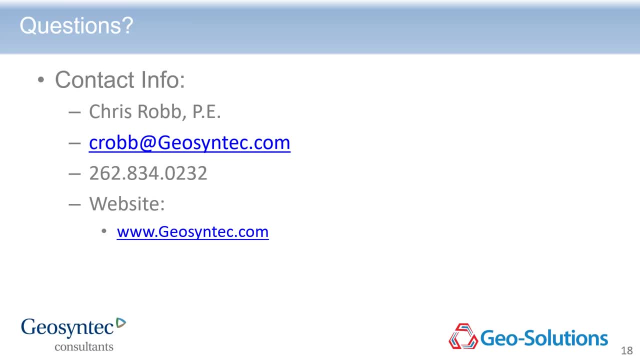 figure that shows all the various factors that might be impacting the ISS monolith over time. So definitely a site-specific consideration. but there have been a lot of case studies where this was implemented a long time ago And long-term monitoring has showed that it behaves as intended over the long, the long-term. 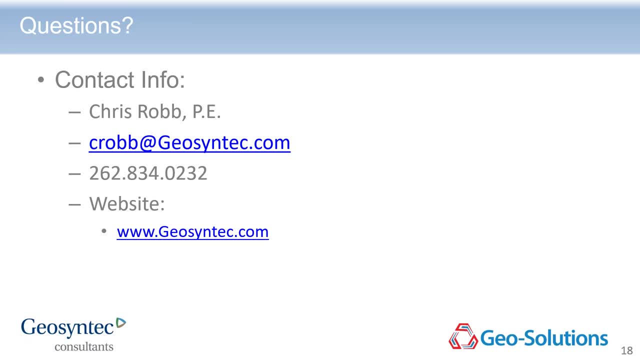 And it's. I would say that probably the gold standard for a case study is the, you know, the Columbus Georgia Manufactured Gas Plant site which was completed in the early 90s, And if you're interested in that you can go out and just type that in and type in EPRI. 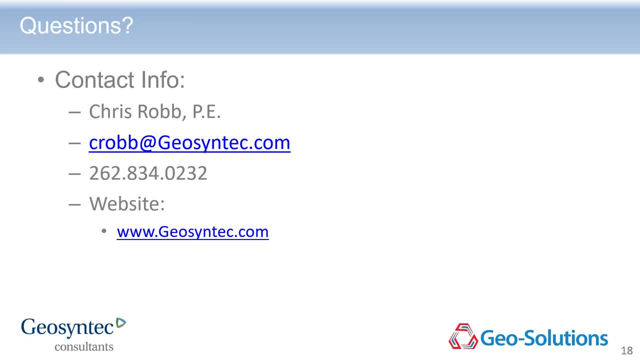 That's the acronym for the Electric Power Research Institute. They did a 10-year assessment after that site was completed. That's a document you do not have to pay for. It's free, And you can read about how they went about assessing the ISS on that site 10 years later. 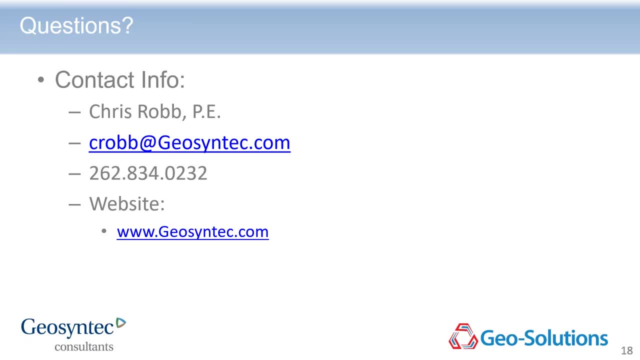 So that's a good thing. It's an excellent case study and it's still holding up to this day, So that's going on 30 years. That's probably one of the older examples in the United States on a, especially on an. 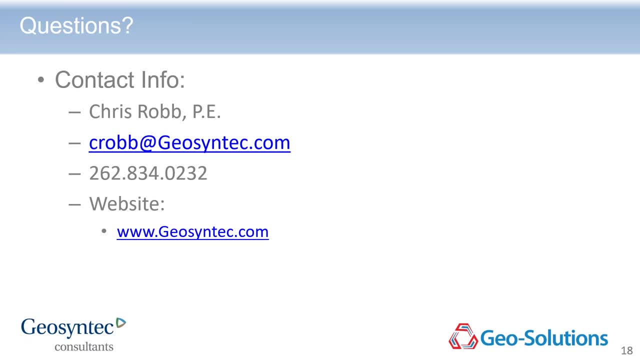 MGP site. As far as long-term monitoring also, what we're seeing more and more of is, you know, really setting up the groundwater monitoring network to monitor the efficacy of the ISS Over time, And we're finding more and more clients and owners are asking us to use groundwater a. 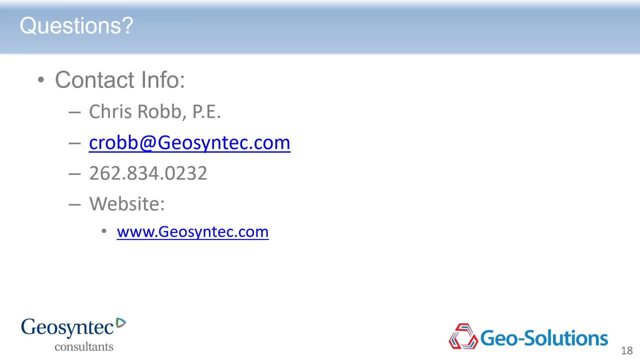 groundwater model to do that and to help design, in collaboration with regulators, what the groundwater monitoring well network looks like. One of the more recent examples I was involved with was a site down in Florida and we found almost an immediate benefit to the long-term monitoring network. 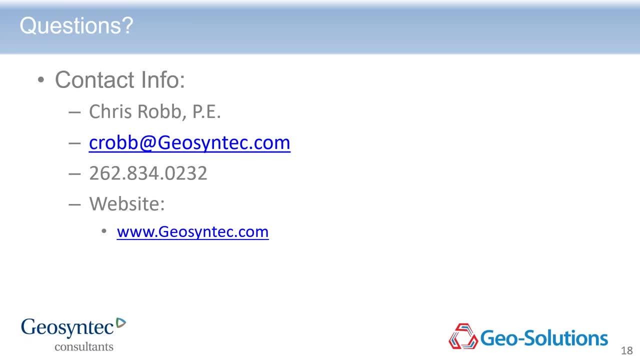 And that's a good thing. That's a good thing, That's a good benefit to the long-term groundwater concentration in most wells directly adjacent to the ISS, And then with some of the more areas we thought would be problematic, what we're finding is: 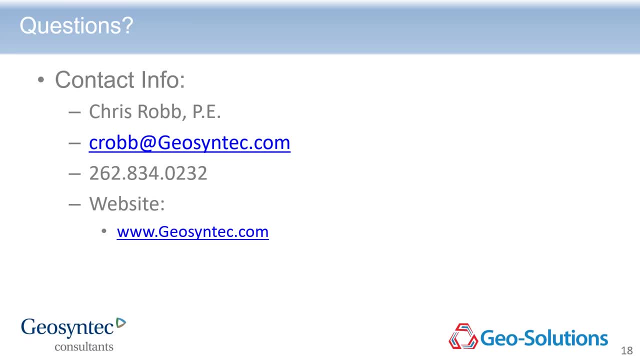 really establishing conditions for a stable and or receding plume, So establishing conditions that will eventually- how shall I say? provide an environment where monitoring is possible And that's really an environment where monitored natural attenuation can take place over time. So 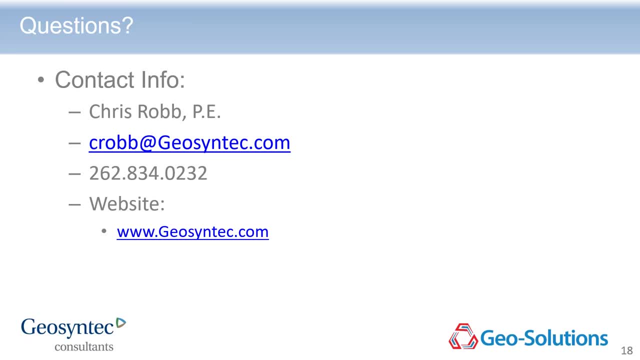 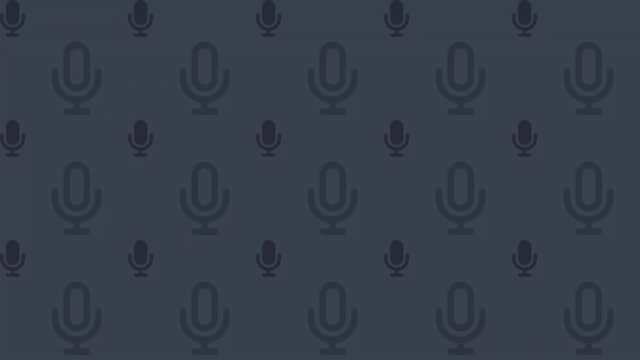 But we can talk more about that, I think, in the case studies. Great, So let's move on. until we have enough time for that, I'll make Darren the presenter. I'm going to- if you could keep me as presenter, Jennifer, I'm going to do this. 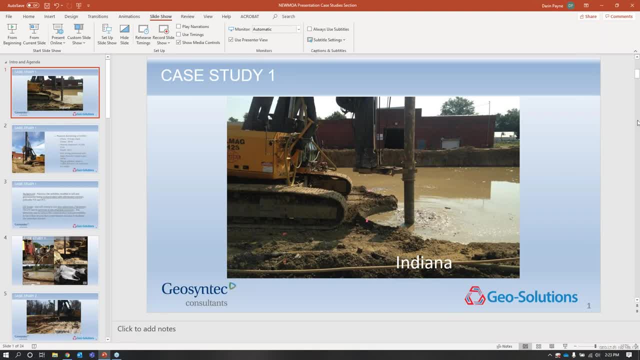 Who's doing that? No, I want to know. Sorry, Yeah, If you could keep me as presenter, Jennifer, I'm going to do this. You can just make me the presenter. This is Chris, Chris, Okay, Sorry. 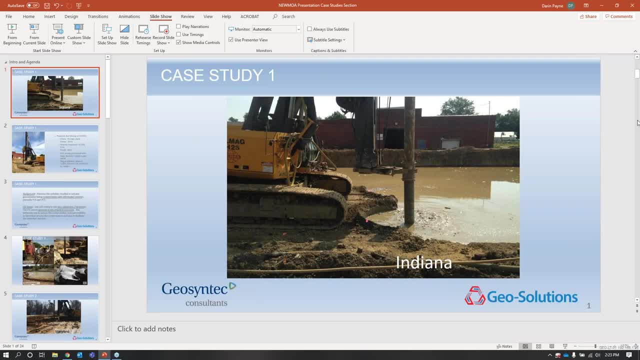 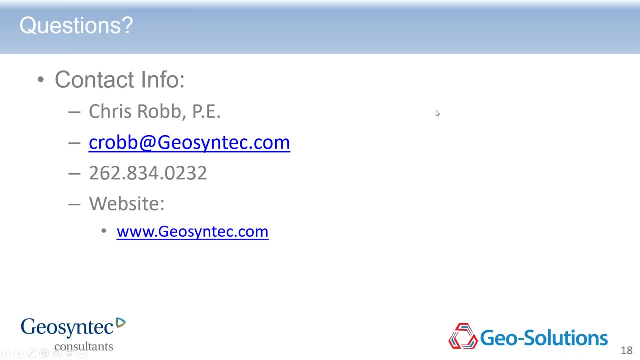 Yeah, Chris, I have one more. No, that's okay. I have a case study. Sorry about that. You have a case? Oh, okay. And then Darren? Okay, Well, let's get going then, Okay, Good. 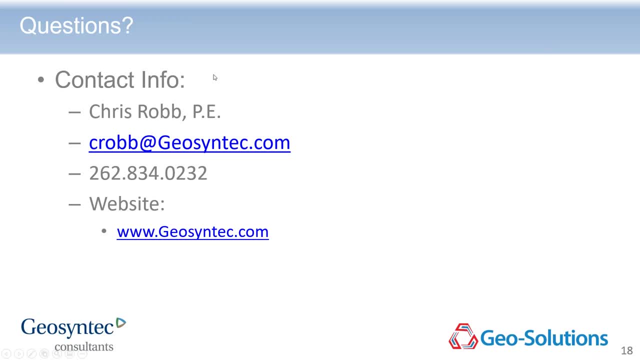 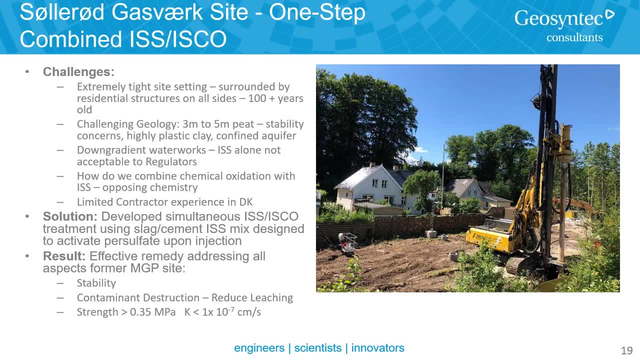 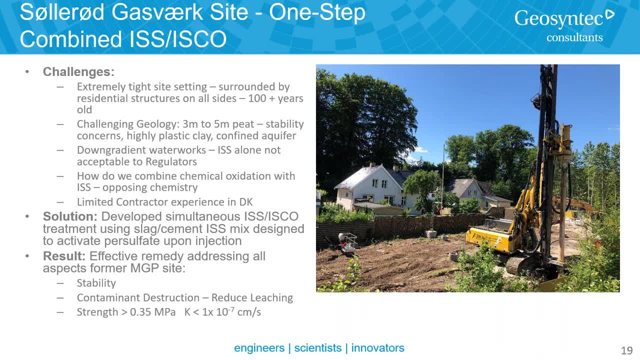 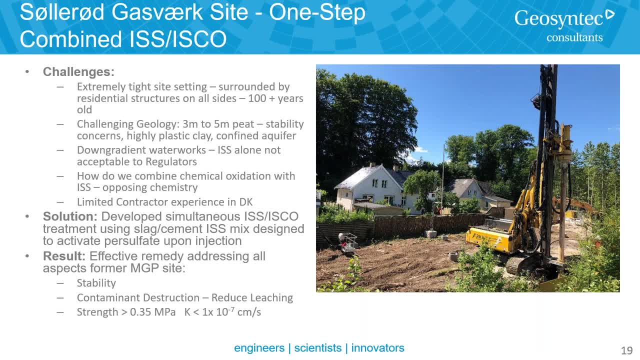 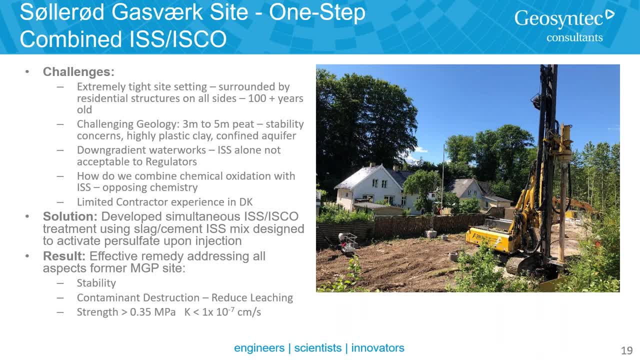 This is the SolarARG-2.. This is the SolarARG-2.. It had very challenging geology, So the first three to five meters were peat, which presented significant stability concerns, But really where we wanted to do the treatment was in a highly plastic clay that was confining in aquifer. 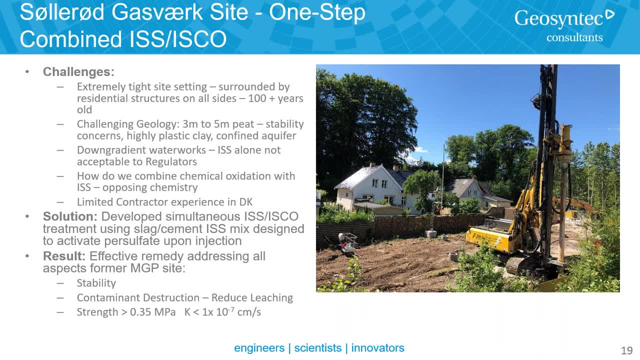 So this clay was extremely plastic and extremely fat and very, very difficult to mix And then immediate downgradient. there was a waterworks. So ISS alone wasn't acceptable to the capital region of Denmark, So we proposed to do chemical oxidation in direct combination with ISS. 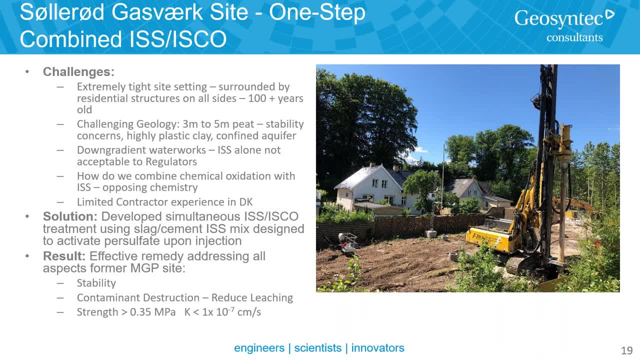 And the thing about chemical oxidation is it's an acidic reaction often, And what we used instead was a base-activated persulfate to kind of overcome some of that opposing chemistry. So our solution is we developed a simultaneous ISS, an in-situ chemical oxidation treatment, using slag cement as the base activator for the persulfate upon injection. 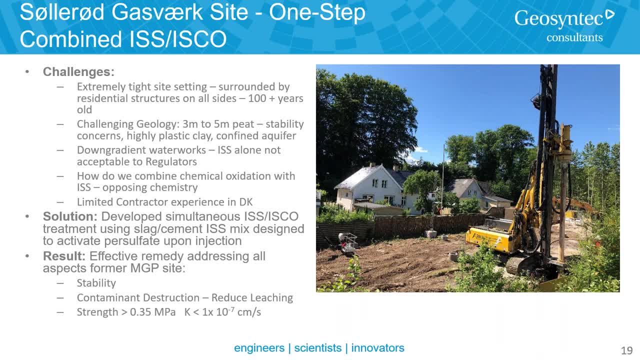 And the result was is: we did effectively and were effectively able to treat all of the soils on site. We addressed stability, We had contaminant destruction, We were able to reduce leaching And we typically had a strength greater than 50 PSI, which is 0.35 megapixels. 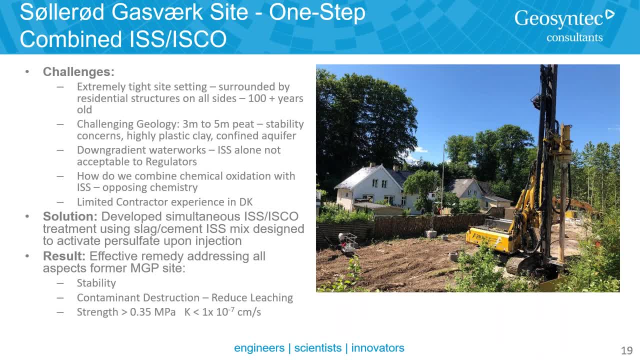 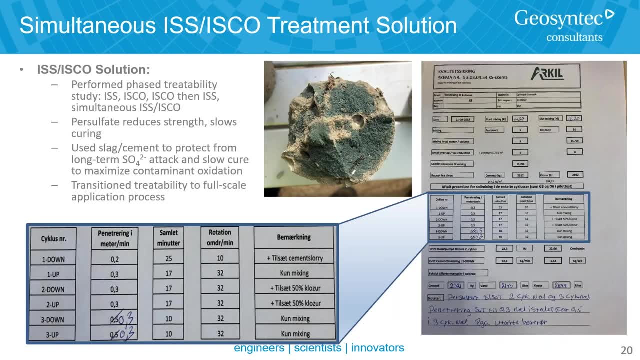 And reduced hydraulic conductivity, typically to less than 1 times 10, to the minus 7 centimeters per second. So for the solution, we performed a phase treatability study. We looked at ISS, ISCO, ISCO, followed by ISS and simultaneous 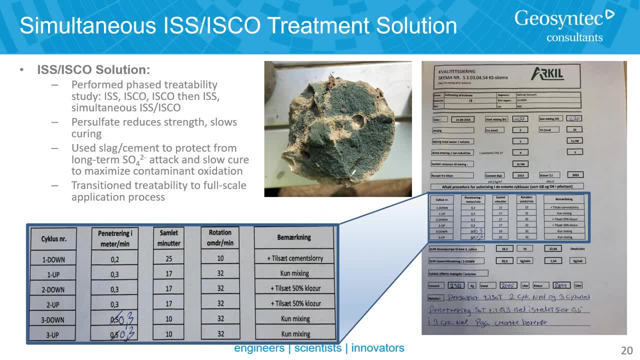 Because we found that persulfate actually can really reduce the strength and slow down the curing of the cement. However, by combining it with slag cement, we were able to protect and inhibit some of that slowdown from long-term sulfate attack And we were able to maximize contaminant oxidation. 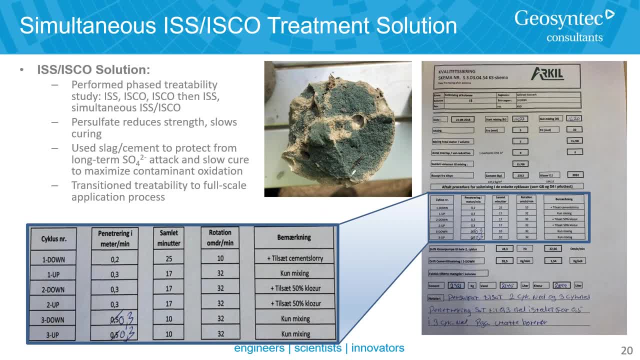 But one of the features and things that I wanted to show on this slide is what we found in these highly plastic clays, And that's what's shown on this drilling log here. is it really came down to all about delivering mixing energy? So, because we have such a tight geologic structure, 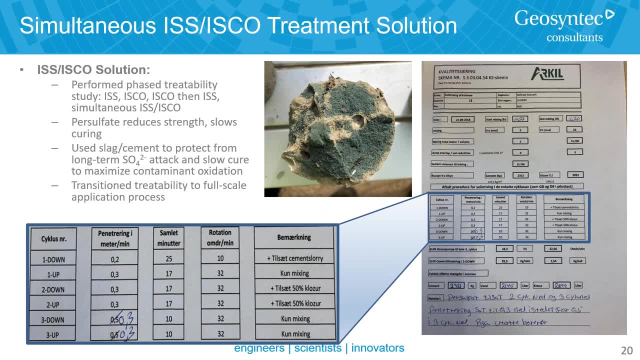 we had to work with the contractor to really slow down their penetration rate to the extent that they could- And this so this is this here is shown, as this is 20 centimeters per minute, or 0.2 meters per minute- And then increase the rotations to the extent, practical slowing the rotations the way down. 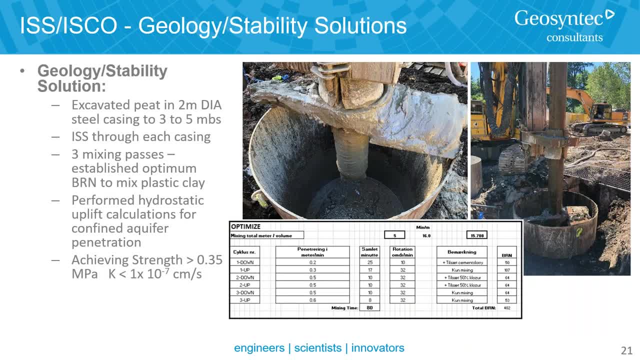 But it was all about delivering adequate mixing energy, And that's really what we found, And that's really what is shown here too, And we had to work with them to optimize that, And we then created a qualitative metric called the blade rotation number. 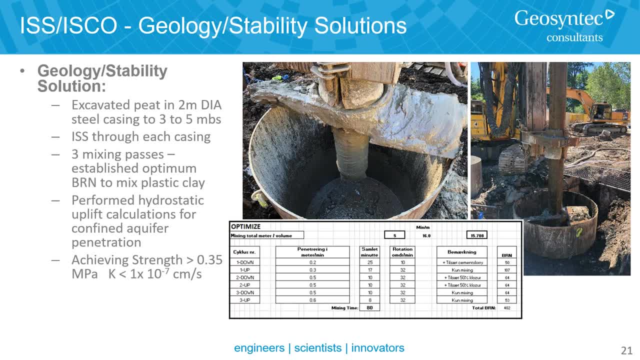 which is used on a lot of geotechnical sites in the United States to ensure we were delivering enough mixing energy and really mixing this clay. So this is just some of the other features of the site, But really what it came down to is three mixing passes to establish that optimum blade rotation number. 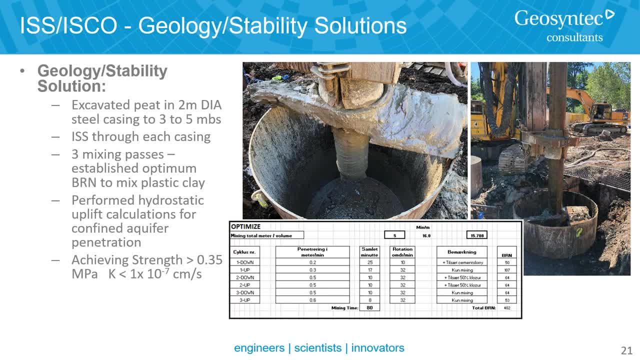 And we had to mix the plastic clay. And then one other unique characteristic of this site is we had to perform hydrostatic uplift calculations Because the aquifer was confined. we were worried that we'd actually have groundwater expressing up through the ISS treatment and at the surface. 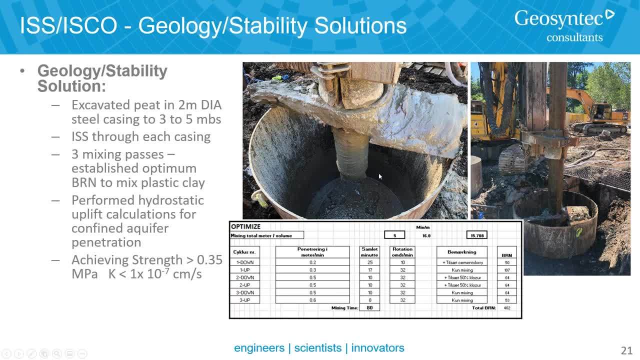 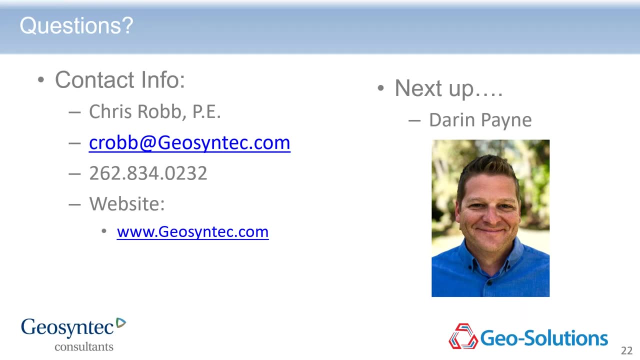 So we had to also design this grout with a little heavier density to make sure that it had enough that its unit weight was greater than water And that we would not see water And that we would not see water coming up through the ISS treatment. So I'm going to turn it over to Darren now, and 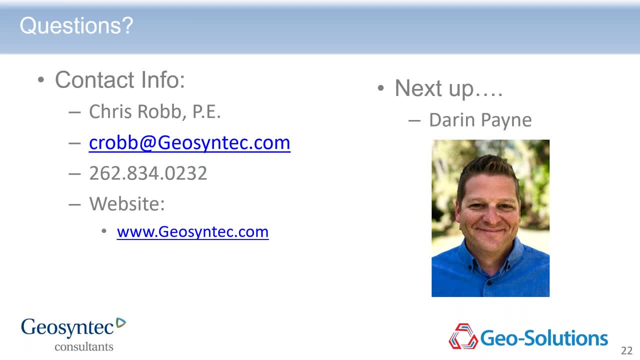 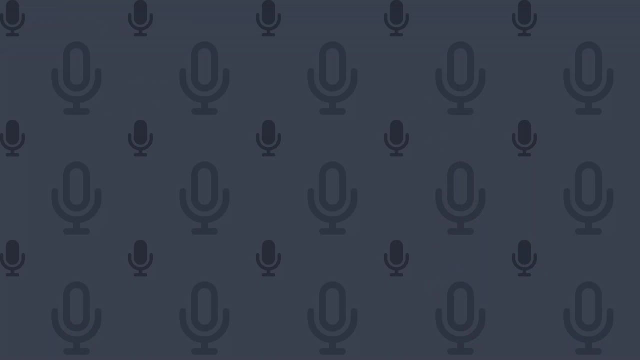 Darren's going to jump into the next case studies and then we'll pick up questions on these case studies after Darren's finished. So over to you. So now I should present her right. Sorry, Jennifer, It was a feature we added. Thank you, Great. 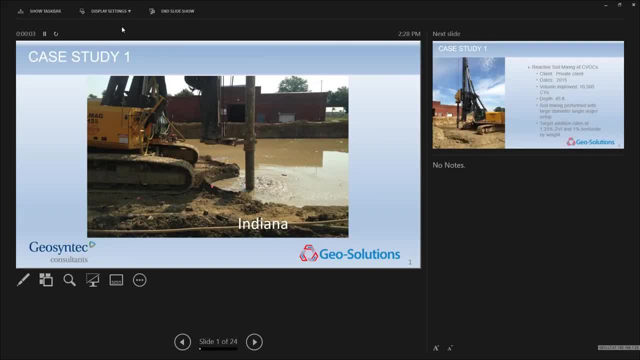 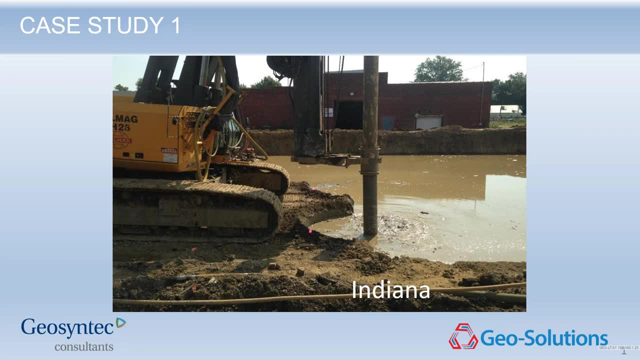 Yes, Okay, Is that up? Yeah, go ahead, Okay. So now we're going to talk about some of the implementation of these techniques and reagents and some real-world experience. So the first site we're going to talk about was in Indiana. It was a soil. 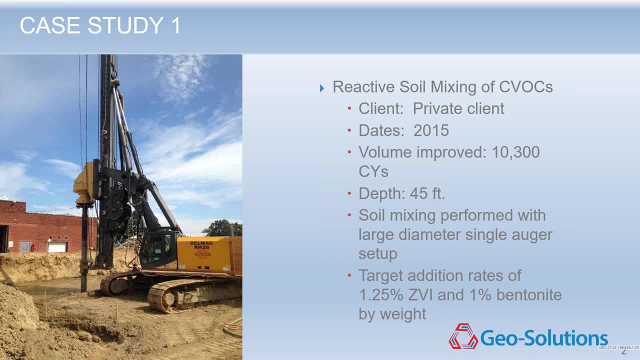 mixing for remediation of CVOCs. The work was performed back in 2015 for a private client. The total volume tree was about 10,300 cubic yards, with treatment down to a maximum of about 45 feet. The soil mixing was performed on site with a 10-foot diameter auger mounted on a track. 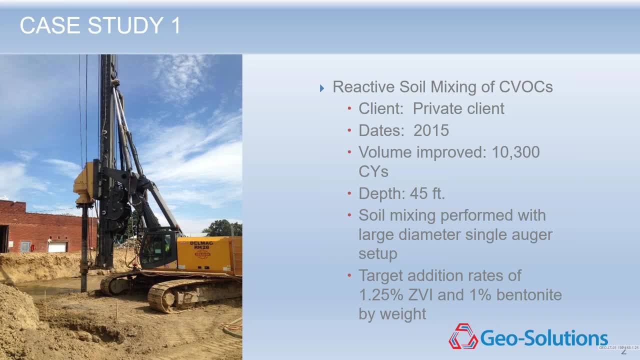 mounted drill rig And based on the results of the pre-construction bench scale, including some column tests, the amount of ZBI needed to achieve suitable contaminant mass destruction was 1.25 percent by weight. Bentonite was added at 1 percent by soil weight to reduce the permeability of the contaminated. 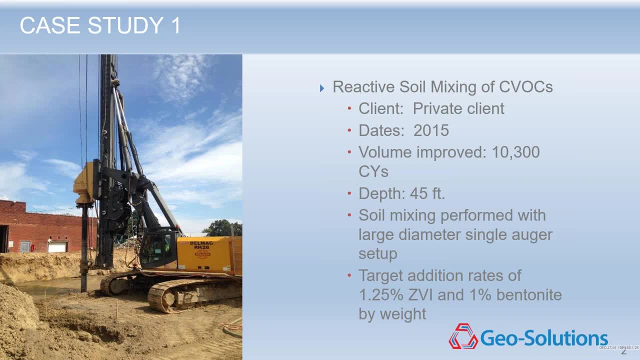 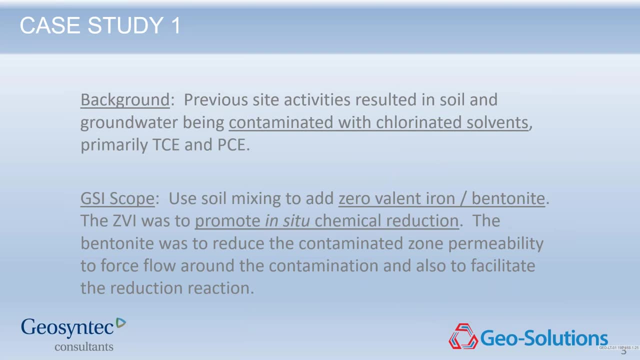 zone and also act as a delivery method for the ZBI. So previous site activities and activities of the adjacent sites resulted in subsurface contamination with chlorinated solvents, primarily TCE GeoSolutions. consulted with the designer for about two years prior to the field work. 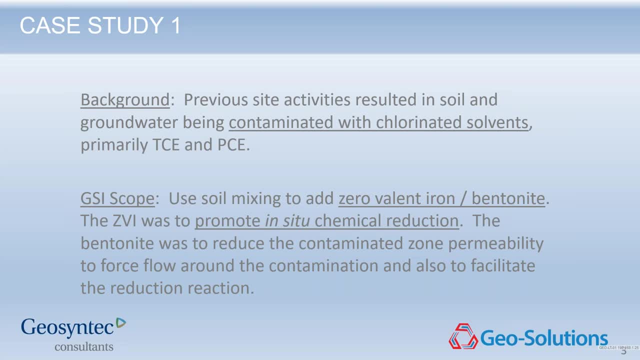 working through logistics and bench scale work with them. During the consulting period, a reactive soil mixing approach with ZBI and Bentonite clay was developed to promote an in situ reduction reaction of the chlorinated solvent source plume and also reduce the permeability of the contaminated area. 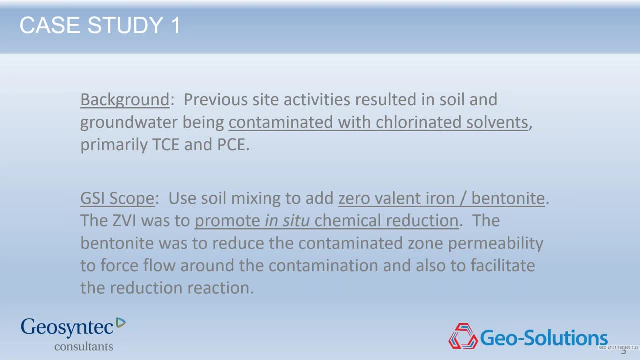 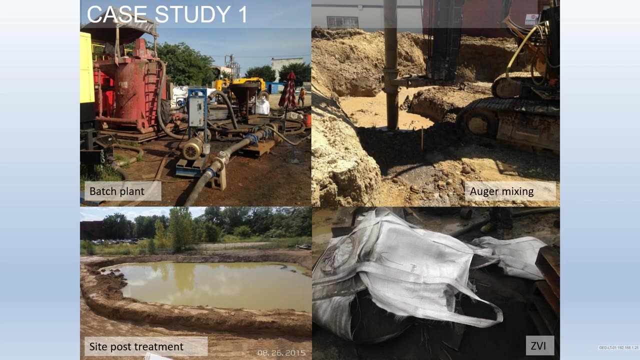 To prevent contamination, Thank you, And also to help reduce the contamination of additional groundwater flowing through. So here's some photos of the work being performed. In the top right you can see the auger actually mixing the soil with the Bentonite and ZBI. 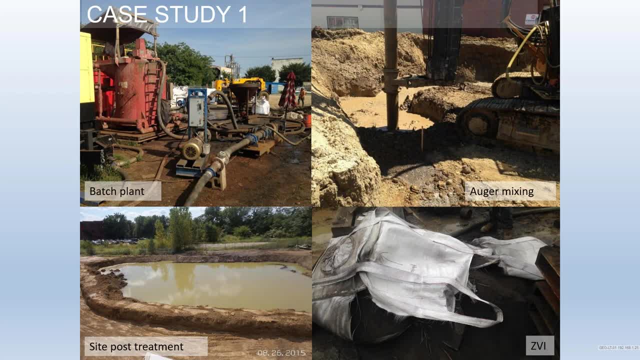 slurry. The bottom right shows the Super Sacks that the ZBI comes in and it's typically loaded into the mixers from those Super Sacks And the bottom left shows the treatment area. So one thing to note with a lot of the reduction reactions is that it leaves a somewhat fluid 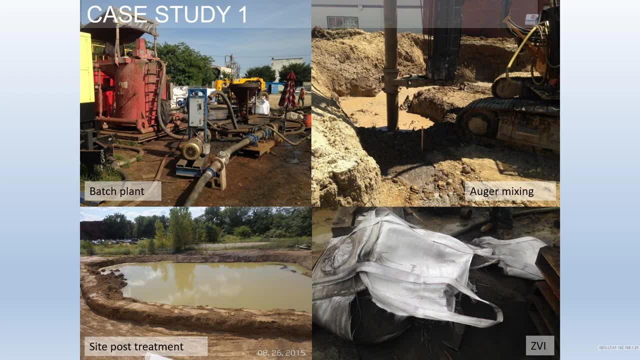 area, as where the oxidant reactions- a lot of those- can be used with a post-cementitious addition. The reduction reactions would be hindered by the pH of the cement and those reactions can take quite some time to destroy the contaminants, So it may be months or years before the cement could be added. 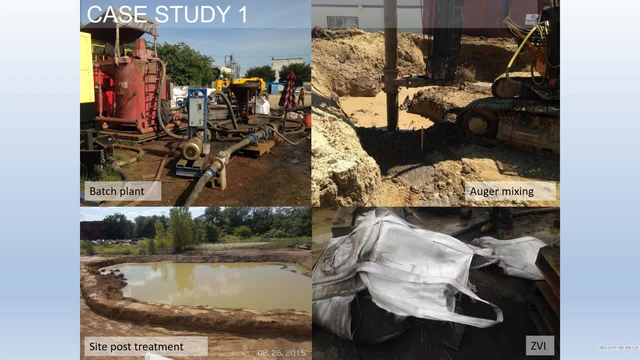 So these areas need time to consolidate and some of the water to evaporate off and go away. A lot of it is stormwater in that particular picture Because we've reduced the pressure, We've reduced the permeability of the mass. The top left is a picture of the batch plant which you can tell it kind of has a brownish. 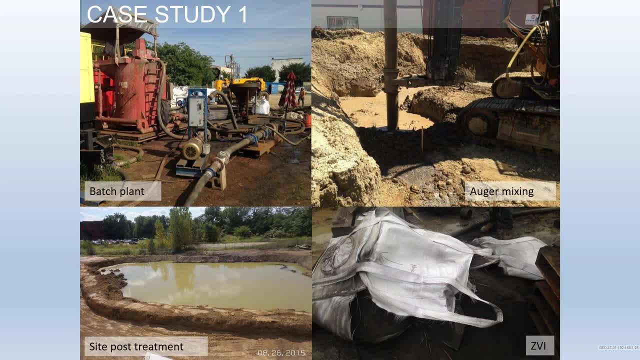 hue. that has a lot to do with the zero-valent iron which tends to create kind of a layer of rust on some of the plant equipment. It can be a little bit challenging to work with if you haven't done it before. If larger structures are planned for the site or desired, 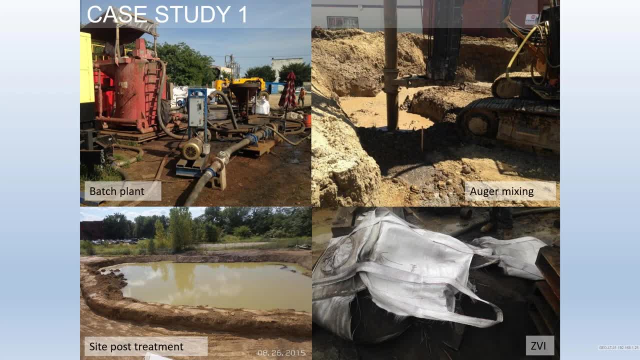 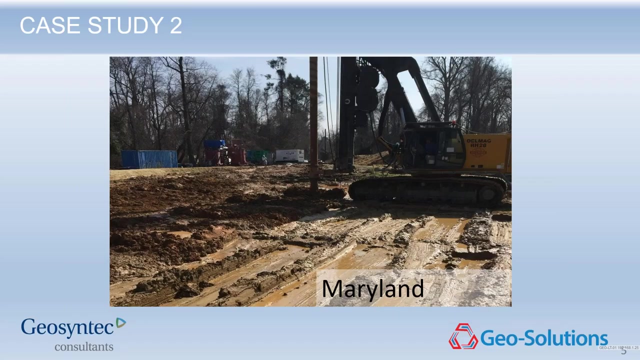 A ground improvement could be done later after these projects are completed. Where cement can't be added, you could improve the surface with a cap and cover system or other. you know, foundation improvement. Okay, So the next case study was a project in Aberdeen Maryland. 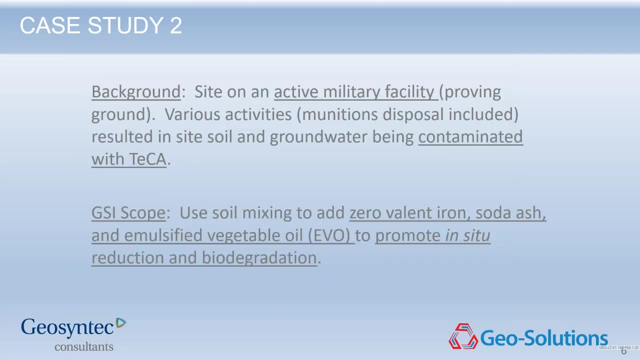 Okay, Great Thank you. The project is located at an active military facility, the Edgewood Base, which is part of the Aberdeen Proving Grounds. GSI was contracted to perform in situ chemical injection to promote chemical reduction of tetrachloroethane. 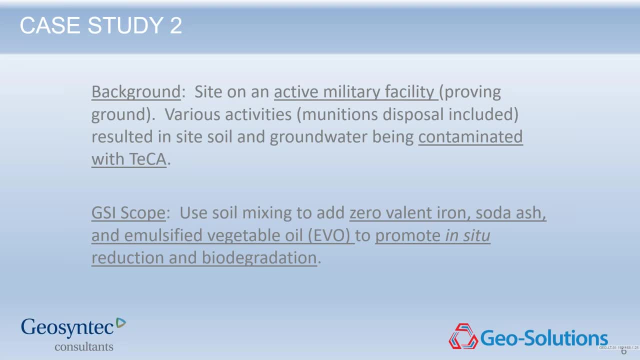 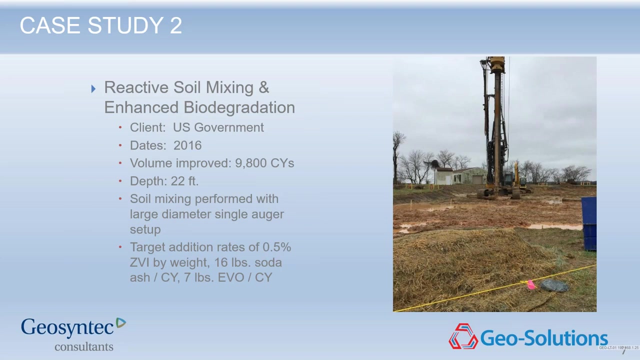 The reagents added to the site included zero-valent iron again, soda ash for pH adjustments and emulsified vegetable oil to promote bioremediation. at completion, GSI was contracted to ECC, who was directly contracted to a branch of the US government. 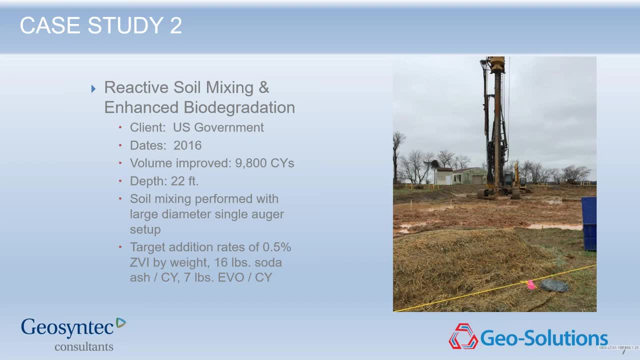 The work was completed at approximately 9,800 cubic yards to a depth of 22 feet below ground surface. The soil mixing on this project, similar to the last, was performed with a track-mounted drill rig. These drill rigs are typically European. 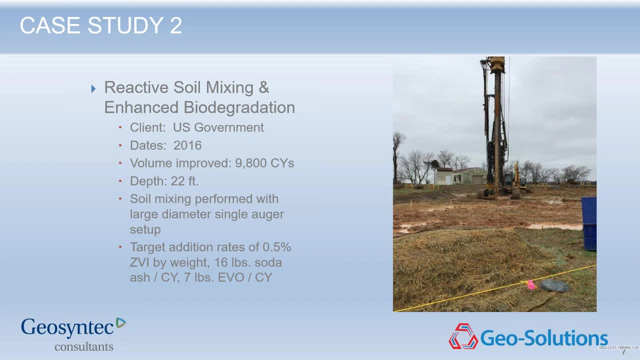 Manufactured caisson-style rigs that are modified for soil mixing. I think Chris's photo showed a different model, and some of these are all showing similar models, but they're track-mounted hydraulic drill rigs that are manufactured for that purpose. So the reagent dosages for this project were selected based on the expected contaminant. 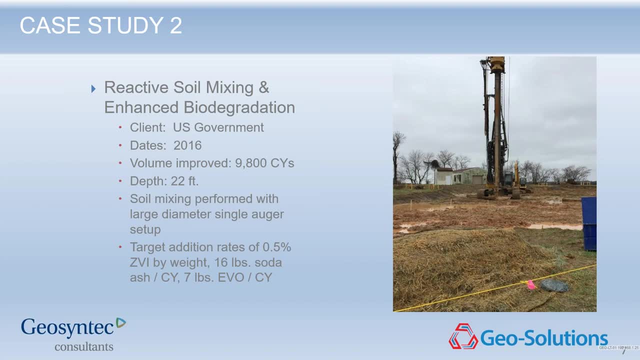 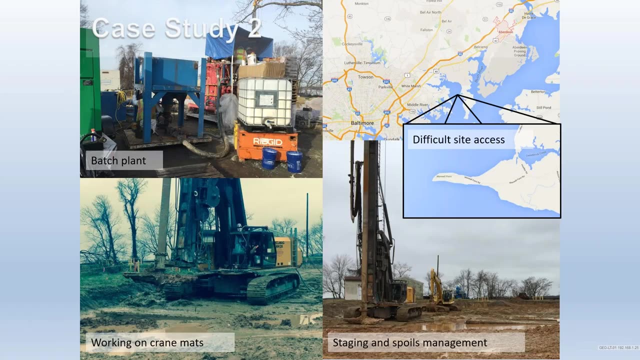 mass and the mass needed to complete the chemical reaction. So no bench scale was completed for that. Okay, So that's the process for this project. Some more photos. So one of the components of the project was that it was located at the back of an active 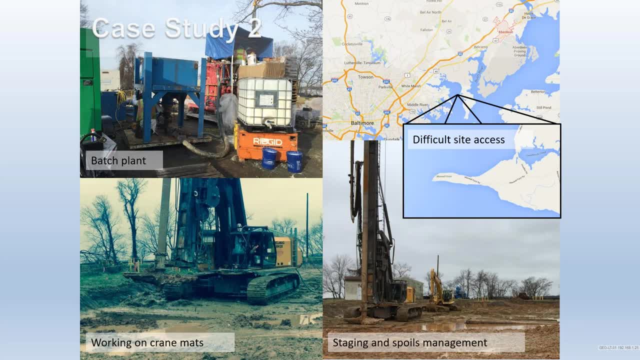 military facility, so that typically has a few of its own challenges. Employees had to be subjected to a deep background search and spent hours at the guard shack for a check-in process. When the door closed, the facility was left open for an entire week. 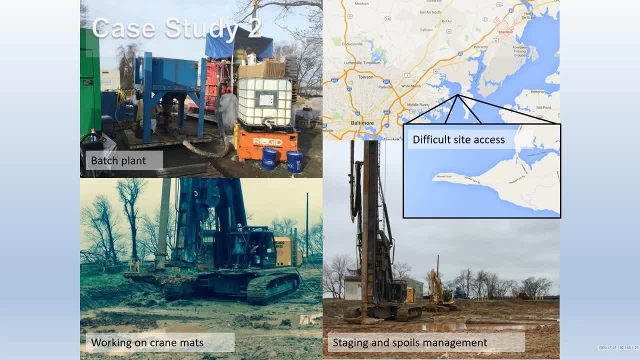 The site was a mess. The site was a mess. The area was not clean, The areas were not well-maintained, The roads and portions of this area were gravel or dirt, so deliveries were difficult. In some cases we'd have material drop outside of the entrance and a rough-drain forklift would bring each piece back individually to our work area. 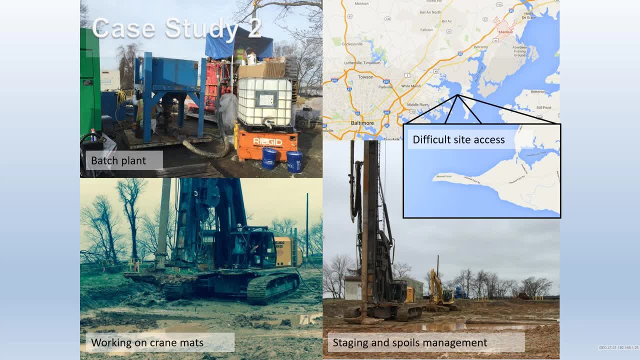 Also because of the site location on a peninsula in brackish water, the near-surface soils were deposited in a marshy condition and were almost always wet, so it left for unstable conditions to work in. So we're still working with the state to figure out how to use this. 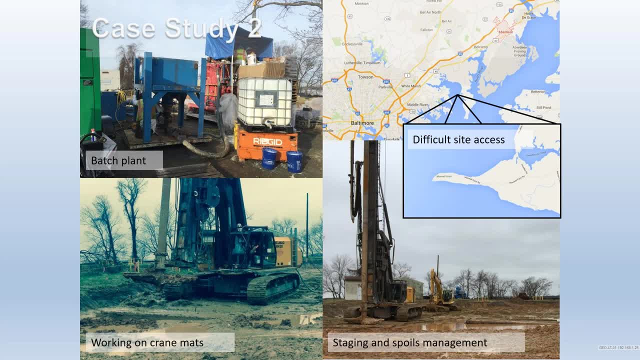 So we're still working with the state to figure out how to use this. We're still working with the state to figure out how to use this. we're almost always wet, so it left for unstable conditions to work in and required the use of crane mats, which you'll see in a lot of these photos, and 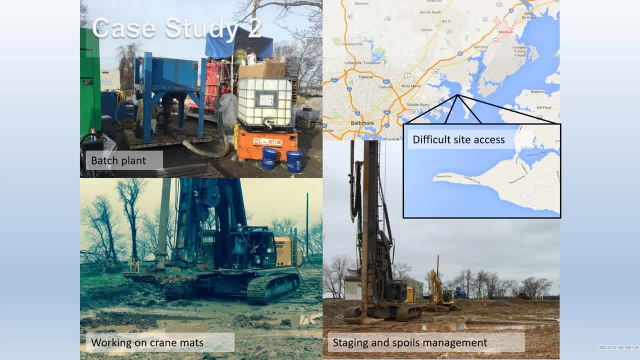 a lot of times they aren't necessary, since a lot of these rigs are heavier, let's say 200 to 300,000 pounds. so in the in the bottom right, you have the drill rig and a support excavator behind it, likely moving the mats that are kind of hard to see, but underneath 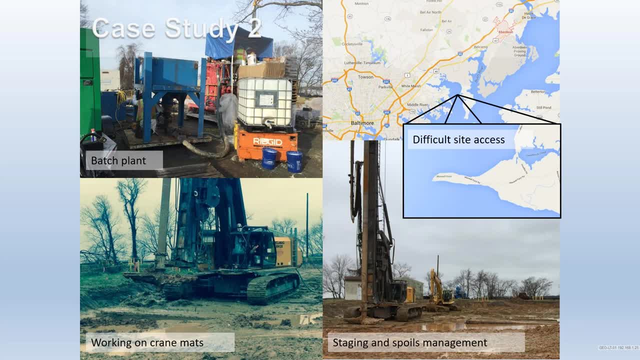 the rig. those are typically the crane mats shown in the picture, to the left as well. so those are four foot by one foot thick, by anywhere from 20 to 30 feet long. in the top left you have a portion of the batch plant which shows where 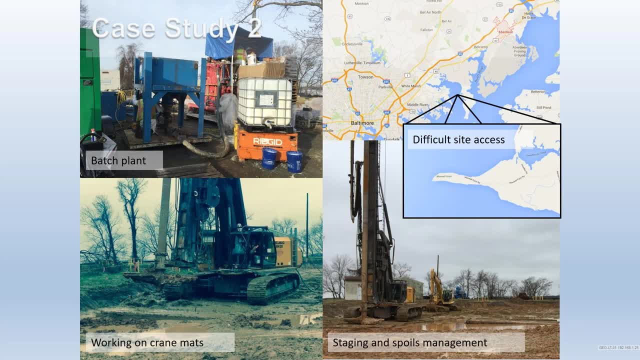 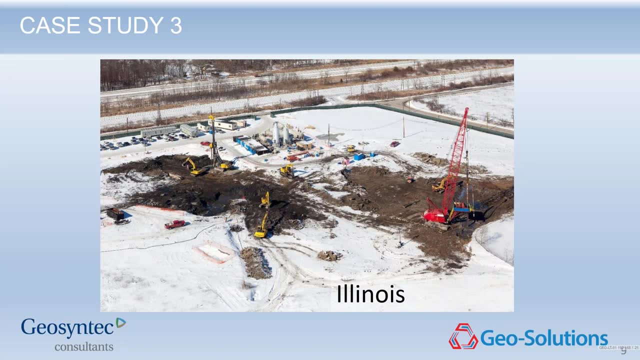 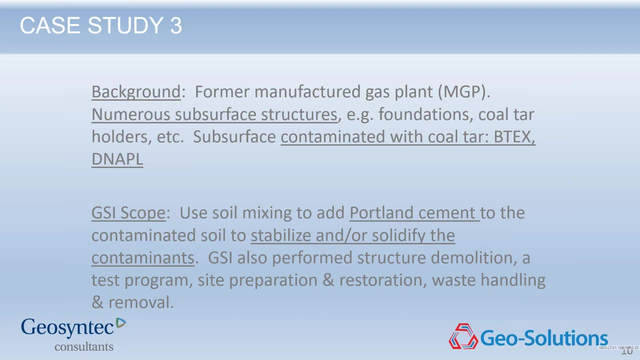 those super sacks are unloaded and some of the ancillary equipment that's being used. so the next project is in Illinois, Waukegan, Illinois. This site was in situ solidification stabilization at a MGP site, so had former manufactured gas plants impacts and, as common on most MGP sites, a lot of them. 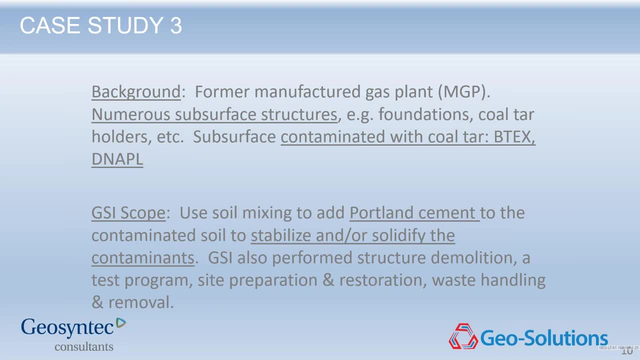 were demolished and backfilled with, with not a lot of future plans for future projects. So a lot of the subsurface is full of obstructions and structures and foundation parts and bricks, things like that. so this project included an excavation of the upper four feet to try to get a lot of that material out. some. 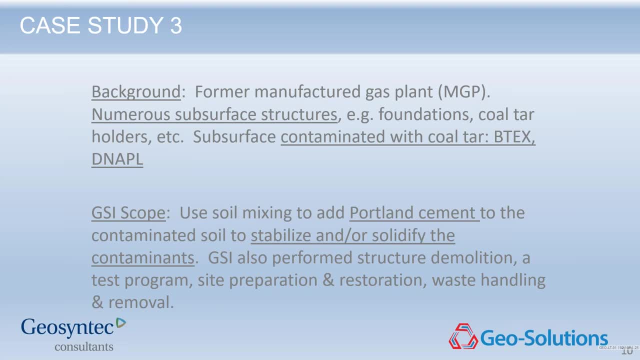 of that had to be demolished and then sized and taken off-site. so an important part of the project became management of on-site spoils and an off-site disposal to try to balance that. a lot of the spoils generated were kept on site so that clean four-foot overburden excavation. 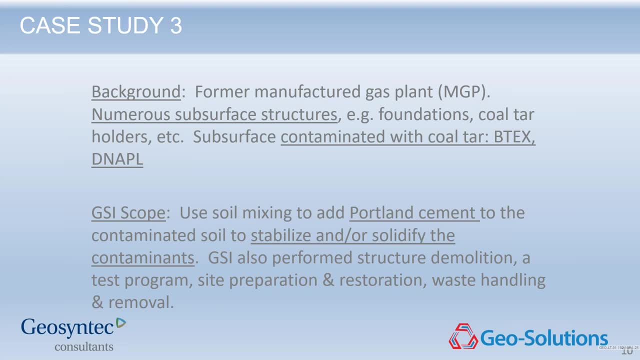 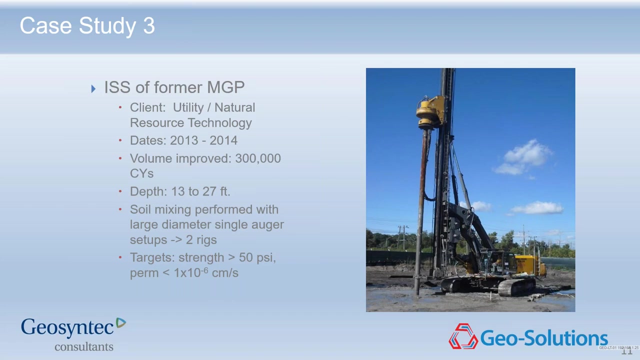 which was shipped off to off-site disposal, and a cap was designed to mound the spoils slightly up to promote overland flow and drainage. This project was somewhat of a landmark project for MGP site. It's a project that's been going on for about five years now. 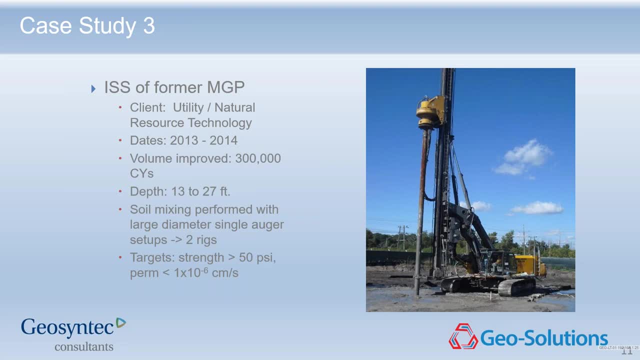 It's the largest soil mixing site in the United States. It's one of the largest, if not the largest, soil mixing at an MGP site in the US. I don't believe that's changed since this was implemented. It was a utility owned site in that area. 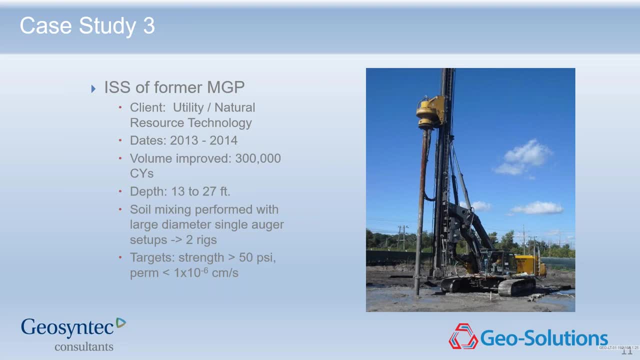 And the improvement injectors were fairly typical for MGP sites and a lot of our sites in general. We had about 50 PSI, one times 10 to the minus six. So this site did include a slag, blast, furnace, slag and cement mixture. 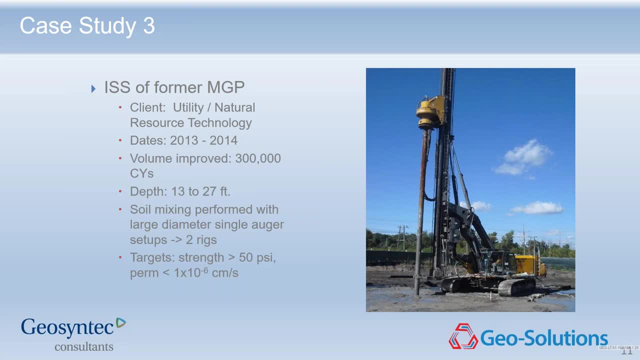 It was about 75% blast furnace slag and 25% Portland cement And that was the ratios within the mix and the addition rate was at about 12% total. So that was a lot of work. The slag was selected to help reduce permeability as well as aid in the long-term generation. 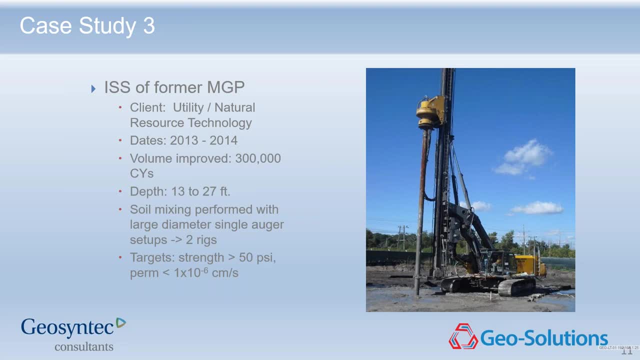 of strength, But it also because they're sandy soils. bentonite could have been used, and is often used, But because it was sensitive to swell, which bentonite can sometimes create, more of slag was selected to try to reduce the impact of that swell. 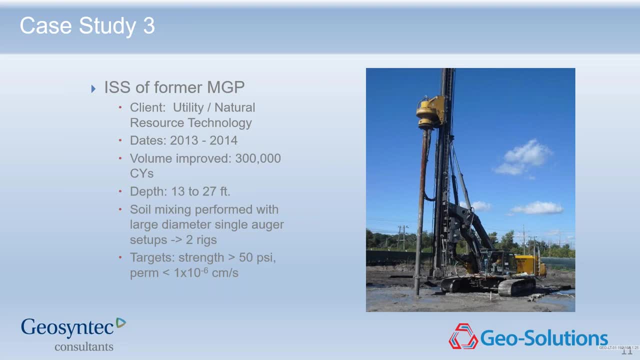 So the water, The water ratio, was very, very lean and the slag was used in lieu of the bentonite. And this is That's actually a fairly typical mix for most manufactured gas plant sites. that we perform: Anywhere from 50 to 75% slag and then 50 to 25% Portland cement. 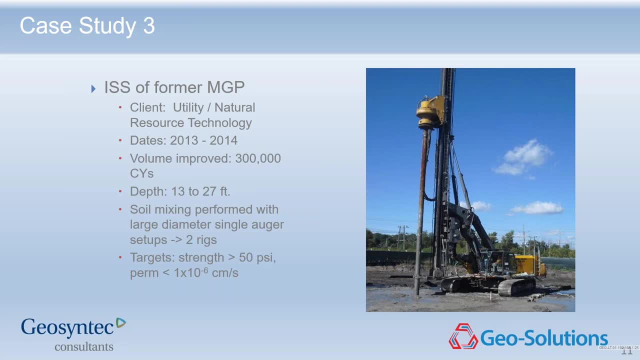 At times, bentonite is included in that mix as well, depending on your soil types. So there were some questions about that. Okay, So, yeah, so we're going to talk about that. It is fairly widely used now and we find it does have its benefits, especially since 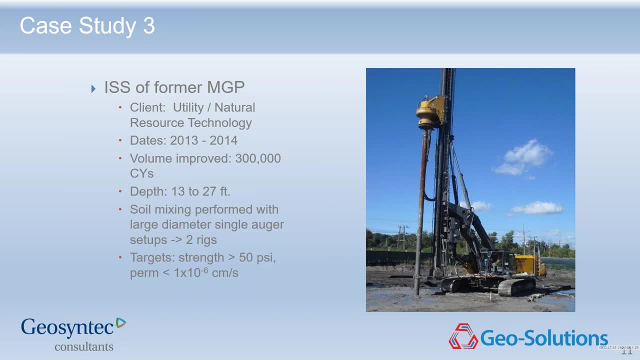 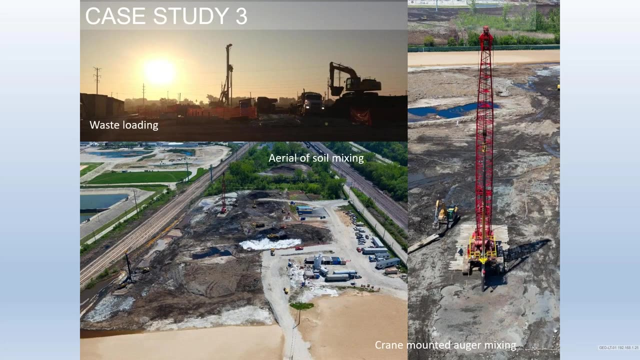 some other reagents are considerably more expensive but may also reduce permeability, but not as effectively. So some photos of the site. To the far right is a crane-mounted solidification rig. This is the site. This is the site. This is the site. 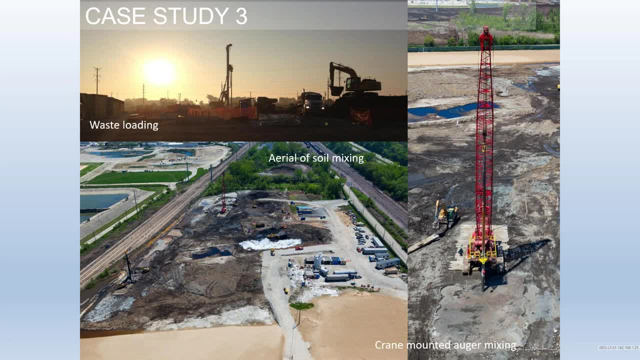 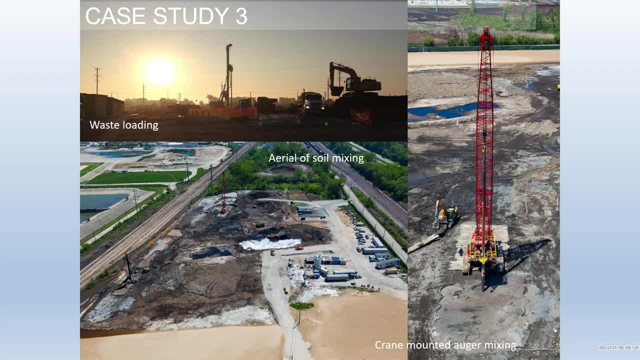 This one was completed over a full winter period in the Chicagoland area, so it was clearly cold, Happened to be one of the colder winters I think they've had in a while. We were able to only miss a couple of days due to sub-zero temperatures and wind chills that were considerably 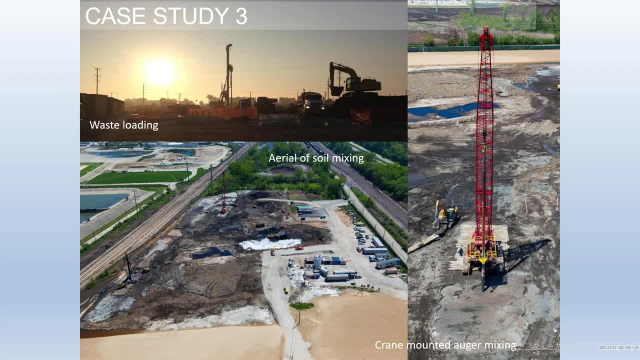 below zero by winterizing the plants and all the equipment every day and maintaining it. So in the middle of the page is an aerial of the soil mixing area and the site itself. Towards the bottom right of that photo is the batch plant, which is a fairly large setup. 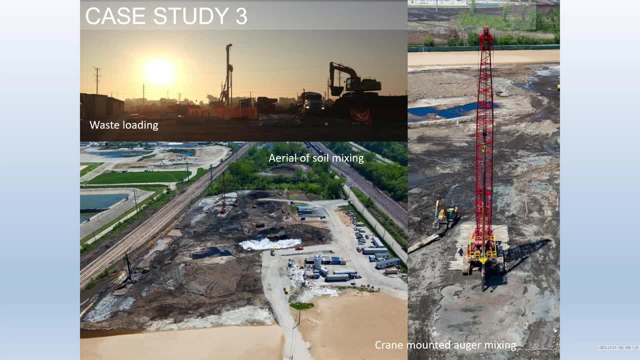 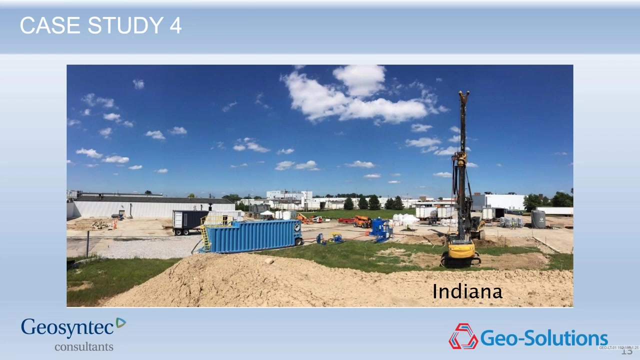 for any site. The site in total was about 12 acres and nine and a half of those acres were being worked on, and at the top left is the waste being load out, with the other hydraulic drill rig in the background. So the next project is another one, actually in Indiana. 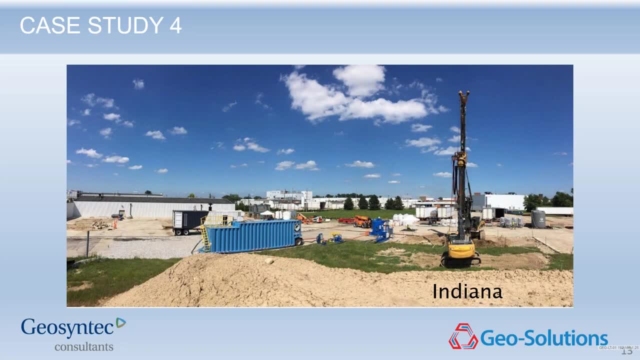 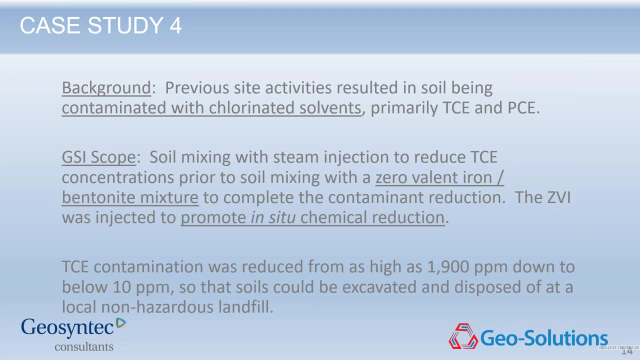 It was a steam-enhanced or steam-injection project. Okay, So Dan kind of alluded to this technology. It includes the addition of steam from an onsite boiler, as well as a considerable volume of compressed air that are injected through the ports in the auger. that would typically 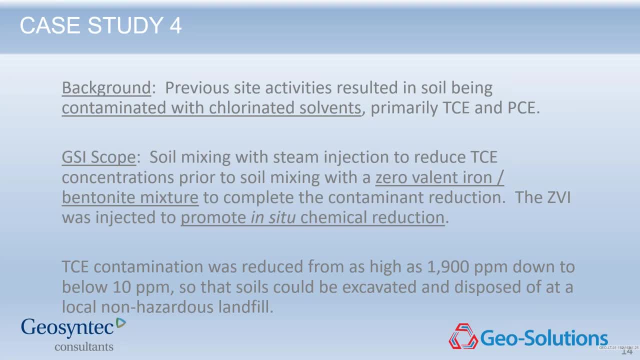 be used for a wet slurry or wet reagent. So the same equipment is basically used, but instead of delivering a slurry, we're delivering steam and hot air, So those two components are added to the subsurface. The steam comes from about 325 degrees to maybe 375 degrees, depending on how hot the 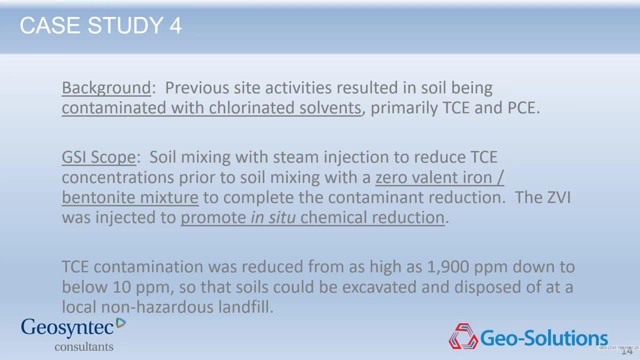 boiler is at the time and the air is 500 to 750 CFM. As the auger penetrates into the ground, it's adding the – it's heating as well as airing, aerating those soils and allowing the contaminants to volatilize, come to the surface and be. 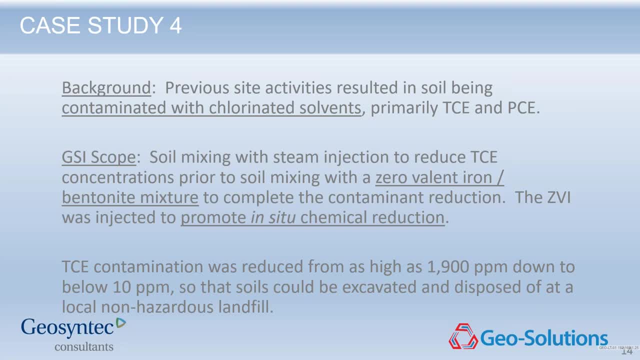 captured under the shroud. From that shroud they're sent to the treatment plant, which is typically a carbon bed. It may have a water knockout and some other telemetry that goes along with that. On this site it was used for chlorinated solvents, primarily TCEPC. 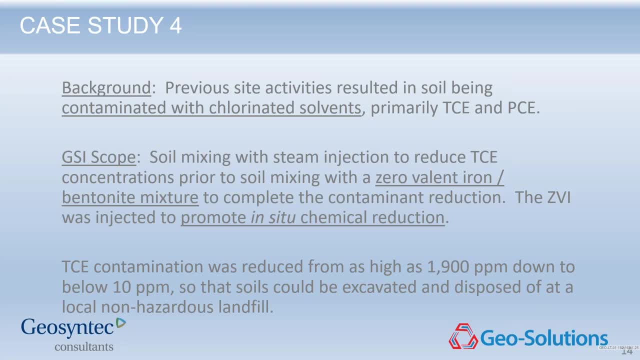 Those have a favorable boiling point for – for the water Okay, That's a good point for this technology. and tend to volatilize fairly easily. Additionally, there is often a polishing step where zero-valent iron is added, either with 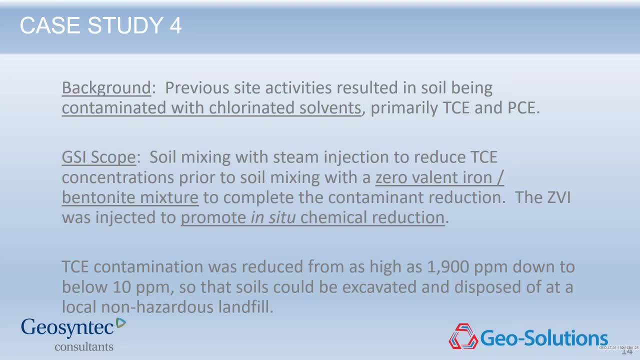 a bentonite slurry or a biodegradable slurry to continue to polish the – what might be left behind On this site. the TCE was reduced from 1,900 ppm down to 10 ppm And the owner had elected to actually remove the soils after treatment and dispose of them. 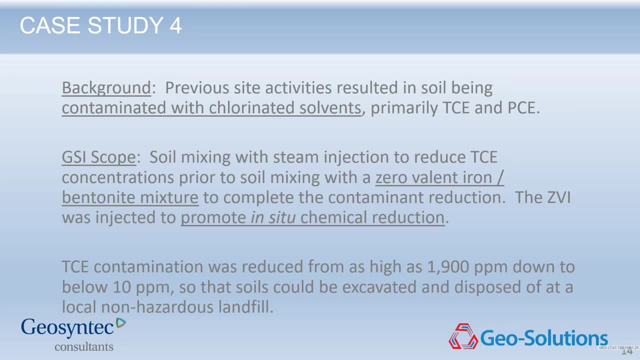 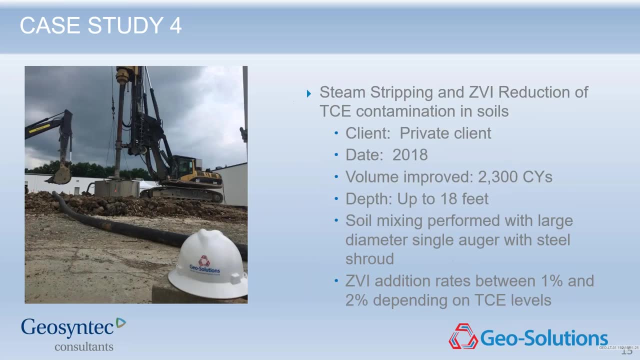 offsite with the goal of not having to provide any further monitoring and really kind of a belt and suspenders approach. The volume tree was about 2,300 cubic yards. It was set up with a track-mounted hydraulic drill rig with the shroud incorporated. 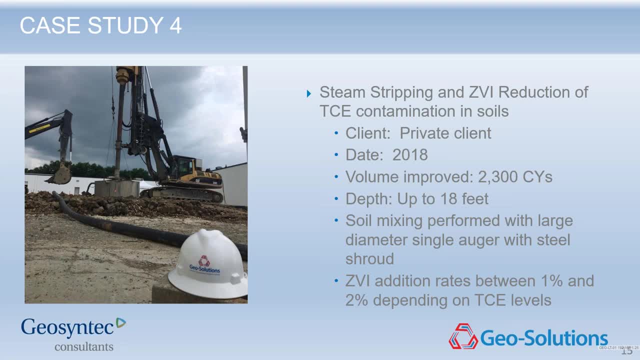 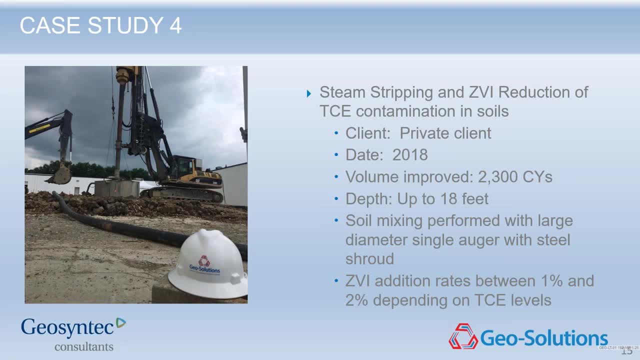 It was to depths of 18 feet and that shroud is – it's a steel shroud. Others could be used, but primarily because of the temperatures involved, steel is the best option. And the ZVI added with the bentonite was – it varied between 1 percent and 2 percent. 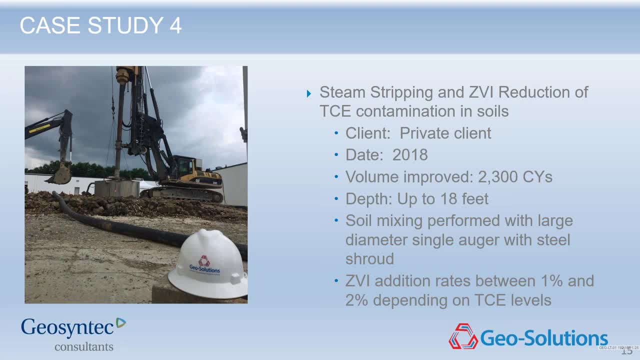 Oftentimes you vary your addition of the ZVI, Okay, the ZBI, in your hotter zones and you can see where those hotter zones are based on what's coming through that you can visually see on a FID and or GC within the treatment. 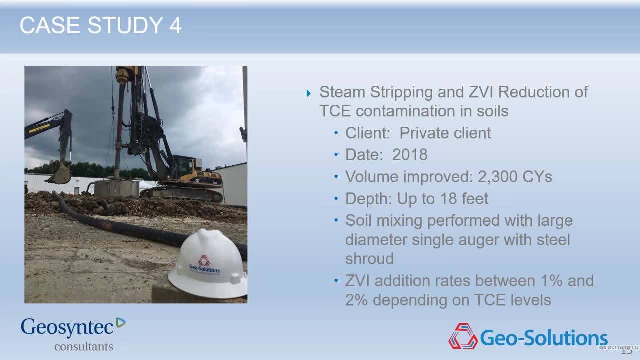 trailer where you can sit and watch the concentrations versus depth and as they go up and down. This can be a good technology if you're, if you have a desire to get 100% clean up. Basically, you can even step out and see what some of the concentrations are just outside. 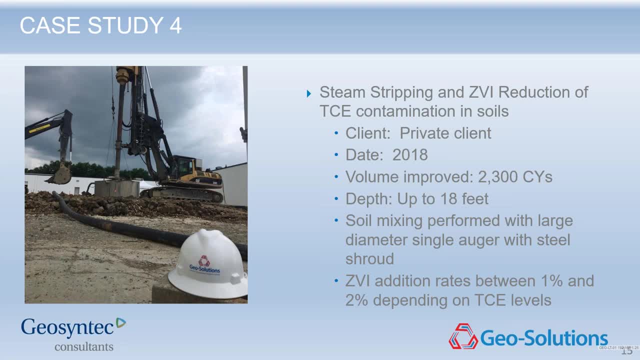 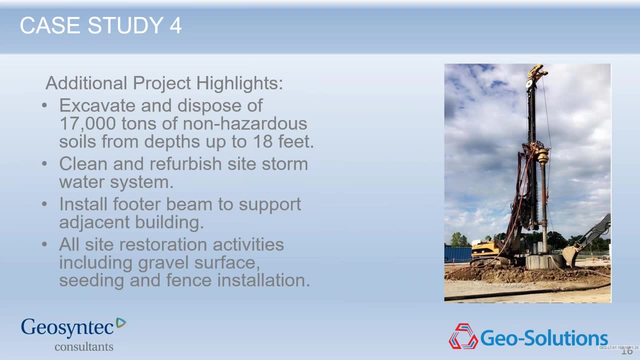 the limits to see if you need to add a couple more columns and things of that nature. So, as I noted, about 17,000 yards of disposal accompanied the treatment And all the site restoration activities were performed after this, Oftentimes the soil. if a bi-polymer is used, it's especially in granular materials. essentially, 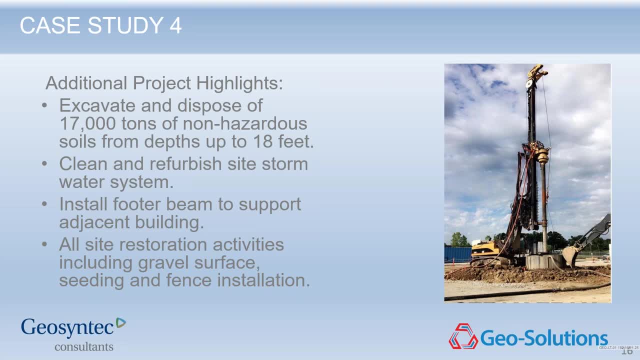 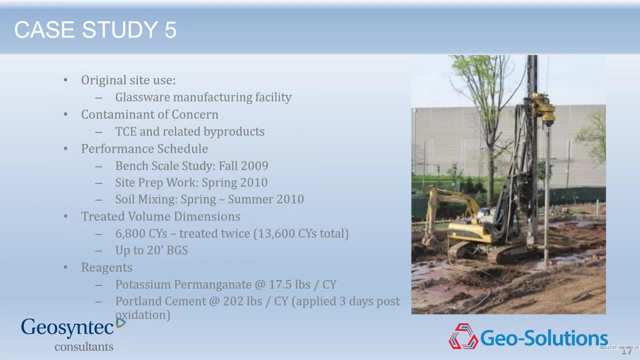 biodegrades and the soils are workable and able to be developed after that point. So the next case study is in East Rutherford, New Jersey. This project was a former glassware manufacturing facility. again, TCE and related byproducts were the contaminants of concern. 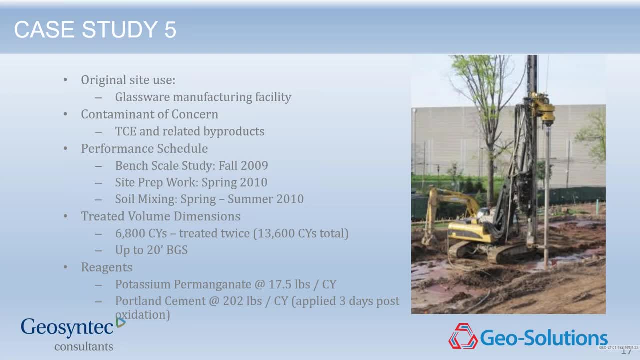 And it was performed back in 2010.. Approximately 6,800 cubic yards actually treated twice, up to about 20 feet. So the potassium permanganate, which is very identifiable in the next slide With its extreme purple color, was added in the initial pass. then Portland cement was. 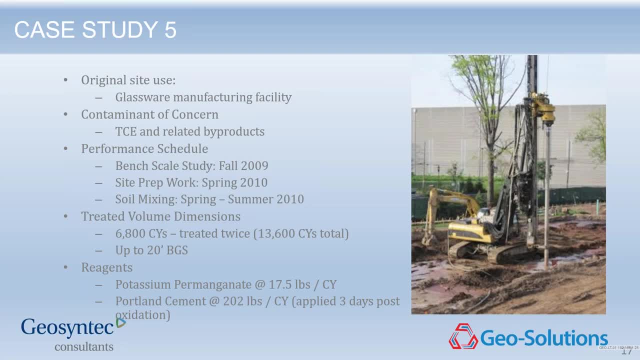 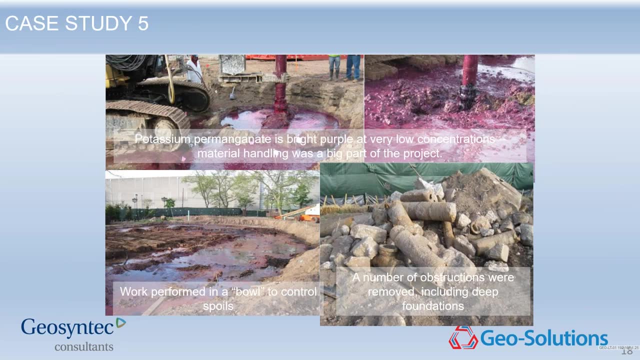 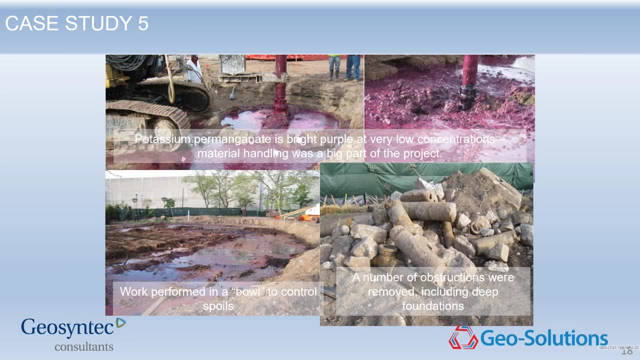 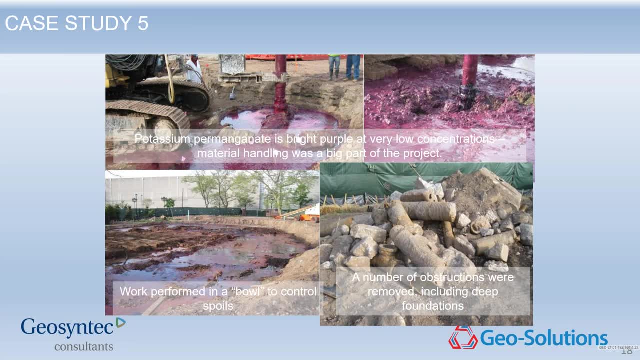 trenches or checkerboard to try to get those instructions out before the mixing starts, which is always the better case. And on the bottom left you can see kind of the berm that was used to control the spoils in the area. Again, all these sites include an overlapping pattern, as Chris. 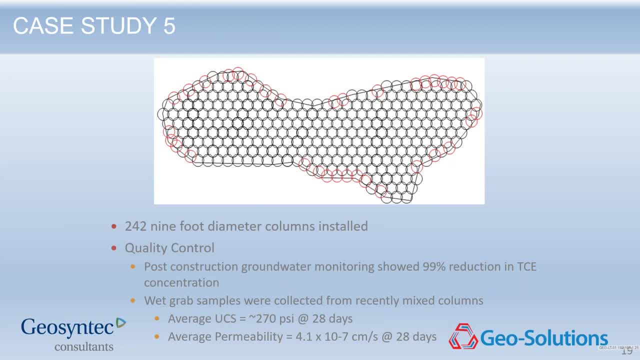 Again, all these sites include an overlapping pattern, as Chris Dan both showed. to achieve full coverage across the site, This project had 242 columns and the average uncompressed strength was about 270 PSI. That wasn't the requirement. These are kind of the average that was achieved. 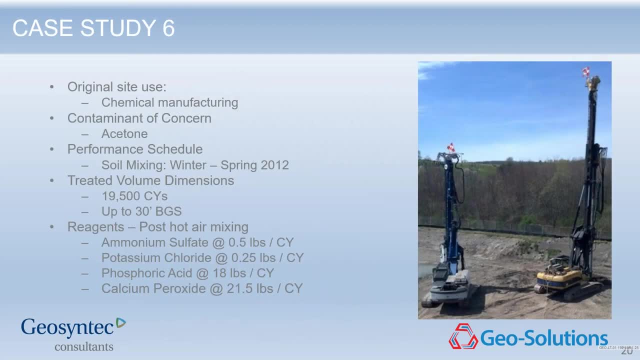 Okay, and our last case study is from Norwich, New York, at a former chemical manufacturing facility. The contaminant of concern here was acetone and about 19,500 cubic yards were treated up to 30 feet deep. This was a two-stage process where hot air was used to mix the soils and volatilize as 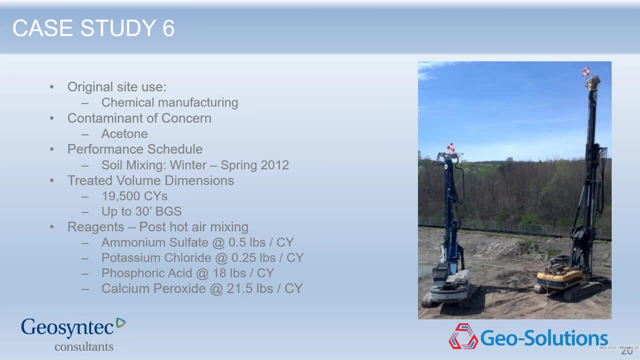 much as possible, and then a combination of reagents were used. after that You can see the two drill rigs. A number of reagents like ammonium sulfate, potassium chloride, phosphoric acid and calcium peroxide were all used in combination. 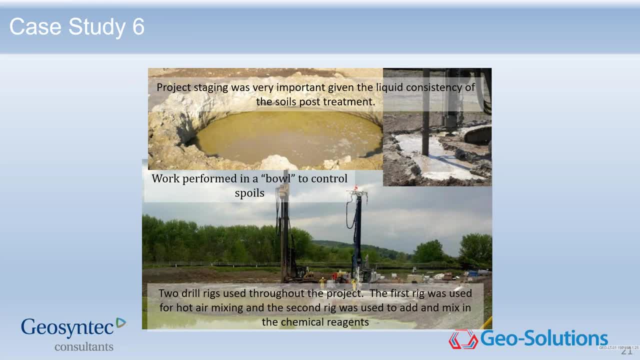 So project staging was important because there wasn't a sematicious portion to this project. so, like some of the others, it leaves some unstable ground for a period of time. And the two rigs worked side by side: 1. One using the hot air to mix and the other using adding the reagents after it had been. 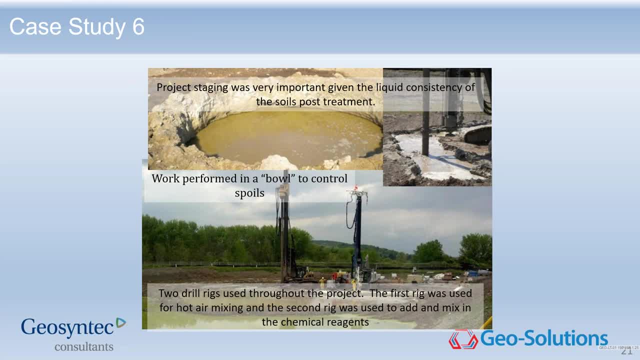 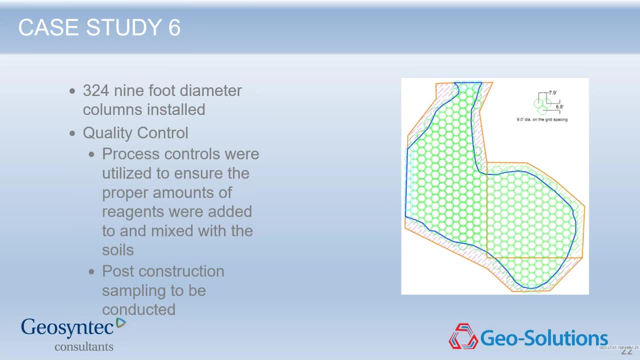 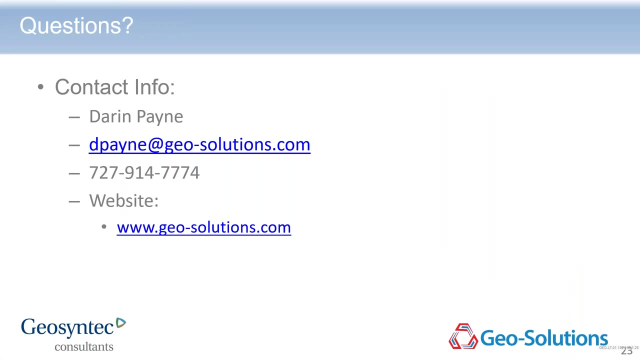 injected. I think I'm running low on time so I'm going to speed through and get to questions About 324 columns. As you can see, it's kind of the industry standard pattern And we have a few minutes for questions. 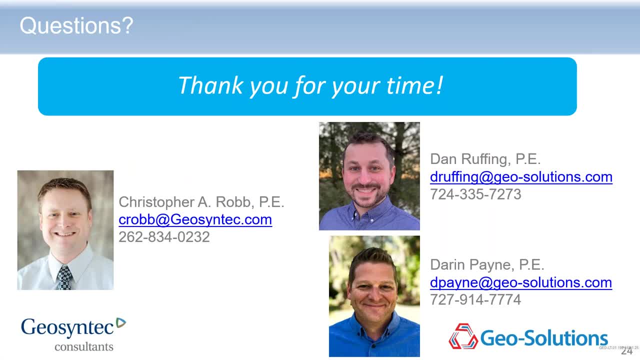 Great. Thank you so much. Oh, here's where everybody looks Great. So I think I want you guys to have time to address this one, because several people have asked about it is the cost. So can you give rough cost estimates for some of the different scenarios in terms of the? 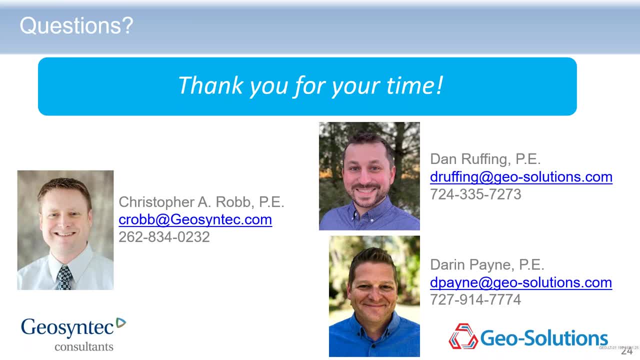 treatment, or when you find, or when people, what situations people hire you mostly for because I'm assuming the cost is higher than some other methods. Well, I mean it often wins out in feasibility studies where you're looking at excavation. with shoring and dewatering or other sites where the contaminants are more expensive to dispose of because of landfill costs or thermal desorption costs or things like that. The cost can vary based on constraints at the site. Based on the cost. Yeah, Based on soil types, largely based on the reagents that you want to use. So an oxidant-cement combination would obviously be more expensive than a straight cementitious solidification project. But I would probably encourage folks to reach out for budgetary numbers based on the site. 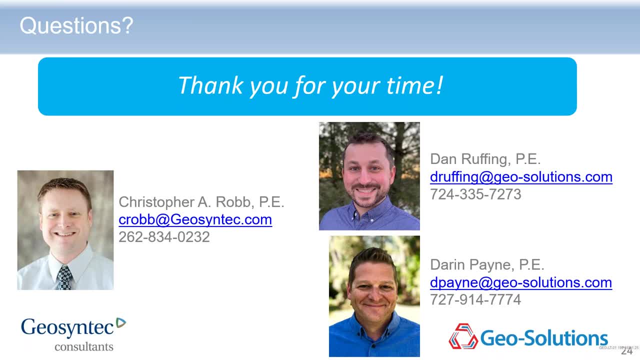 and what the goals are, because I hate to give a huge range, because I don't think that's truly helpful to anyone, But I think that would be probably the better way to go about it. Okay, I think to clarify case study five, where there was two rounds of treatment. they were: different treatments. right, There wasn't a problem with the first treatment that necessitated the second. It was the first one was treatment and the second one was solidification. So case study five: Yeah, Is that allowed that permanganate to react prior to the add of cement? 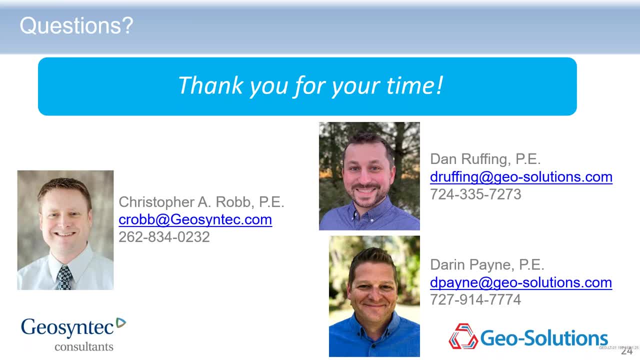 Now, it's not like it completely stops reacting when the cement's added, but it gave it a little bit of time for resonance. And, Dan, I don't know if you want to add any more to that, but It wasn't a second treatment of the contamination. 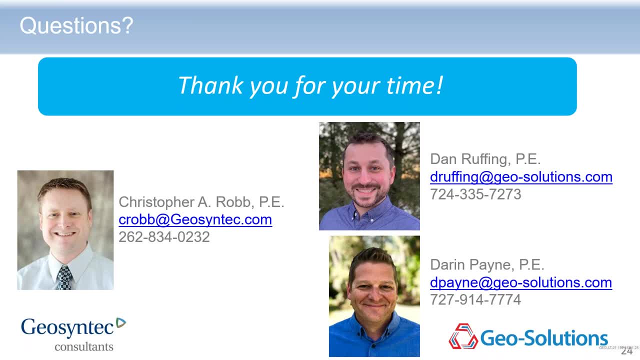 That's correct, Jennifer. The permanganate was the oxidation reagent, and permanganate does not behave well in the presence of cement, So we had to allow it to react for 24 to 48 hours before the cement could be added to. 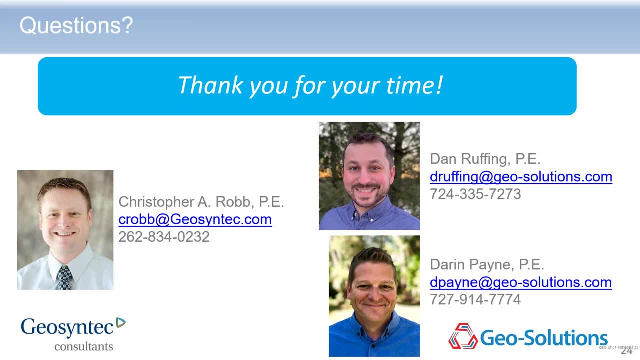 it And the cement was really added to it to facilitate future site development. not necessarily for the environmental remediation component, And I can chime in- We find that in that's a feature that they need more and more of, especially in these. high plastic clay sites, like over in Denmark, is they are looking for a solution because the initial chemical oxidation treatments is rendering the soils unusable for future redevelopment, So they're looking to put some cement in as well. Okay, Is there any direct contact concerns with some of this in-situ stabilization or other? treatments, Direct contact not so much. I mean generally. if you just put a simple depending on what the state of the land is, I would say no, Okay, Thank you. Thank you If the state requires a simple soil barrier over the ISS, that's enough. I mean it's going to turn into a solidified monolithic material. It's not really friable, So from that aspect, not so much. The one thing that we are looking more and more at and should be considered- and I did- 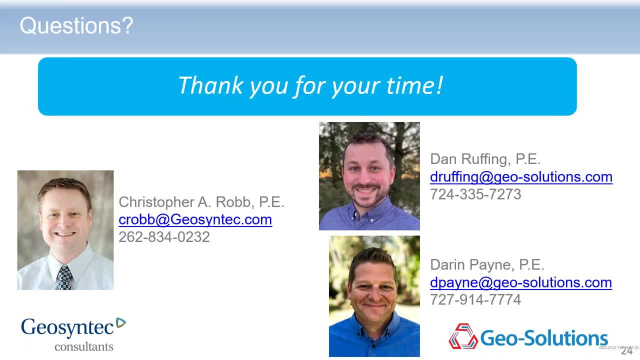 not put it in any of my slides- is vapor intrusion And, in particular, if you are going to build a structure on top of this material, you should be aware that it can. there can be- Okay, It can be, there can be odors that will come off of it over time if it's not properly addressed. 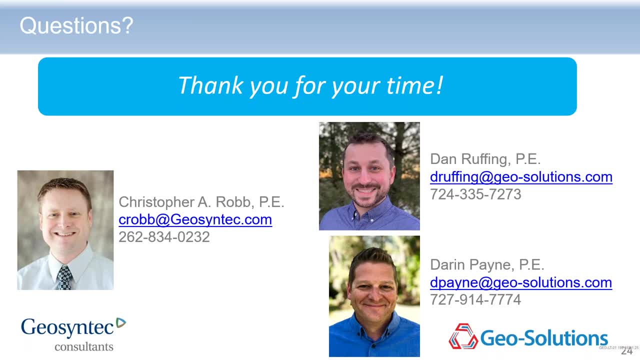 in the design, So some sort of subgrade ventilation system or just a passive layer, So, but that's something to just have some awareness around. Is it harmful vapors or just smelly vapors? No, generally it's not harmful vapors. 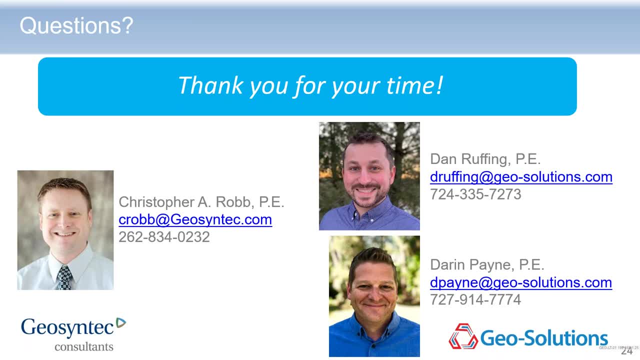 It's generally just an odor, but it still can be a nuisance and you should have your your designers and engineers evaluate that. if you want to put a structure on top of it Just like you would on any other brownfield site, Okay. 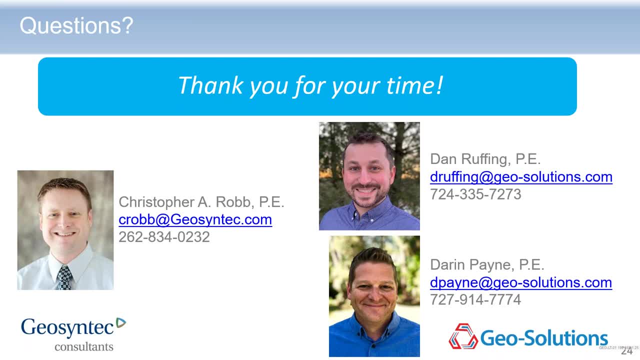 All right, There's a couple of questions that I don't think we're going to have time for because it's three o'clock now. If everybody can stay on for a little bit, I can ask these last couple, but I think some people are dropping off. 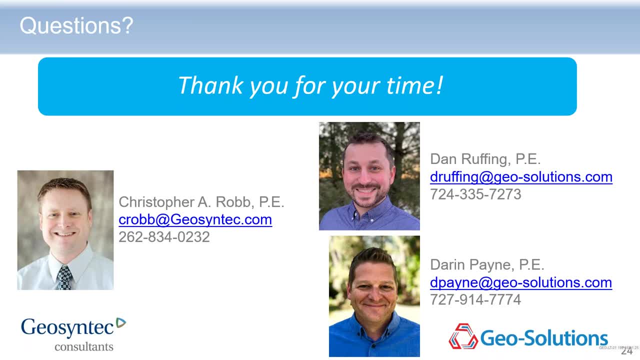 So I just want to be mindful of that. So if everybody can stay for a few minutes, we'll ask the last couple of questions, But otherwise I just want to thank everybody for joining us today and for and hope you have a good rest of your of your afternoon. 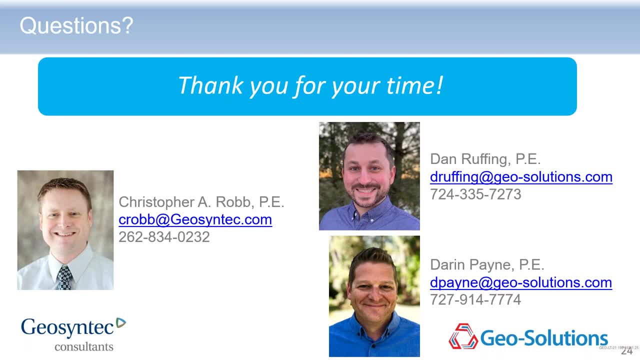 So getting back to the last couple of questions, So how about treatment? So like for that MGP site, case study three that Darren gave- is there documented improvements to the groundwater contamination And how? what kind of time period does that take place over? 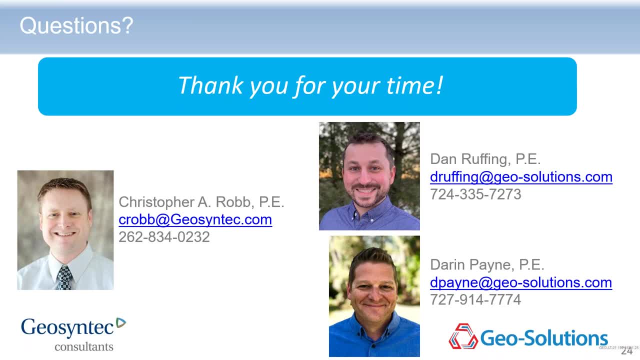 Chris, you might actually know more about the post data than I do. Which site was that? That was Waukegan, Oh, Waukegan. Yes, I actually don't know much about the data out there, but I know, but I know a lot about. 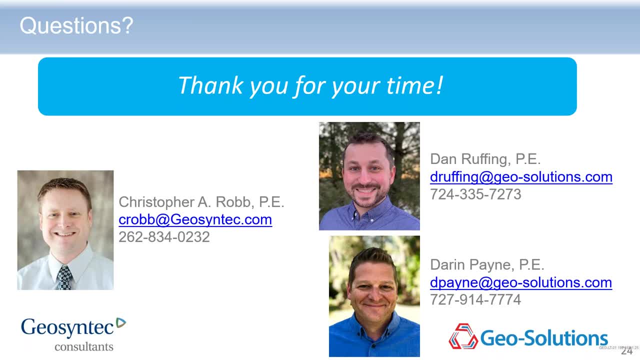 the data at the Solarod site- the case, the first case study- And they have found that they've seen a tenfold reduction in concentrations of benzene and naphthalene in the groundwater and that it's attenuating before it reaches the waterworks. 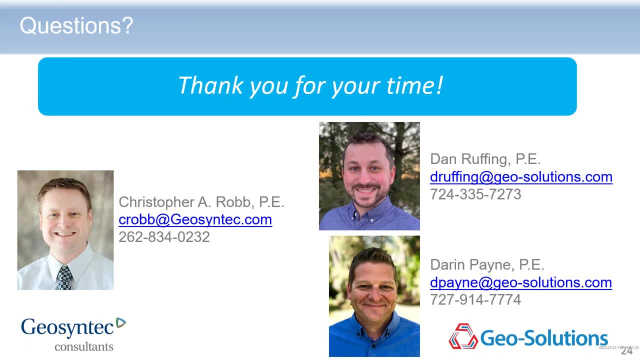 So in that regard, it was a success And that information just came out a couple of weeks ago- that remediation was completed in 2018.. That's so. that's roughly two years later. So That's the Denmark site. 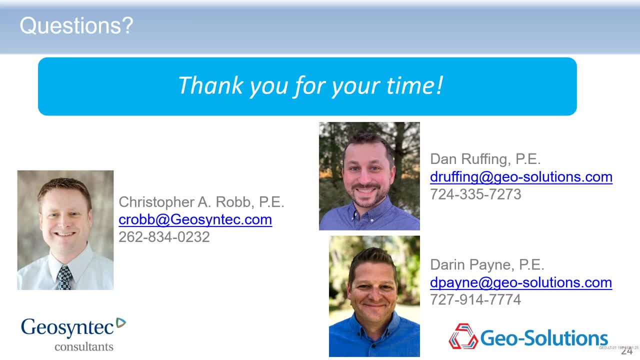 Yes, That's the Denmark site And that is an MGP site in the high plastic clays. Okay, And then the other question related to that site is about sulfate concentrations in the groundwater after treatment with sulfate, So noting that sometimes those injections exceed groundwater standards for sulfate. 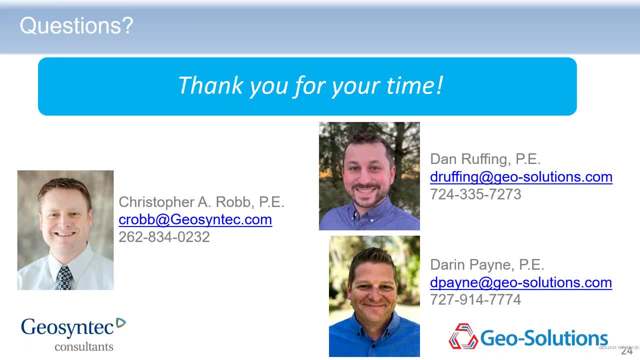 How was that addressed? or was that an issue in Denmark? In Denmark it wasn't an issue. Okay, It wasn't an issue because what we found is that the sulfate that was liberated through the persulfate oxidation reactions actually was used in the cement, in the cement chemistry. 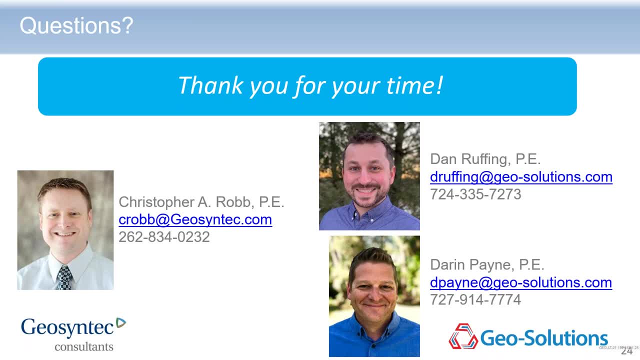 And we we did a little bit of research on it and we found that it was incorporated into compounds such as ettringite, That's a, that's a cementitious mineral, So it actually had was beneficial in that regard, But nothing that was so exacerbated. 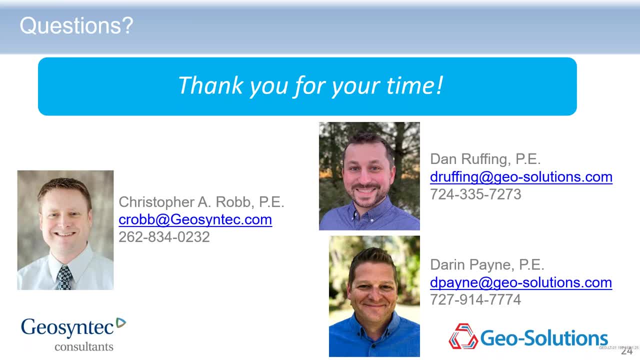 Okay, So that's a concern And obviously in Denmark, being directly adjacent to their waterworks, it was a concern for the downstream groundwater extraction. So, Okay, So you can design design around that issue. it sounds like Yes. 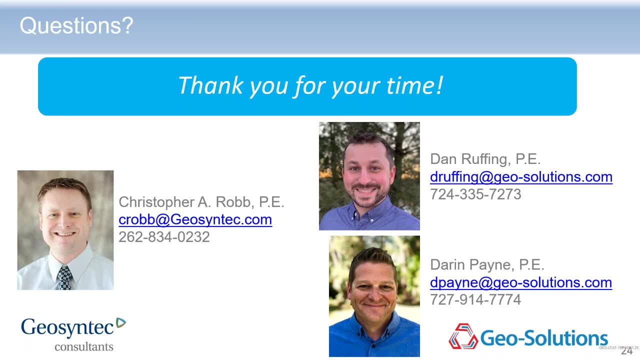 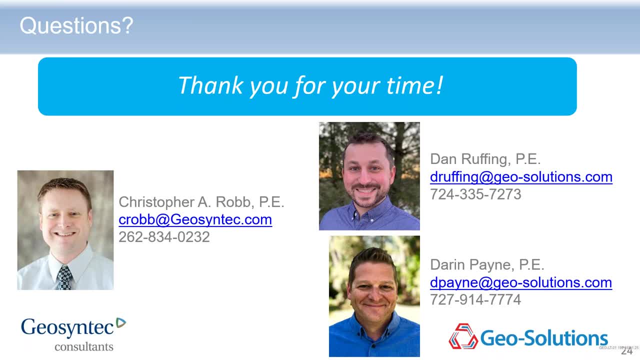 And again, I don't know if it's an issue if the, the, the, the, the, the design in the cement mixture in Denmark. So it has some. there's lots of reasons to use blast furnace lag or to consider using it And there's not a downside to using it in terms of introducing contamination? Generally no, I mean. blast furnace lag is a commercially available product. So if you go to most cement suppliers, like a Lafarge or any large cement supplier, they often will have blast furnace slag. It's a product that's. 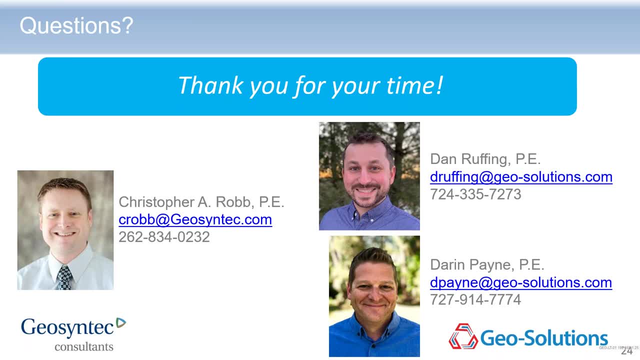 utilized worldwide as a cement enhancement or replacement, called slag cement, And there's an actual ASTM standard for it, C-989.. And in general, no, it's not a concern In some states. I know here in Wisconsin we actually had to do a beneficial use. 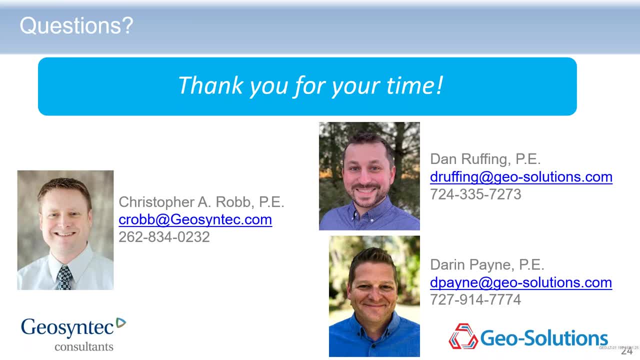 byproducts certification, where we just sent in some very general chemistry about the slag to get authorization from the state to use it in place of cement for this application. But that was a one-time certification And once it was on their books it's been applicable to all future ISS. 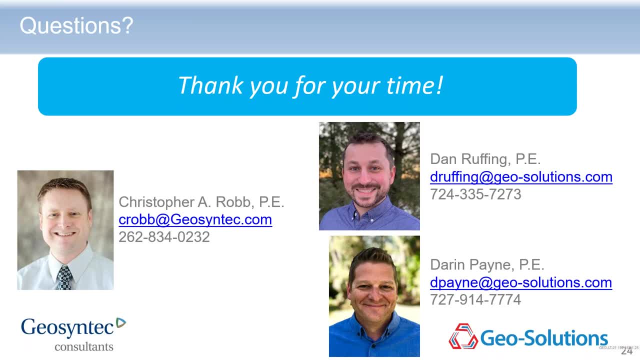 projects done In this state. So generally, no, it's not an issue. Okay, great, I think there's one more question And that would be. I think that's it. Yeah, So, going back to the thought about landfills and being able to treat landfills, what's the size? 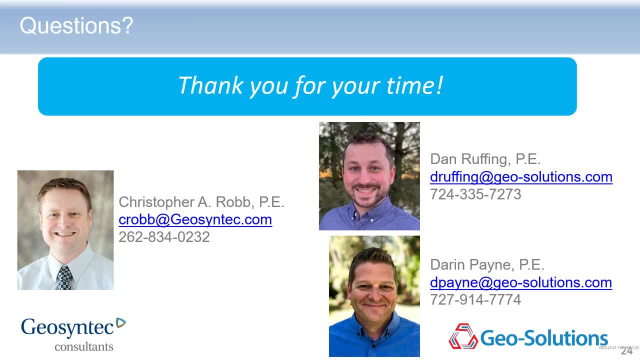 obstruction that you can deal with or not deal with. If there was a washing machine in there, would that create a Yeah big problem? or how is stuff like that handled, Aaron or Dan? I figured you want to jump on that one. Yeah, I mean anything that can'tthat a steel auger can't pass through is going to be an issue to some degree. If it's within the top 15, maybe as deep as 20 feet- the support excavator can reach in and maybe remove it. But the washing machine example that. 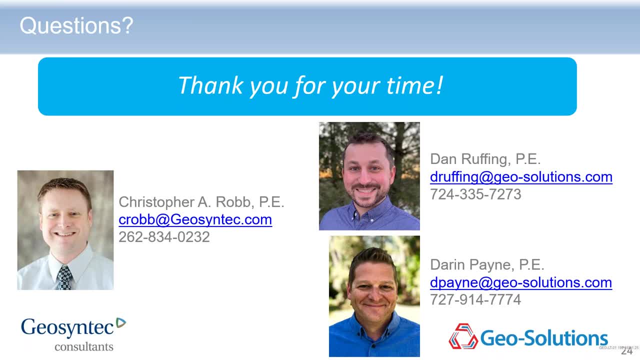 is probably not going to be something you're going to be able to pull up through the column, And you really don't want to sit there and try to pull up large obstructions when the column's in its fluid condition, because you end up creating a 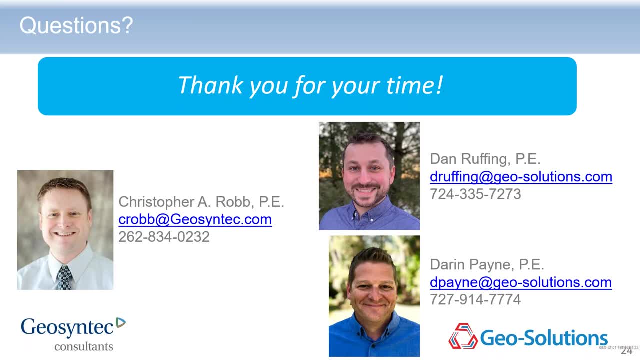 quagmire on site, just destroying the sidewalls of the column and collapsing the entire soil mixed area. So a lot of times if there's larger obstructions, like the East Rutherford case study that Darren talked about, at that site we encountered. old pile foundation system. So we went through and once we determined that there were foundation issues in the site, we did geophysics over the whole site, identified which columns were obstructed. we treated all the columns around those known obstructions and then we excavated. the obstructions out before we went back in and did the soil mixing. So if it's isolated things like that, then you can do some pre-excavation, specifically if it's, let's say, less than 20 feet. but if you have deep, large obstructions, they're going to be very challenging. You might have to kick into a more expensive technology like jet grouting to extend your columns down below and around those sort of obstructions. Okay, So generally, how big can rocks be, or whatever that don't create a big problem for you. That's a real loaded question, Jennifer. I mean we've pulled boulder-sized materials out on. 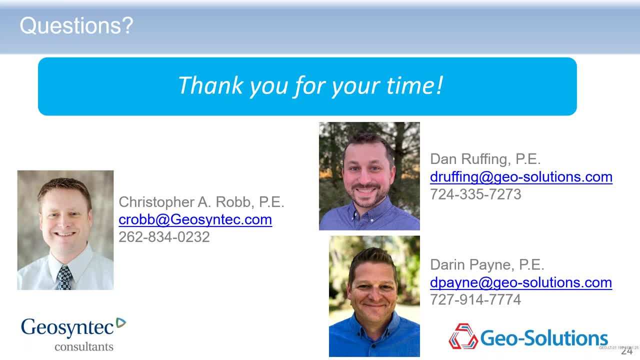 the order of multiple feet across in both dimensions, but it really just depends on how lucky you get and where the obstruction is located within the column and at what depth. And again, you don't want to spend too much time, so if it doesn't come out immediately, 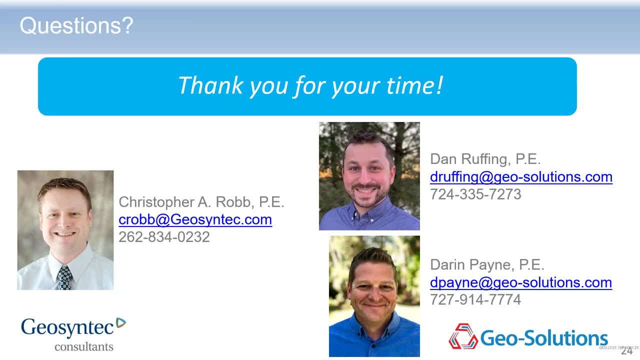 a lot of times you give up and deal with it after the fact. Right, But how many inches can a stone be before it creates a problem? How small can they be before they create a problem? It kind of depends also if they're like inter-dispersed or kind of a bunch of things nested together like larger cobble layers or 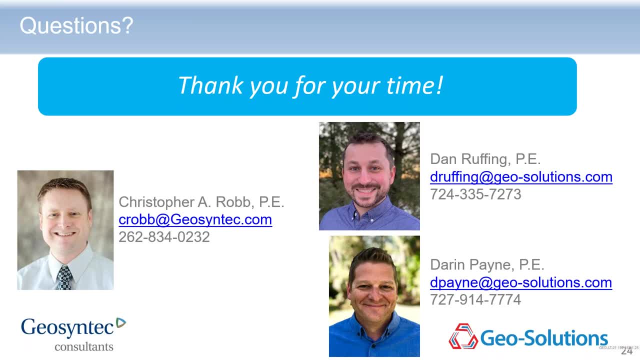 bricks that were put all in one area might be a problem, But I mean, I like to say a couple of bricks here and there, inter-dispersed, not all nested together, things like that or smaller than a basketball. If there's one or two of those in the column, sometimes we can work around it. 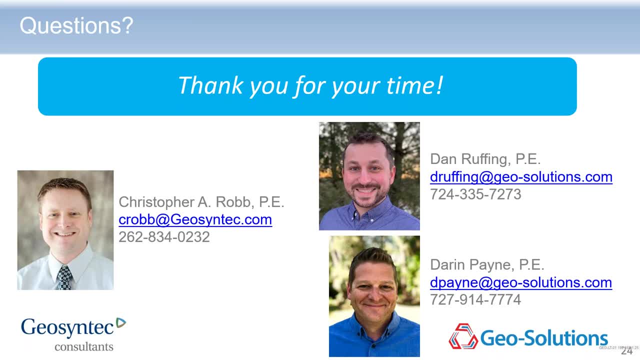 but it's certainly not what the equipment's made for. but it wouldn't shut the job down. But nested cobbles boulders certainly an issue. Pipes are always a no-go because of the way that they are typically in the ground. 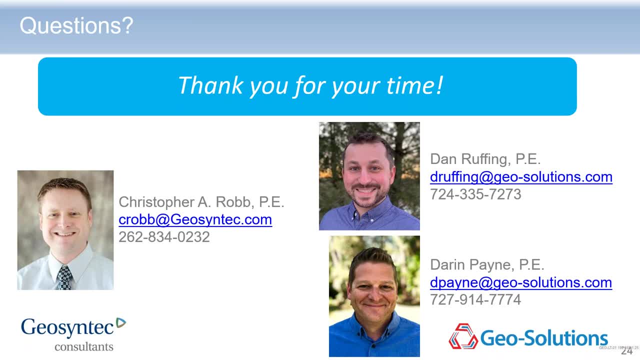 If it's a one-inch surface line. a lot of times we just tangle that up in the auger and peel it off. but ideally you'd have a good handle on where those things are as best you can, And if that includes pre-trenching, you have to do some of that. Yeah, Darren, you might want to also.